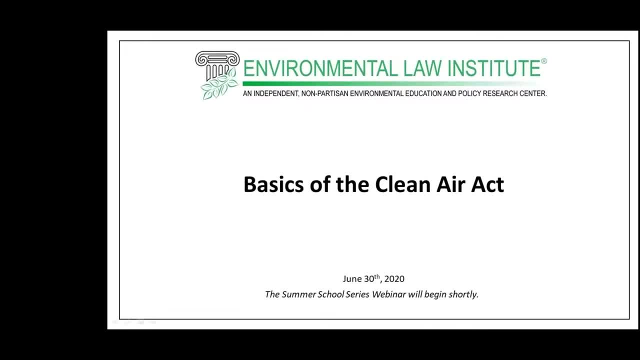 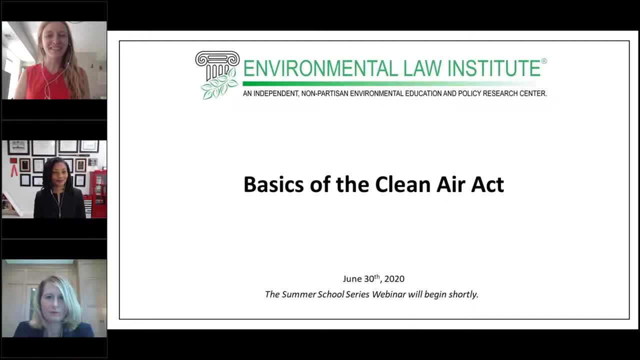 Good afternoon and welcome to the Environmental Law Institute. You have joined us for the basics of the Clean Air Act. My name is Caitlin McCarthy and I'm the Director of Education Associates and Corporate Partnerships here at ELI. We are delighted to welcome everyone. 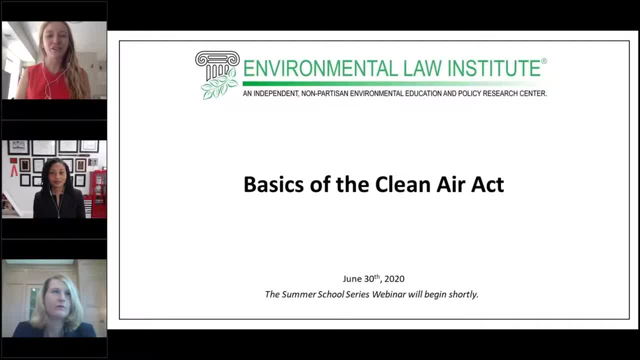 to ELI's annual summer school series and I encourage you to join us here at ELI every Tuesday for summer school. For more information, please see the events page of our website at ELIorg. I will note that summer school seminars are taking place by webinar only. 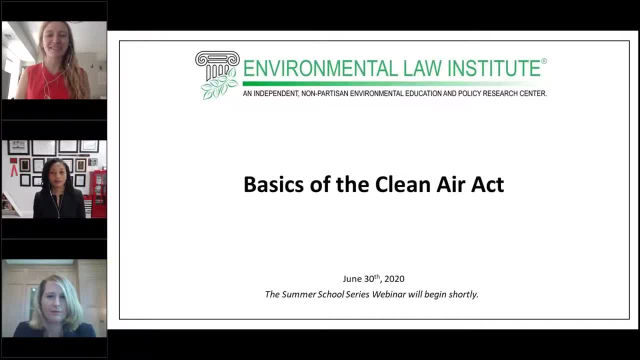 this summer to ensure the safety of our panelists, participants and staff. Thank you for your understanding and for joining us. At the end of today's panel, we will have time for a question and answer session. Please submit your questions using GoTo's question box and. 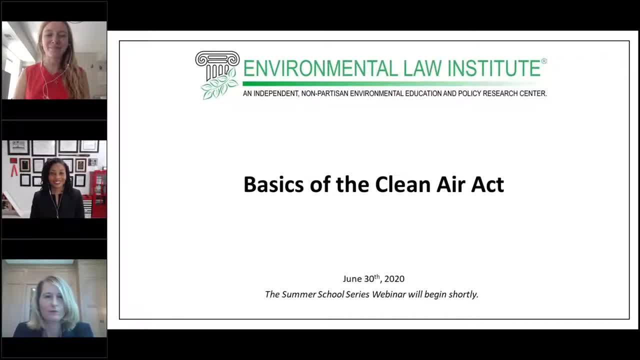 please do not wait until the end. Send your questions as soon as you think of them. I would also like to thank our outstanding panelists for joining us today to lend their leadership to summer school. While I will introduce them briefly, momentarily, the full speaker. 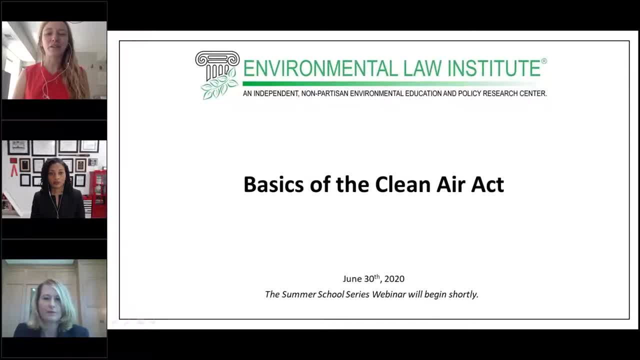 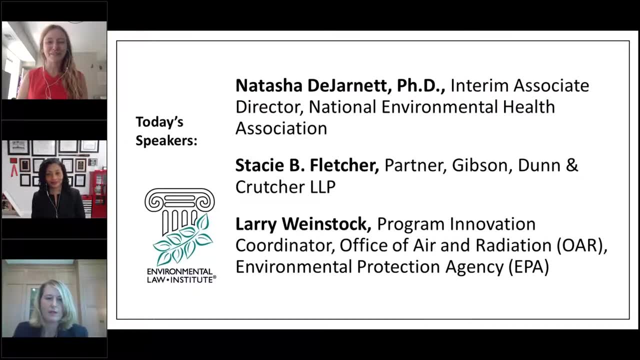 bios are posted on our website, ELIorg, and I would encourage you to check out their expertise in more detail there. As we begin, I would like to briefly introduce our panelists. Dr Natasha DeJarnette is the Interim Associate Director of the National 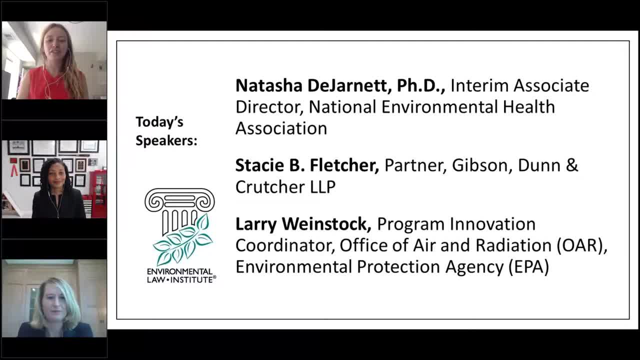 Environmental Health Association. Her extensive educational background is in science and public health And Natasha also has vast work experience in research development, environmental health and safety. She contributes an interdisciplinary approach to assessing environmental health challenges. Natasha is renowned for her drive to improve quality of life for people through influencing meaningful environmental health. 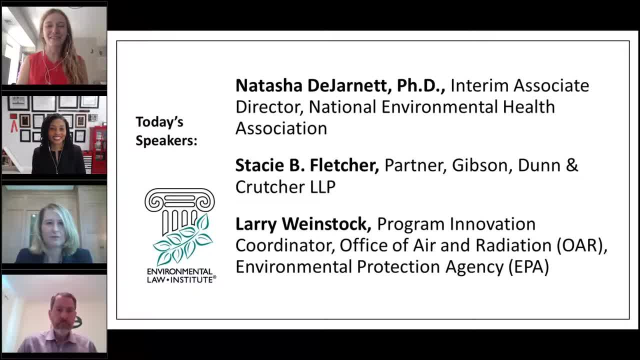 policies. Natasha, we appreciate you lending your expertise to summer school. Stacey Fletcher is a partner at Gibson Dunn and Crutcher. There she is a litigation partner and practices in the firm's litigation department And is the co-chair of the Environmental Litigation and Mass Tort Practice Group. Stacey has handled 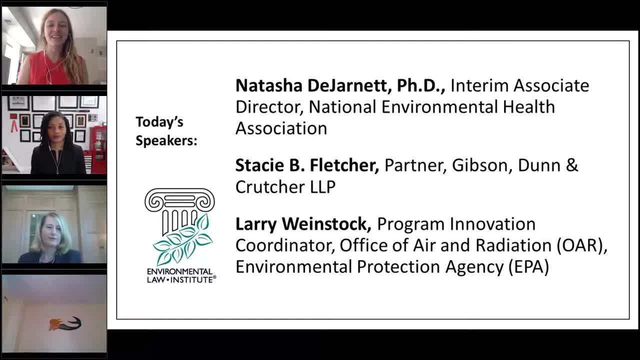 a wide variety of cases under federal and state environmental statutes, including serving as lead counsel on numerous enforcement defense matters with the EPA and state agencies. Stacey received her law degree from the University of Virginia, where she was the executive editor of the Virginia Law Review, and her Bachelor of Arts degree from Davidson College. Stacey. 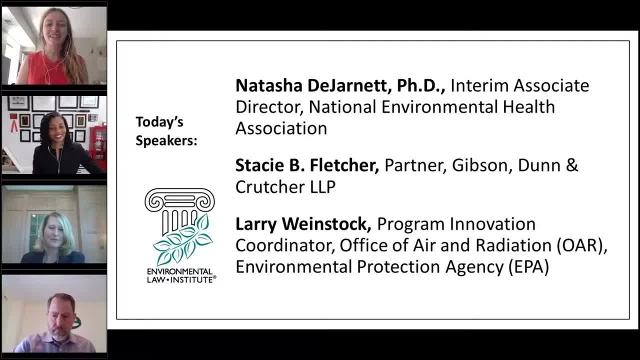 thank you for joining us today, And Larry Weinstock. Larry Weinstock is the program innovation coordinator for the Office of Air and Radiation at the Environmental Protection Agency. He is a highly skilled program manager and regulatory professional with extensive experience in a range of federal program leadership roles. 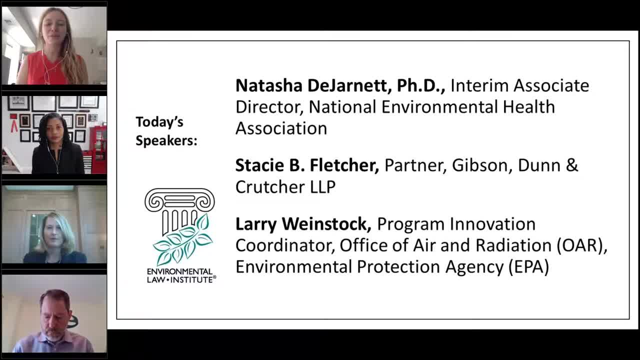 Larry has established two EPA programs, in addition to serving as a program innovation coordinator in the EPA's Office of Air and Radiation. He has been recognized for his talents in facilitating collaboration among various departments, offices and multiple stakeholders. Larry, we are delighted to have you here with us today, And with that I will turn. 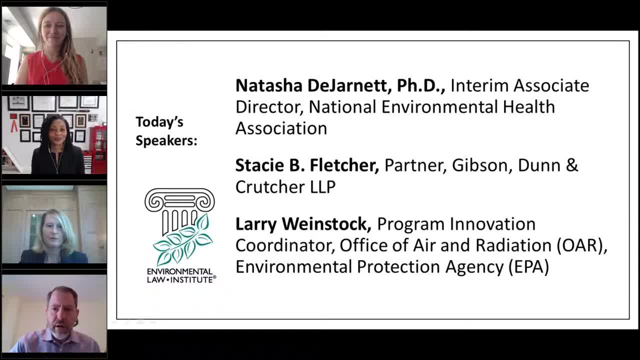 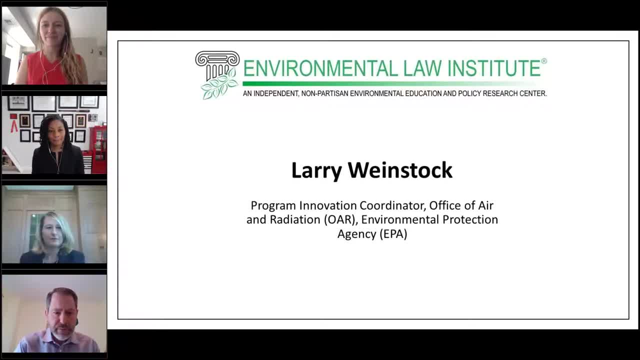 things over to you to get us started. Hi there, I'm really pleased to be here today And I'm happy to give you guys an overview of the Clean Air Act. So if we could just get started on the slide. Okay, next slide. 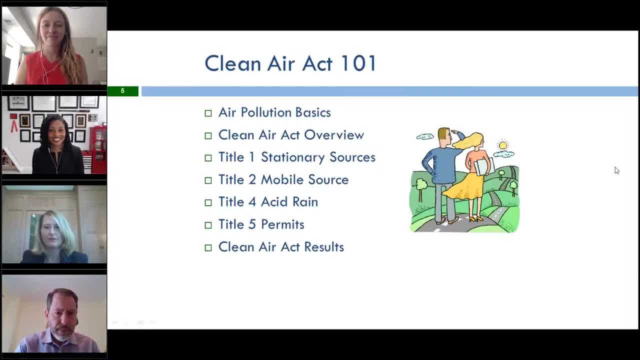 Okay, what we're going to talk about today. I'm going to cover some air pollution basics, a Clean Air Act overview. Larry, we're excited to be sitting here today And I'm also touched by you guys entering the program today. 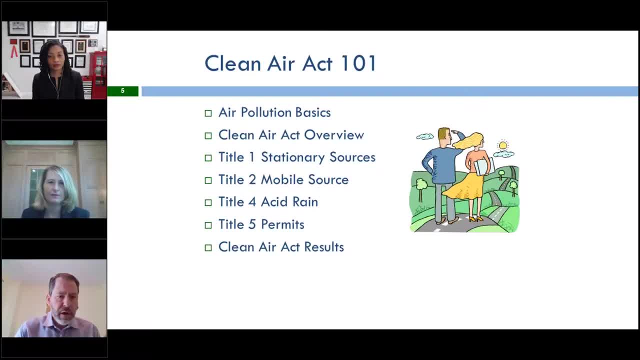 And you don't have to wait to greet us. I'll be happy to help answer our questions so far. If there's other questions, feel free to put it below. review and then talk about four of the major titles of the Clean Air Act, and then a little. 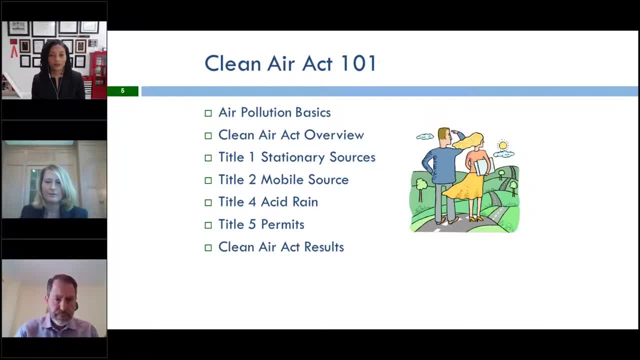 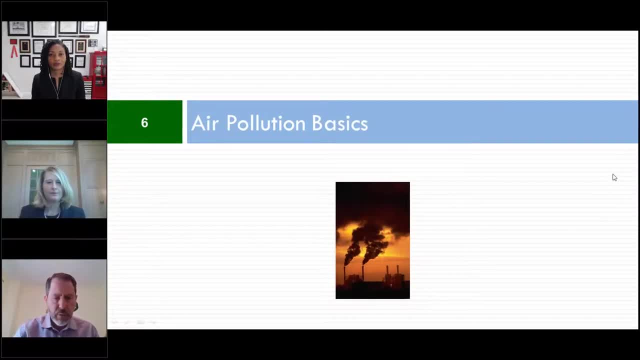 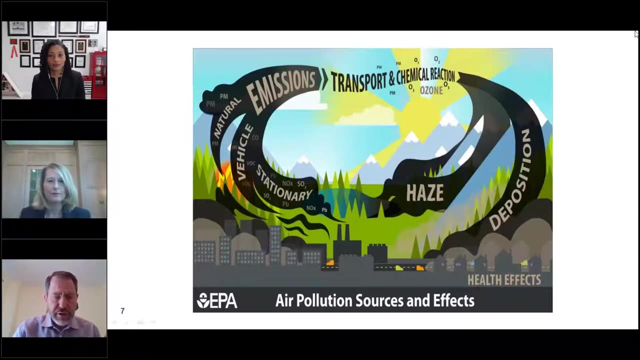 bit about the results of the Clean Air Act. Next slide: Okay, And one more Okay. So to really understand how the law works, it's helpful to understand how air pollution works, So I'm going to spend a couple of minutes on this slide, just so you have an understanding. 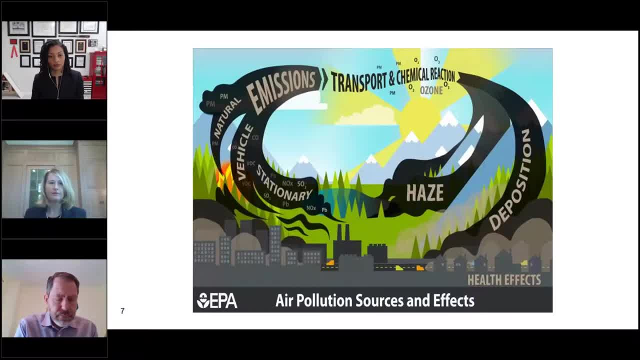 of air pollution science and why the act is the way that it is. So, on the left, you see a city and you see that there are all kinds of emissions coming off that city. Some are from stationary sources. You have SO2, sulfur dioxide. 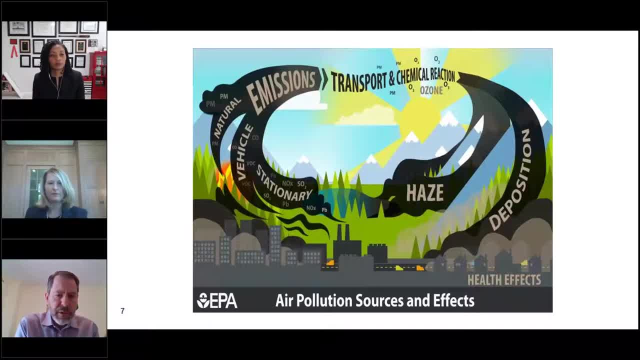 You have NOx, which are the oxides of nitrogen. You have PV, which is lead, And VSD is volatile organic chemicals compounds. Those compounds are things like benzene or, if you think of gasoline, if you spill gasoline. 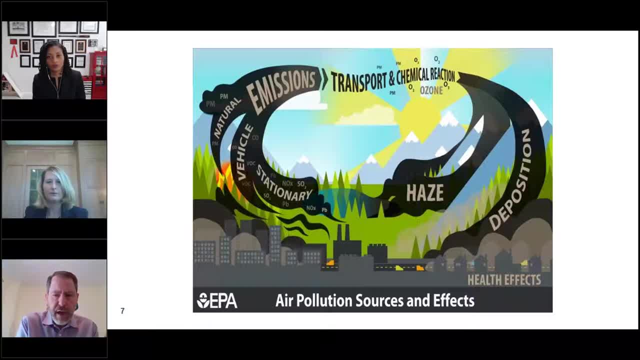 you know that it all evaporates. Lots of organic compounds have that same property, and so when they evaporate, they wind up in the air. Sometimes they're also produced directly from things like vehicles or stationary sources as well, So you have all of these pollutants going off. 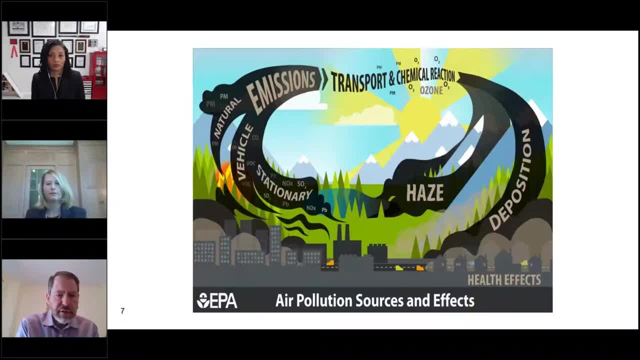 You also have some natural pollutants. See, there's a fire on the left-hand side. The California fires were famous. It was all over the news all the pollution, mostly particulates, that were coming off of those fires, although trees in their natural state can often release VOCs as well. 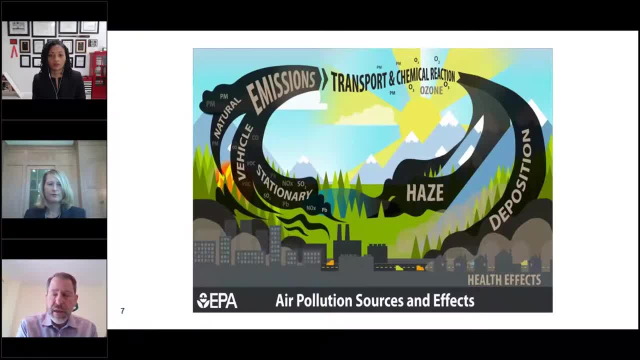 So you have all these emissions going up into the atmosphere and they can be transported. Sometimes, if you're in a city, that transport is the same city as the sources. the transport is immediate, You're just. you know, you're right next to them. 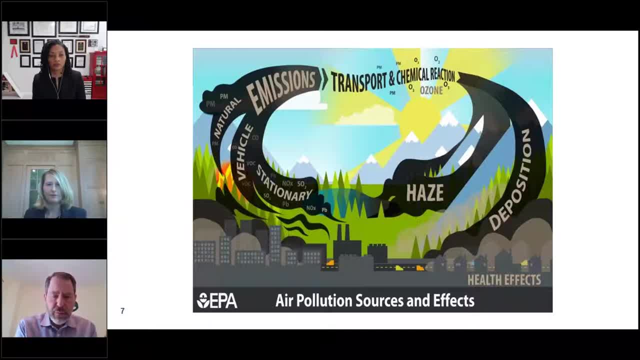 But these emissions can also go high into the sky and be transported for tens or even hundreds or thousands of miles. EPA monitors in California can actually detect pollution from China. So, as you see in this slide, we have a nice sunny day, and that's because the sunlight. 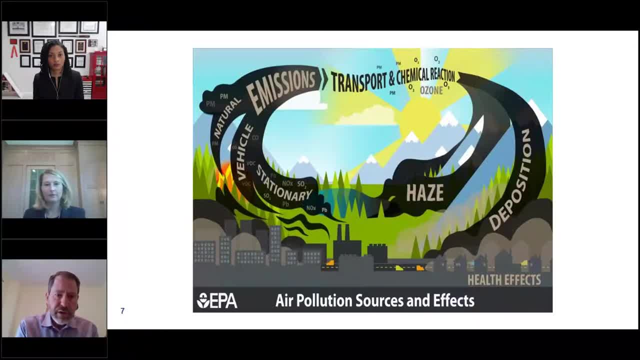 and the heat are going to drive chemical reactions, Especially between the VOCs and the CO2.. So you know you're going to have a lot of CO2.. You're going to have a lot of CO2.. So you know, if you have no CO2, you're going to have a lot of CO2.. 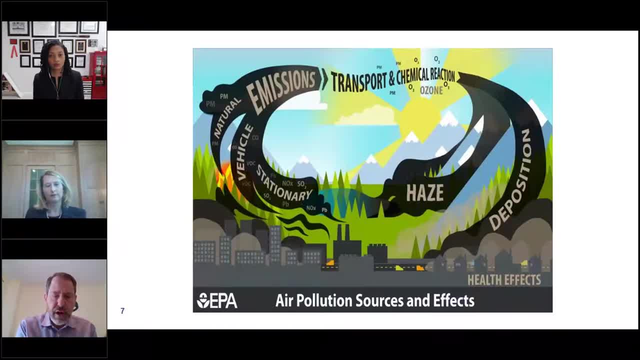 You're going to have a lot of CO2.. So, you know, because of the CO2 and the VOCs and the NOCs and also some of the sulfur dioxide, you're going to be creating new particles. The chemicals themselves are going to break down, they're going to interact with each 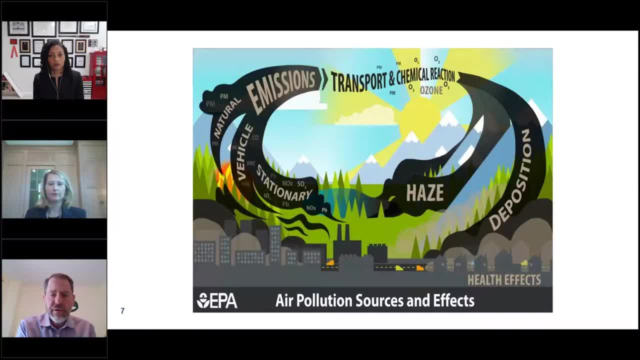 other. You're going to create more particulates and you're also going to create ozone. Ozone is a toxic chemical. It's very reactive, which is how it causes damage in the body and to plants as well. Okay, chemicals together are working. you know. they're in the atmosphere. they break up light from the sun. 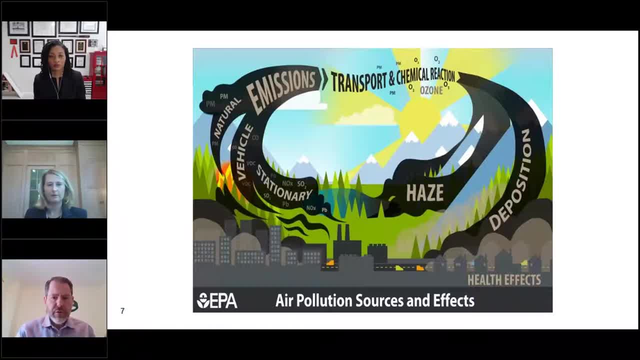 so, while the sun is driving their production, they're also diffusing the sunlight, so it can't be seen, and so, um, or well, it can be. i mean, it can be seen, but it's not as direct, um, and so you get haze on really polluted cities. if you look from a distance, you may even be able to see, like a black. 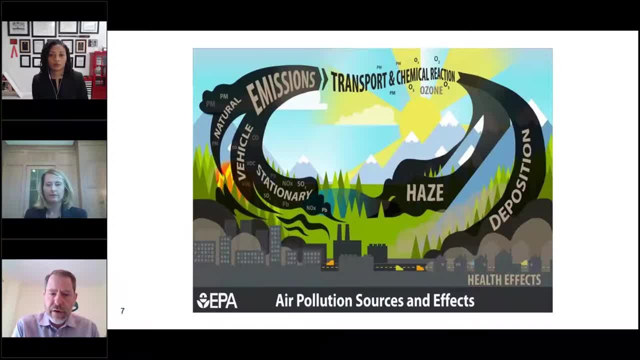 brown layer in the air, um because of the coronavirus and um reductions in economic activity. for the first time in literally decades, people in new delhi have been able to see the mountains around them, so the next thing that happens, um, or that can happen, is that these: 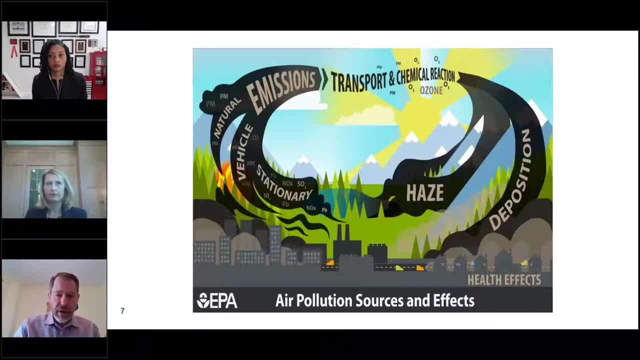 chemicals that are in the atmosphere can, can drop. you know what goes up, comes down, and that includes pollutants as well, and so by getting that deposition, which can either be wet, in the form of acid rain, or dry deposition, you bring those poisons back down um to the 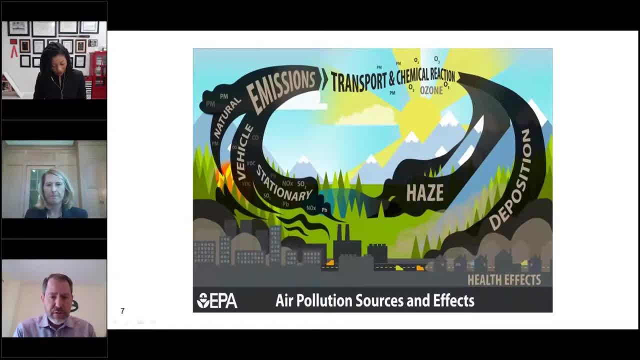 level where people are breathing them and that's where you get your health effects. so, um, for a city like washington, for example, the general air flow is from southwest to northeast, so actually the worst ozone in the washington dc area tends to be just north north east of the city. next slide: 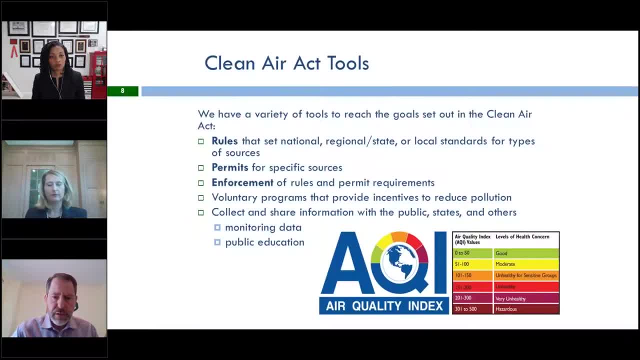 next slide, please thank you. so we have a variety of tools to reach the goals set out in the clean air act. we have rules and regulations that that standards for all types of sources. we have permits for larger sources. we can enforce these rules. we have voluntary programs that provide incentives to 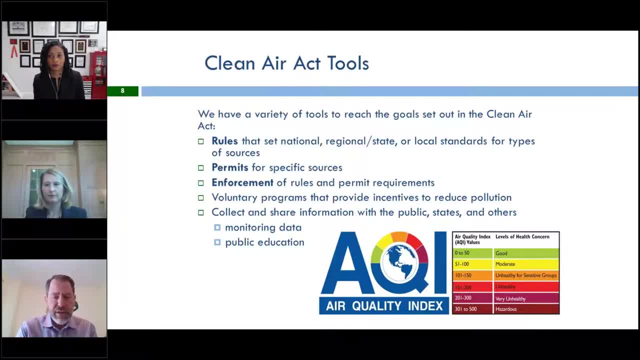 companies to reduce pollution or provide information to the public so that they can take action on their own. we also have monitoring data, and we have a lot of data that we can use to monitor the quality of the air in the area and public education, one example of which is the aqi the. 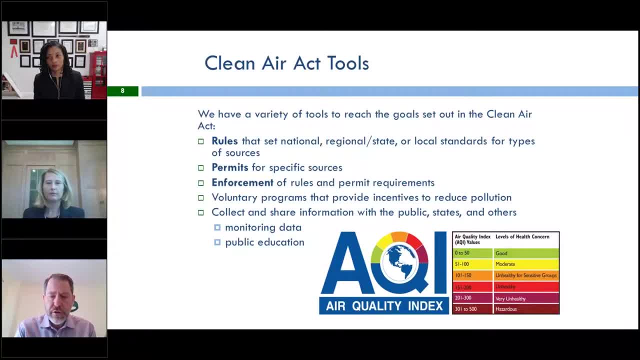 air quality index. this index is set so that a hundred. if you're at 100 or higher, you are violating one or more of the national ambient air quality standards. the next, which we'll talk about in just a couple of slides. but this air quality index is actually an app. you can get it on your 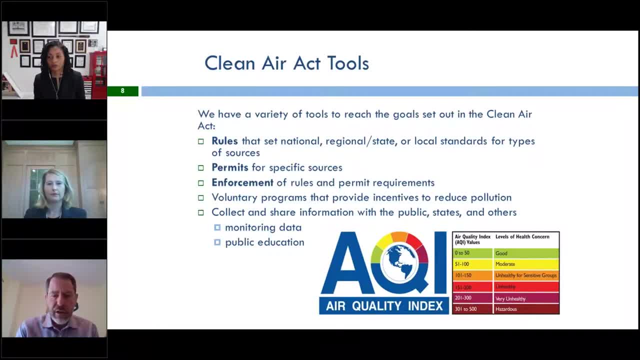 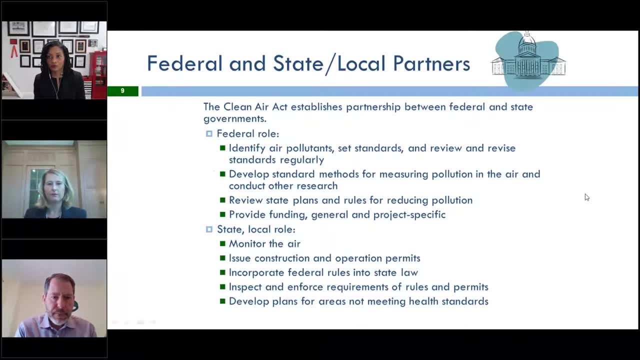 phone and it will tell you the air quality in your area on any given day and what the air quality will be in the next couple of days for your where you live next slide. so the cleaner act has set up a federal state local partnership, so there's a different, there are different roles for each of the actors. the federal role. 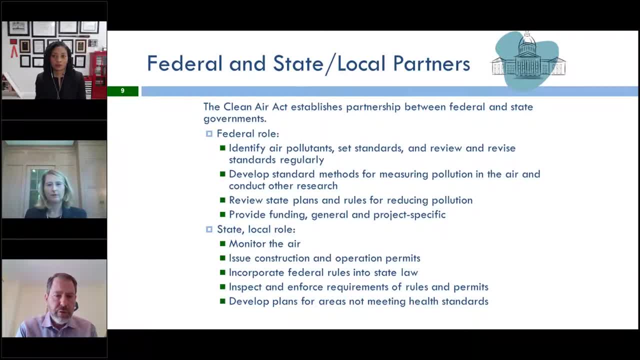 is. we identify the air pollutants. we set standards, review and revise those standards regularly. we develop standard methods for measuring pollutant pollution in the air. we conduct other research. we review state plans and rules for reducing pollution. state plans need to meet federal standards. state rules need to be at least as stringent as federal standards. 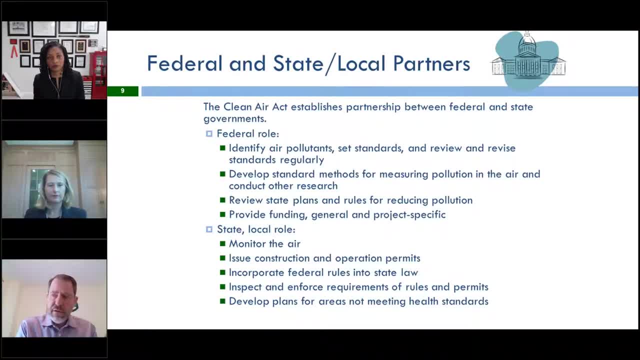 and we provide funding both general and project specific. so the epa air budget provides about is provides almost as much money to the state as we do for all epa work. we provide a lot of general support and then project specific report support. state local role is they do the monitoring. 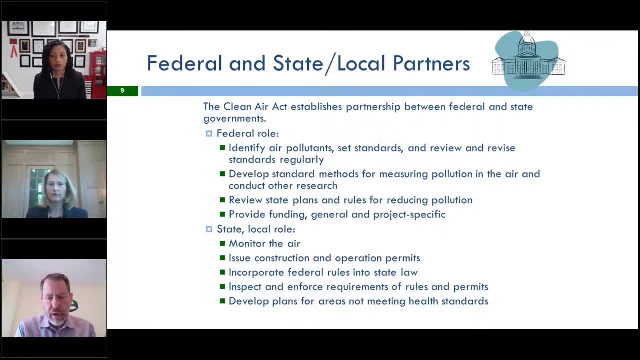 under epa guidance and under epa rules for locations and monitors and how the monitors are to be operated and the equipment in them, the issue, the construction and operation permits. they incorporate federal rules into state law. they do most of the inspection and enforcement is done at the state and local level and they develop plans for areas not meeting. 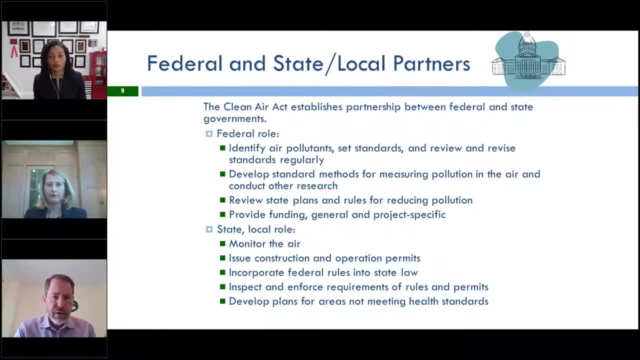 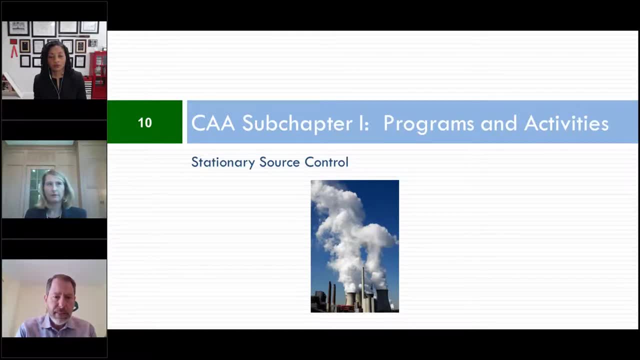 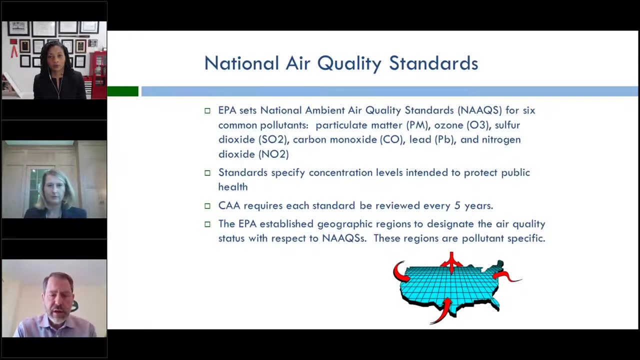 health standards, which we'll talk about also in a couple of slides. next one: so, uh, we're going to talk about stationary source control now. next slide. so the key, one of the key regulations around air quality it is, are the national air quality standards. epa sets national ambient air quality standards. these are the next. 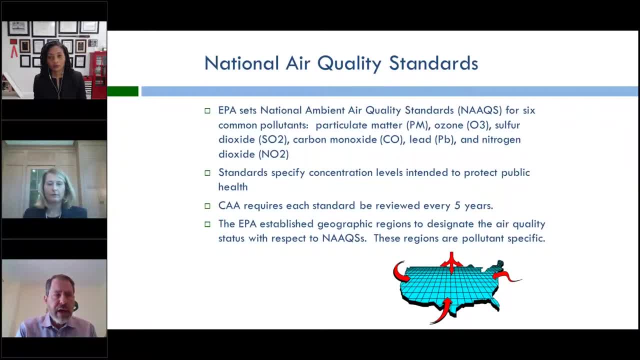 for six common pollutants and the idea here is that they're ambient air, so it's like the air generally in any area. so, for example, we're worried about all of chicago and what the air is like in chicago. so these are not standards about specific facilities and the people who live next to them. there are six common pollutants: particulate matter, ozone, sulfur dioxide, carbon monoxide, lead and nitrogen dioxide. the standards specify concentration levels intended to protect public health, and these standards are supposed to be revised every five years, although frankly, that's we're not good at getting them done that often, and we've established geographic regions to. 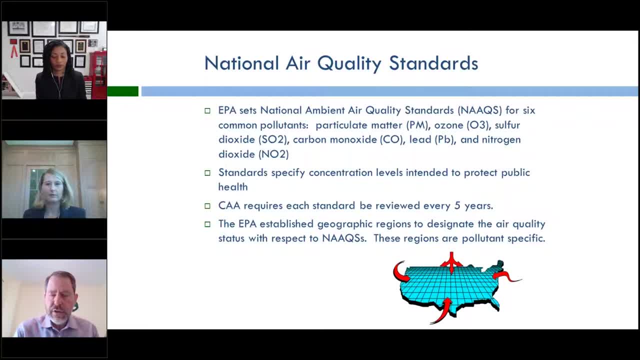 designate air quality status. with respect to the next, these regions are pollution pollutant specific, but for example for ozone. the state of new jersey is split in half, basically between the philadelphia airshed and the new york city airship. next slide state implementation plans for the sips. the state developed 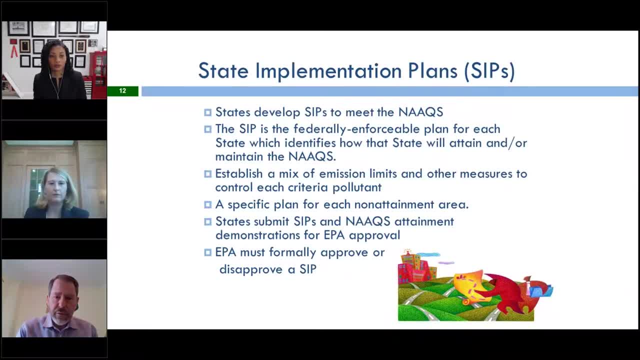 these plans so that they can meet the next. they are federally enforceable plans for each state. they identify how that state is going to attain or maintain the next. so just because you're meeting air quality standards doesn't mean that you don't need a sip anymore. they establish a mix. 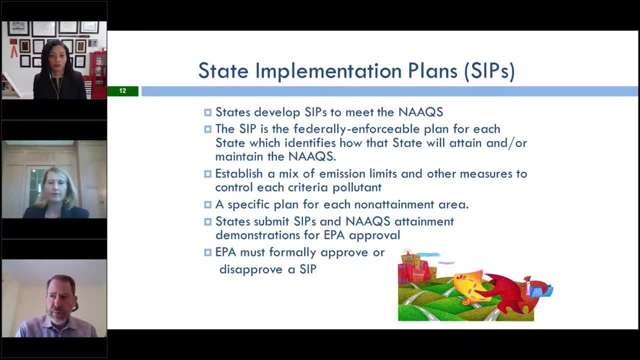 of emission limits and other measures that will control each criteria pollutant or the precursors for them. so ozone, as i showed before, isn't actually emitted by any facility it's really created so people would care about. for ozone you mostly care about either vocs or nitrogen. knocks and it depends on the local area which one is more important. for example, in los angeles, if you further reduce vocs, you may get some health benefits because a lot of them are poisonous, but you're not going to actually reduce ozone unless you reduce nox. a specific plan is for each non-attainment area, taking into account the sources. 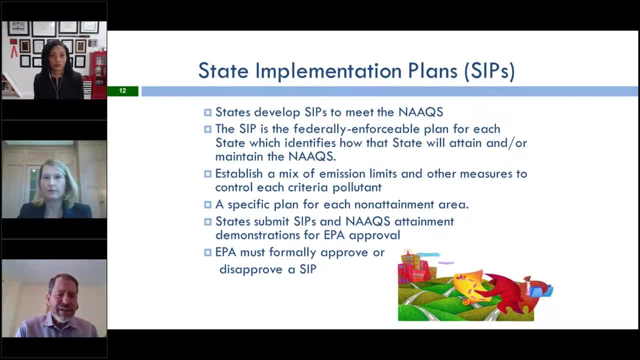 and the meteorology of the area. The states submit those steps and their attainment demonstration. So the state not only has to have a plan, they have to do modeling around that plan and that modeling has to show that they will either maintain the NACs or they will come into. 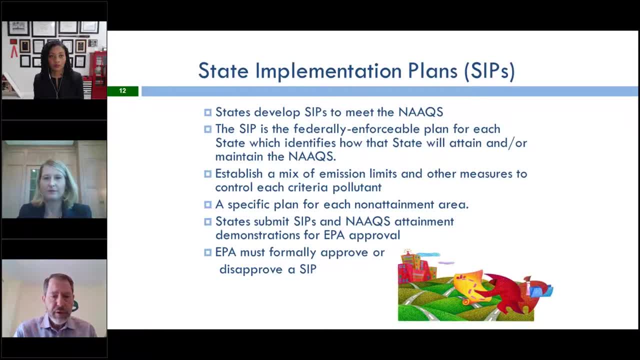 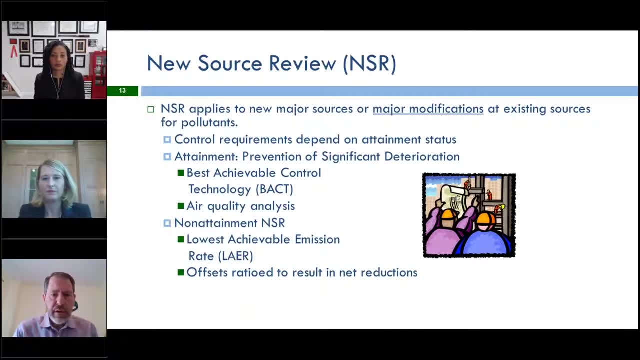 compliance with it, And EPA has to, by rulemaking, formally approve or disapprove a step. Next slide, NSR. I'm going to cover this pretty briefly because I know Stacy's going to talk a lot about it, But NSR applies to new major sources or major modifications at existing sources for pollutants. 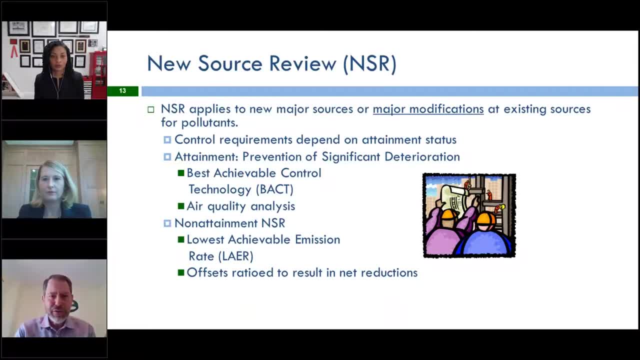 This is actually one of the most complicated parts of the Clean Air Act, just because of all the various issues around: what's a major modification, or even what's a source, and when are things going to change? Connected or not connected, and it can get very complicated. 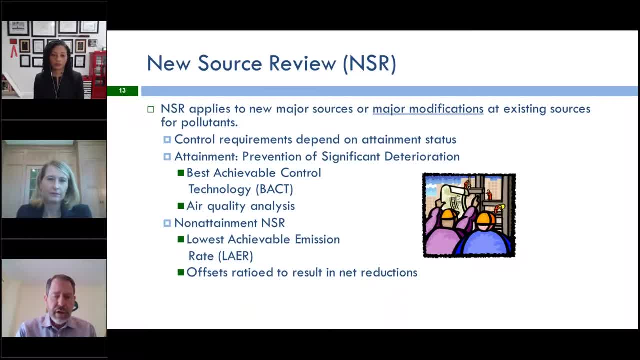 Control requirements depend on the attainment status. If you are in attainment for the relevant pollutant, then you have PSD prevention of significant deterioration and you have to put on best achievable control technology and do an air quality analysis to demonstrate that you will not cause the new action will not cause the area to go into violation of the NACs. For non-pollutants. the new action will not cause the area to go into violation of the NACs For non-pollutants. the new action will not cause the area to go into violation of the NACs For non-pollutants. 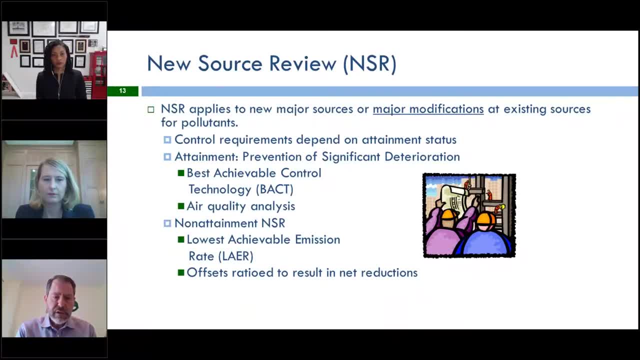 the new action will not cause the area to go into violation of the NACs. On attainment NSR, you have a tougher standard, lower achievable emission rate and you have offsets that are a ratio to result in that reduction. If you are going to be adding pollution, you have to find ways. other people who've 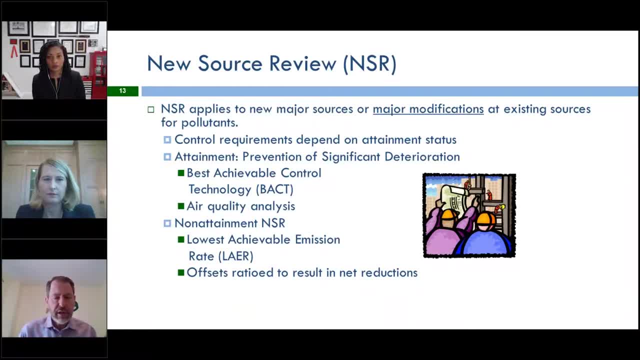 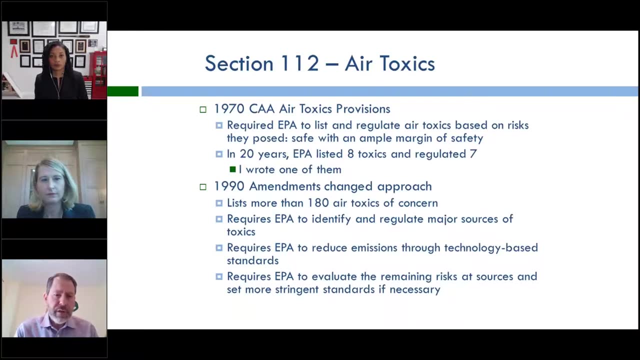 had reductions or if you're a large facility, you can do it internally and actually show that, as a result of the activity and the offsets, that there will be a net reduction in pollution. Next slide, Section 112, air toxics. 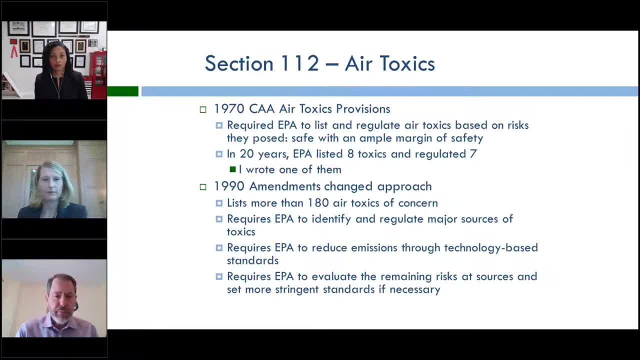 In 1970, the original Clean Air Act had air toxics provisions. They were required to list – EPA to list and regulate air toxics based on the risk they posed which was safe, with an ample margin of safety. In 20 years, EPA listed only eight toxics and regulated seven of them. 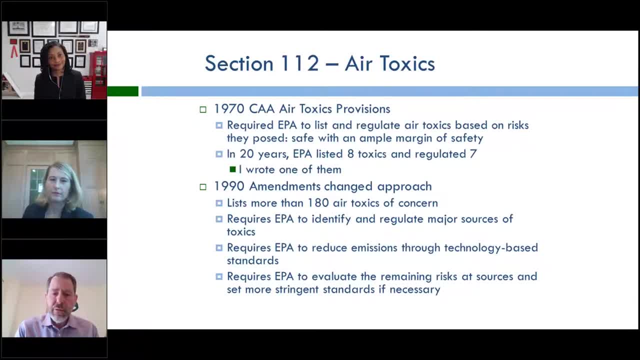 Probably one of the first major jobs I had at the agency was writing one of those – the air toxic standards for radionuclides. The problem was that it wasn't clear what exactly we were supposed to regulate and it wasn't – you know, an ample margin of safety is based on a complicated risk assessment. 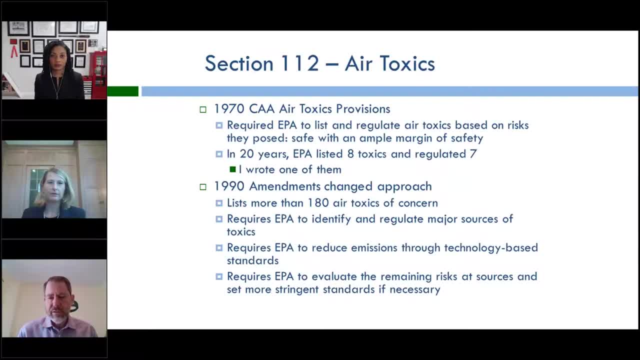 You have to get detailed information about each source, about the populations around them, and you have to do a lot of modeling. It was just a very complex – process designed to create – make everybody safe around it. So it was like – the goal was to have, in a way the – from an environmental and health. 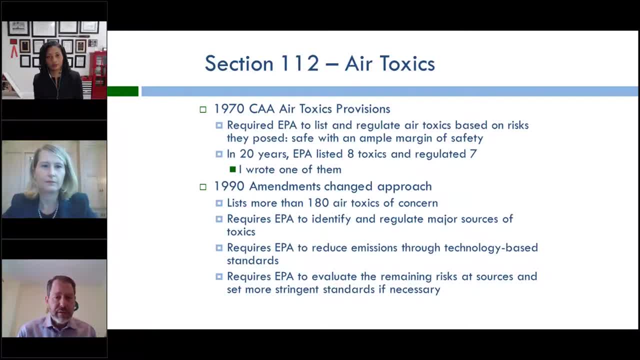 point of view, the best possible regulation, but it was a very complicated process, and so it was very difficult for EPA to actually implement in any way – in any large-scale way. So the 1990 Clean Air Act amendments changed that approach. 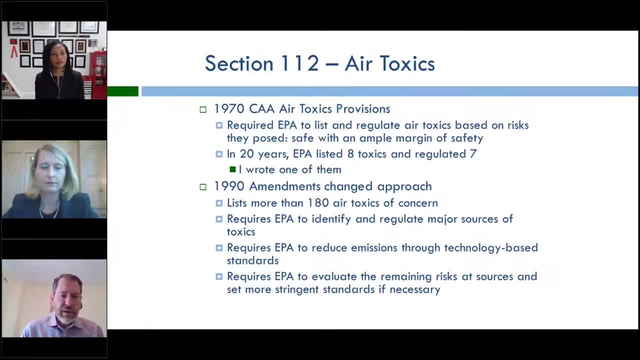 Instead of EPA having to list toxic, it actually listed a hundred and fifty – a hundred and eighty – air toxics of concern. It required EPA to then identify and regulate major sources of those toxic – major sources in this case being ten tons of any specific air toxic or twenty-five tons of all the. 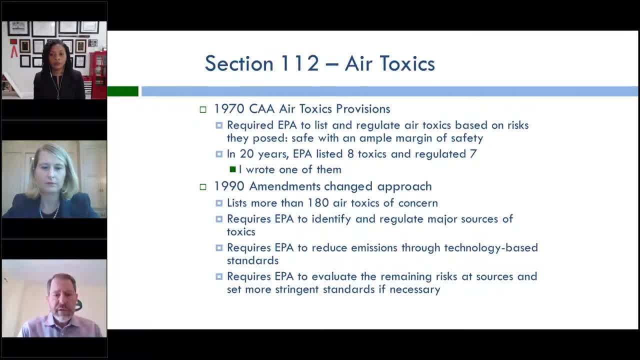 air toxics together. Air toxics are basically chemicals that are in and of themselves, are hazardous, poisonous, they cause cancer, they cause acute respiratory effects, things like that. EPA was required to emission – reduce emissions through technology-based standards and required to evaluate the remaining risks at those sources and set more stringent standards if necessary. 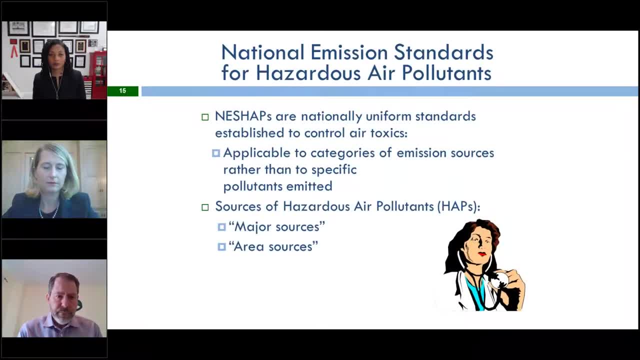 So let's – next slide. So the standards we set are national emission standards for hazardous air pollutants, the NESHAPs. They're national uniform standards established to control air toxics. They're applicable to categories. They're categories of emission sources rather than to specific pollutants emitted. 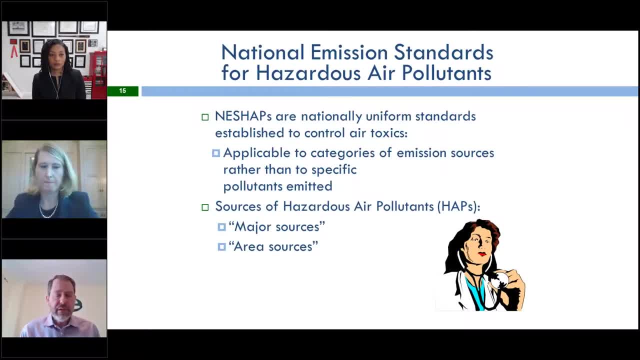 So, for example, when I said that we took these pollutants and then did source categories, so you have a chemical like benzene. Benzene comes from a lot of different facilities. One, for example, is a petroleum refinery. but a petroleum refinery also has a lot of. 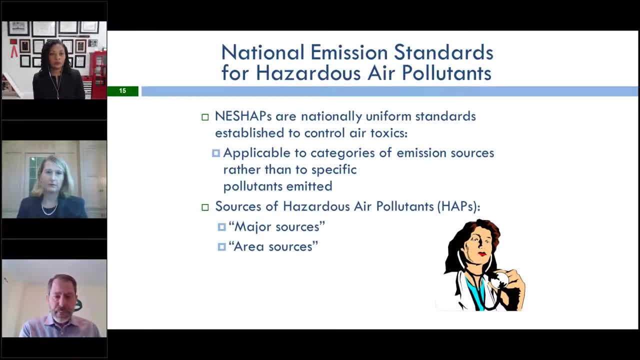 other emissions. So there are a number of different hazardous air pollutants that come from a petroleum refinery And instead of specifically targeting each one of those, we would just target the source as a whole. So we had emission source categories that would cover multiple pollutants all at once. 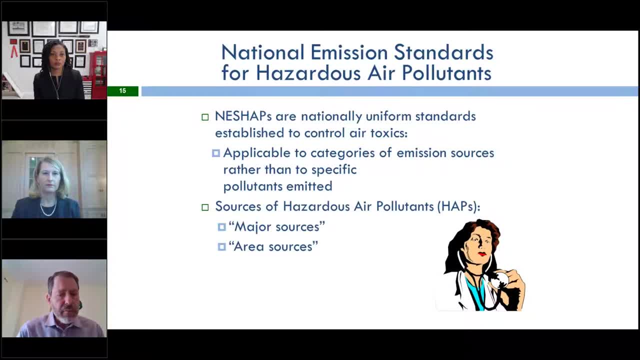 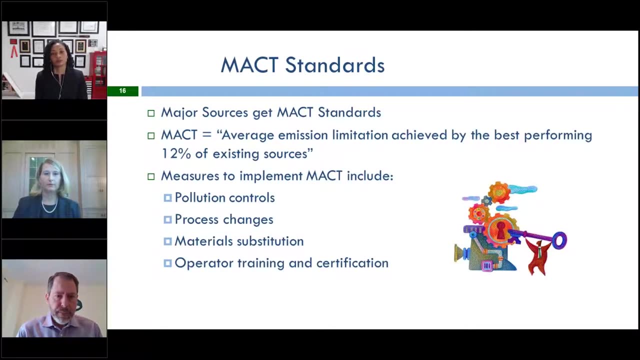 Sources of hazardous air pollutants, which we call HAPs, are major sources, which are the larger ones, or area sources, things more like dry cleaning facilities, gas stations, etc. Auto body shops, things like that. Next slide: 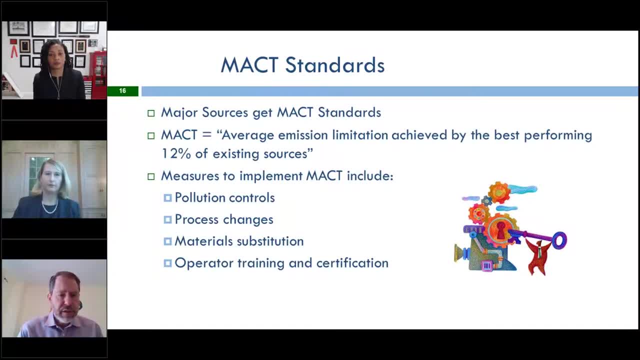 So the MAC standards, as I said, are technology based, So they're based on the average emission limitation achieved by the best performing 12% of existing sources. So if you had this source category and say there are 100 facilities, you look at the 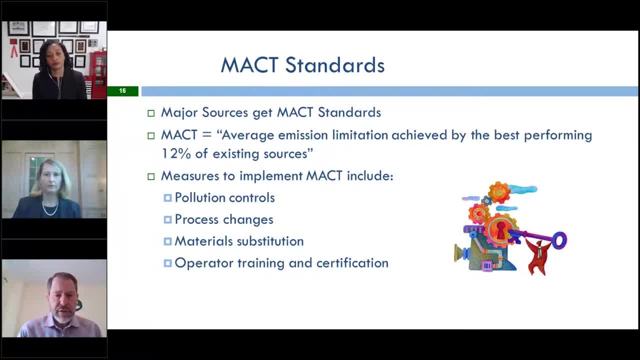 12, best performing in terms of emissions, farming, in terms of having the lowest emissions based on the control technology or work practices or materials they're using, and you just average that emission limitation and then that becomes the max. So it can be any one of a number of things. 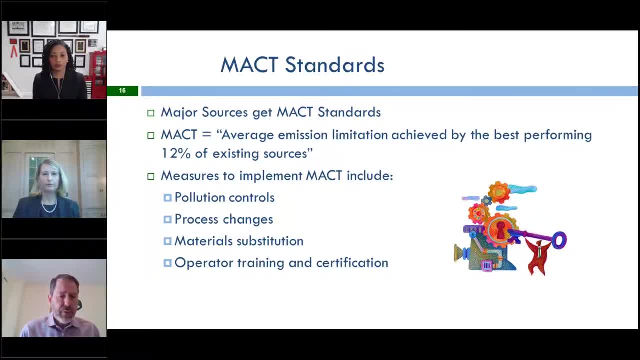 It doesn't have to be specific controls- Excuse me, It could be process changes, operator training, things like that. But this is you can see, is a much simpler process. You start with the chemicals. It's easy for us to know where the sources of those chemicals are, and it's also easy. 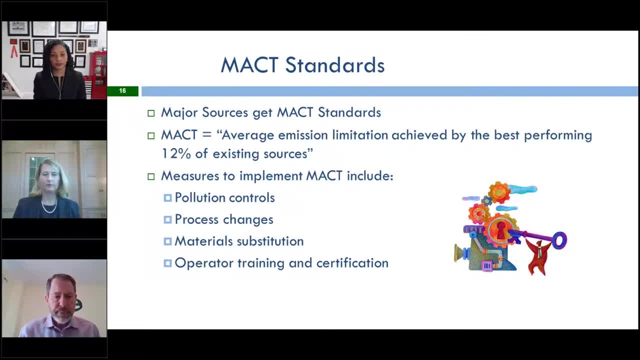 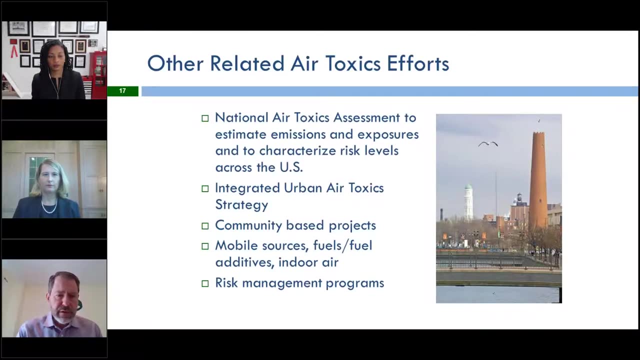 for us to know what kind of control equipment people are using or how they're producing it, And so we just average the best 12 percent, and that's the standard. Next slide: We have other efforts related to reducing air toxics. We have the National Air Toxic Assessment, or NADA, which produces the NADA data. 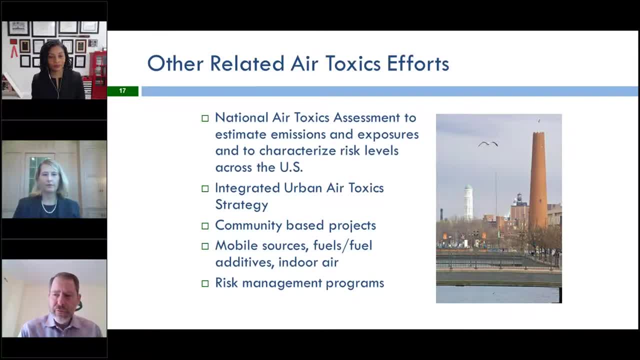 This estimates emissions and exposures and characterize risk levels from all toxic pollutants across the United States. This comes out about every three years. We have an integrated urban air toxic strategy to work on the smaller area sources found in urban areas. We have community-based projects. 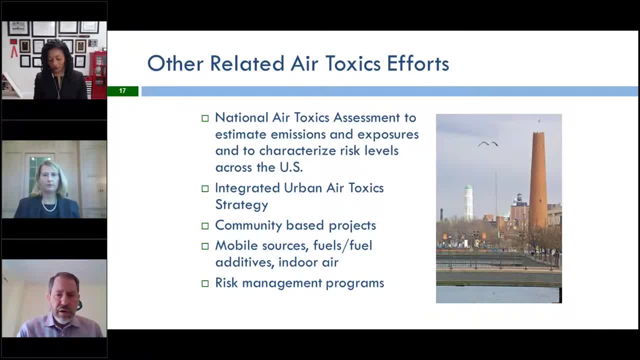 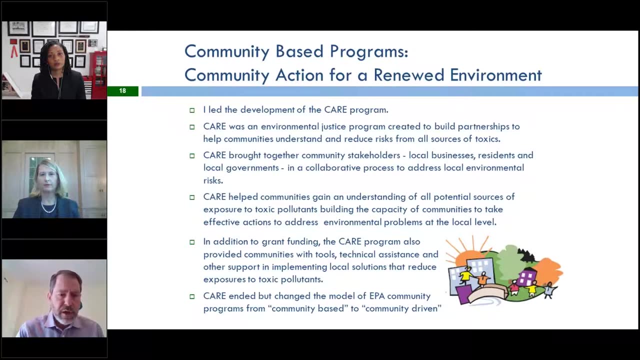 Mobile sources, fuels and fuel additives- all can release air toxics- and a number of other risk management programs. Next slide, So related to community-based programs, I'm going to just tell you about one that I led: the development of the Community Action for a Renewed Environment. 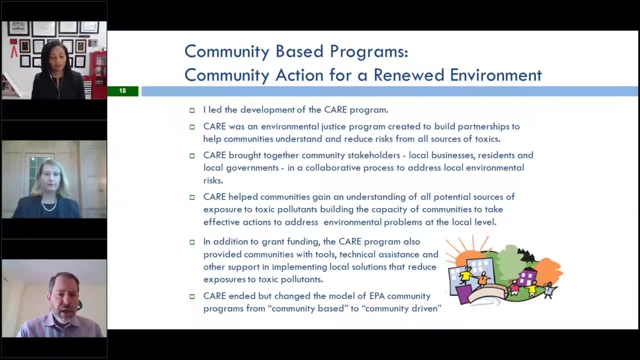 This was a groundbreaking EPA program designed to protect, help environmental justice communities. It was an effort to build partnerships. These partnerships would include the local community, the local government and the local businesses together to create this partnership, which would first look at all of the sources. 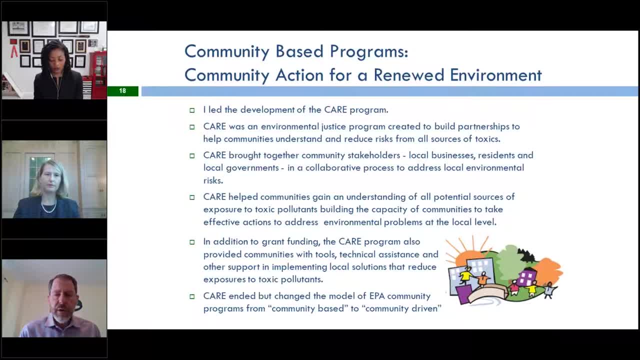 of air toxics and risk in those communities and then help the community decide on their own what problems they wanted to tackle, what were most important to them. Next slide, Next slide. So by doing this, the communities would gain an understanding of the potential sources. 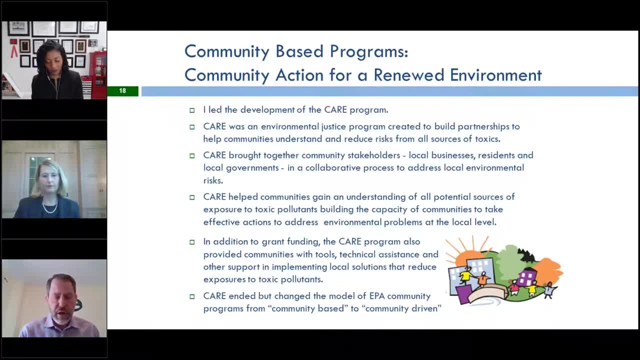 and they would also. what CARE did, which was different, was normally what had happened before, that was, say, the air program had something for air toxics and the water program had a water program, something dealing with local water issues, And all the different offices were all kind of their own little fiefdoms and people weren't 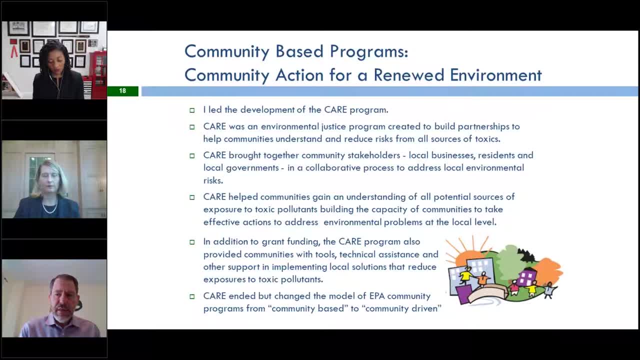 working together, Next slide, Next slide, And so the thing that was really fascinating is when people come to the local government, when people see the air office. we're actually lucky if people in communities see EPA as not the entire federal government, So people would often be frustrated because they might get an air grant. but really the 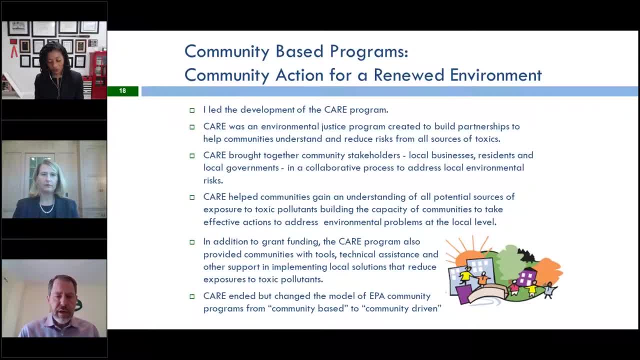 water issues were more important, And so what CARE did is we created this multimedia way to provide communities with tools, technical assistance and other supports so they could implement the solutions they wanted. It's kind of, in a way, instead of doing centers. 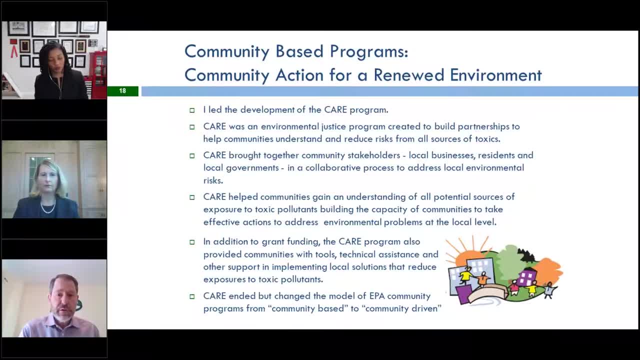 You know, the example I used at the time was Dell Computers, because Dell Computers had figured out how to do mass customerization. You could have, you know, they could build a million different types of computers with all the different features, but they were mass producing them for each individual. 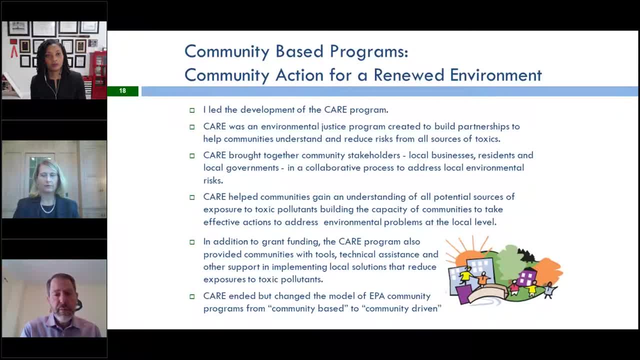 And so here, instead of EPA saying you have to take this program because you happen to qualify for this grant, we were giving them a grant and we were saying: what do you care about? and here are all the choices and you take from them. 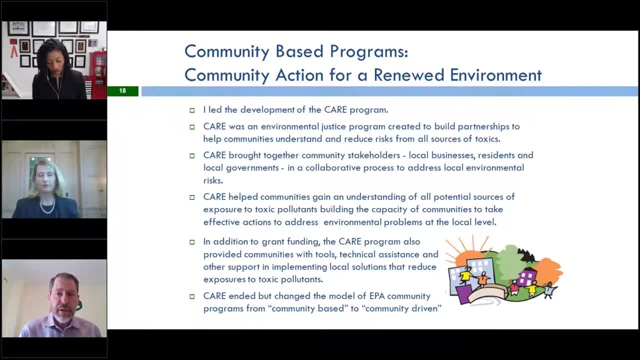 One of the things that was important was to really change the attitude of people at EPA, because people were a lot of the technical people in particular- were saying: what if the community chooses wrong? And what we were trying to do was saying that was impossible because, by definition, 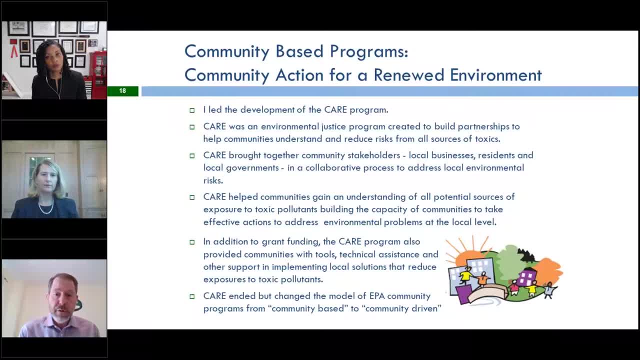 what the community viewed as the most important risk was the most important risk, and that's what we should be working on, And so what we? by doing that, we changed the model of EPA community programs from community based- things happening in communities- to community driven where the action was driven. 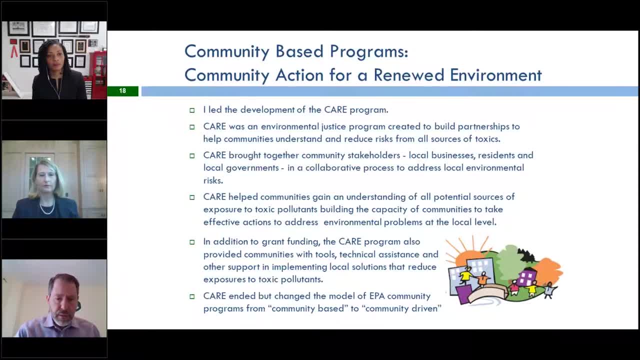 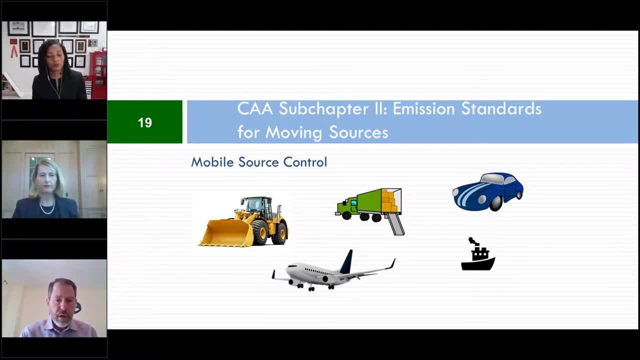 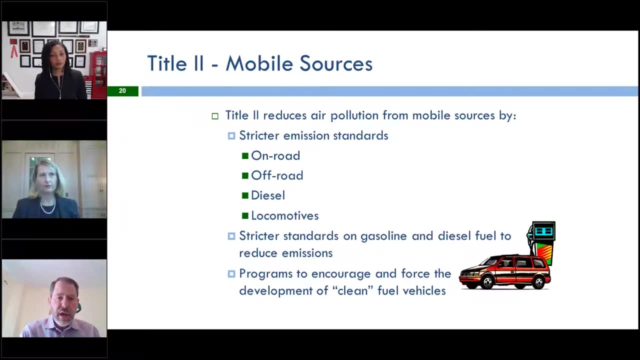 by the community and what it was trying to do. Next slide: So we're going to talk about mobile sources now. Next slide, please. So Title II of the Clean Air Act. It reduces air pollution from mobile sources by having stricter emission standards for 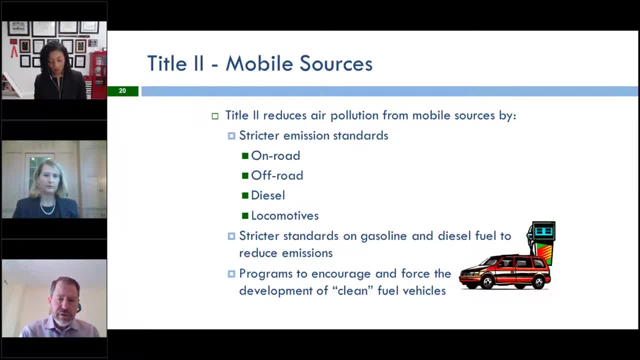 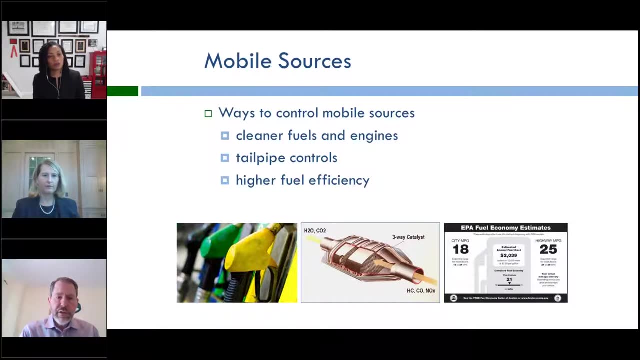 on-road, off-road diesel and locomotives. These stricter standards, also on gasoline and the fuel to help reduce emissions, and programs to encourage and force the development of clean fuel vehicles. Next slide. So there are basically three ways to control emissions from mobile sources. 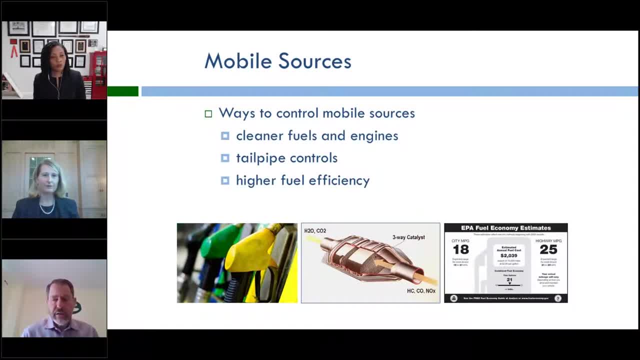 You can have cleaner fuels and cleaner engines, So the actual- If the actual- engine produces less pollution or cleaner fuels. for example, in the winter we are more concerned about carbon monoxide because the cold engines don't burn as efficiently And so you can have the carbon that's in gasoline instead of burning all the way to create carbon. 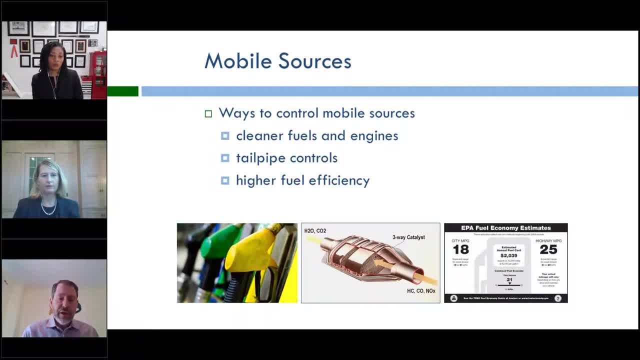 dioxide, which has its own issues, but at least for the people who live in the city or are near where the engine is actually operating. Next slide: It's not immediately, you know, poisonous, but carbon monoxide is a poison, And so, like when you know when people would commit suicide by running their car engine. 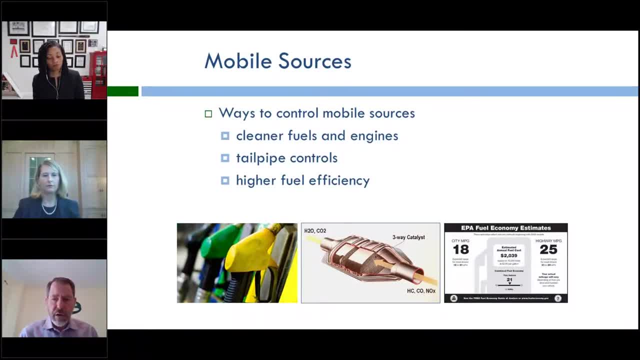 in a garage. what was killing them was the carbon monoxide, And so we have add more oxygen to the fuel, so there's more oxygen in the mix and so you get less carbon monoxide, but in the summer because, as I was showing earlier, you have. 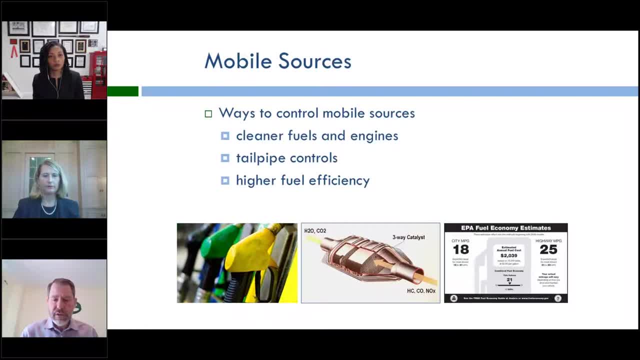 oxygen creation in the hot sun. you care more about having less VOCs, and so you care about how much evaporation there is in the gasoline. So gasoline is reformulated so that it is less, has lower evaporation. It's called Reed vapor pressure, which is just a measurement of how quickly something evaporates. You can also have tailpipe controls, for example a catalytic converter, and you can also just increase the fuel output. You can increase the fuel efficiency so that there's less fuel that's being burnt, so that there would be less pollution coming out of the tailpipe. 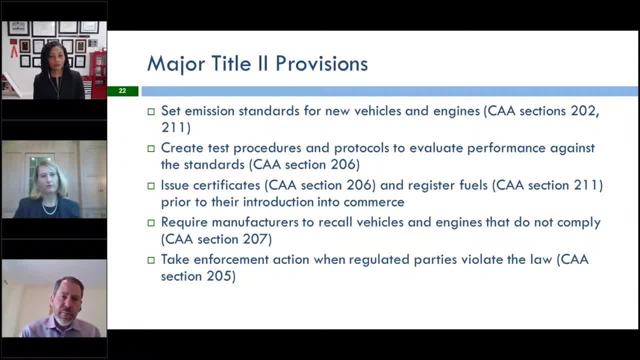 Next slide. So there are a number of major Title II provisions. There are emission standards for new vehicles and engines. There are test procedures and protocols to evaluate performance against those standards. So you, we issue certificates and register fuels prior to their introduction into commerce. 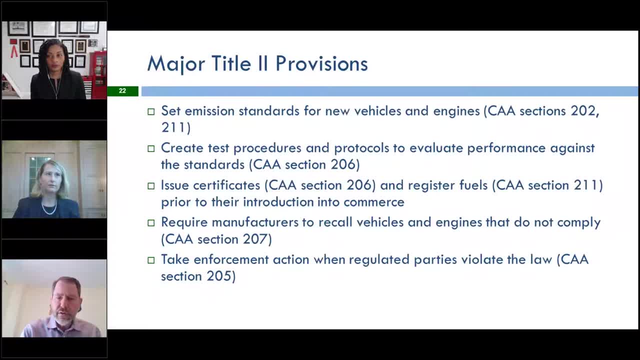 We can require manufacturers to recall vehicles and engines that don't comply and take enforcement action. So we have a lab in Ann Arbor. If you have a new car, you're a car manufacturer. that car has to get shipped to Ann Arbor so it can be tested to make sure that it meets Clean Air Act requirements for emissions. 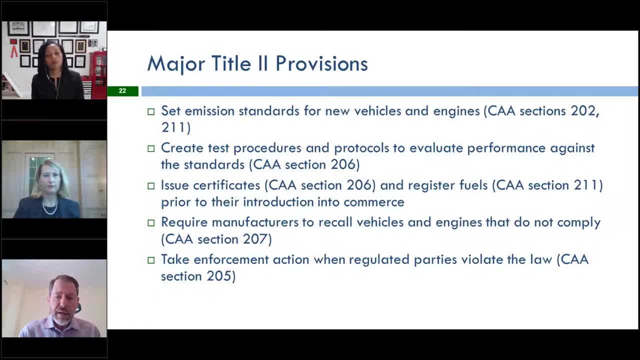 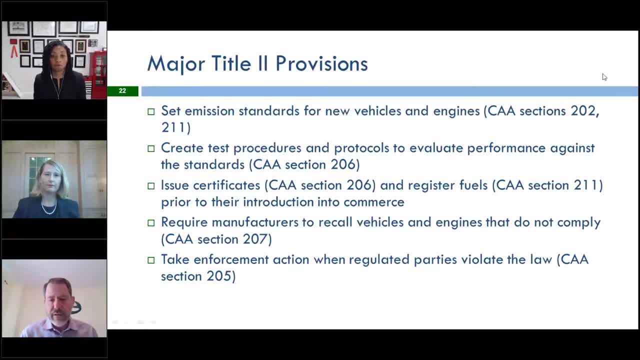 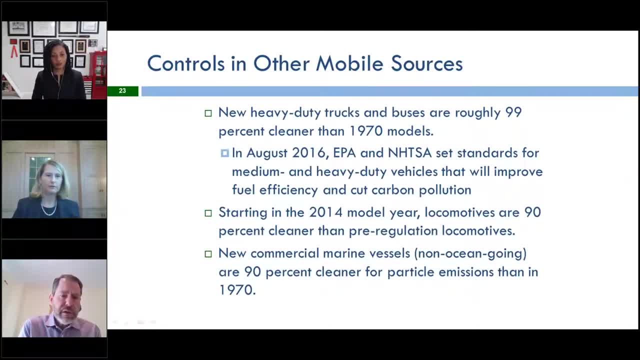 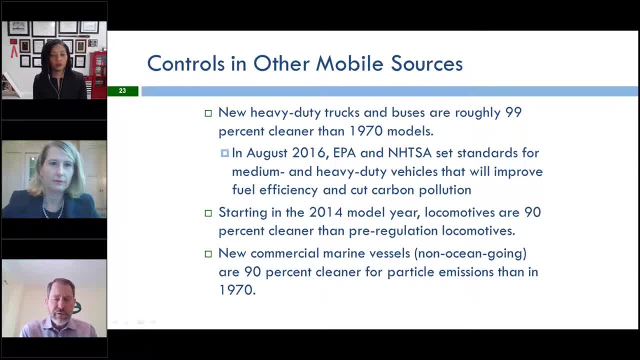 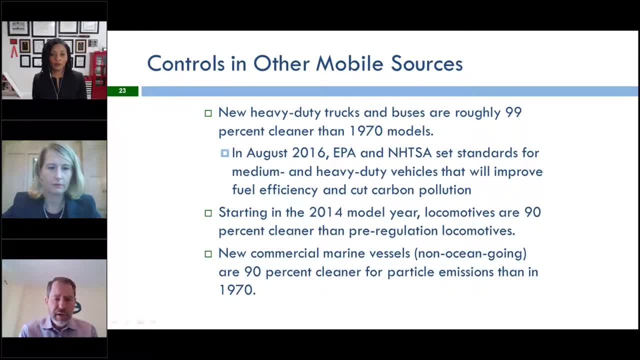 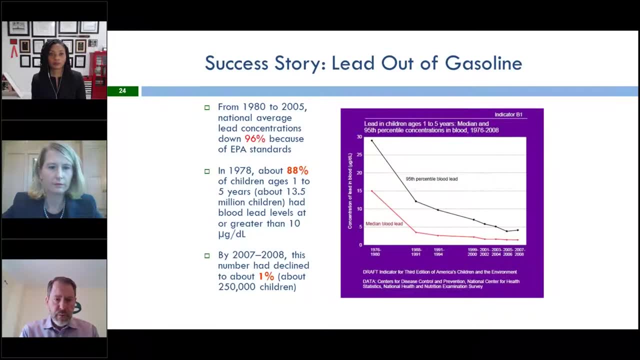 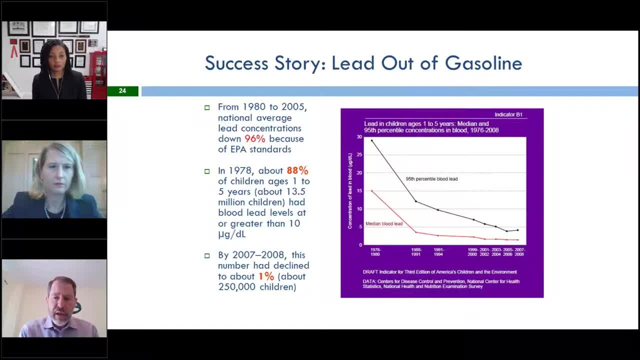 gasoline, both because it was a pollutant and because it prevented catalytic converters from working properly. So one of the major emission control devices on a car is the catalytic converter, which converts the hydrocarbons such as like benzene or other toxic chemicals. 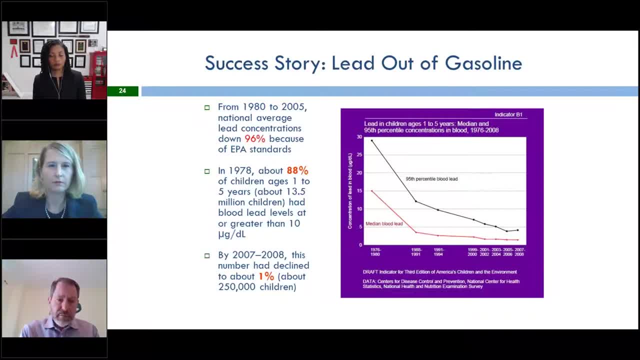 into just carbon dioxide and water. And to do that, the lead- there's a catalyst on this honeycomb that interacts with the air, and the lead would interfere with the catalyst. so the catalytic converters couldn't work, And so we took the lead out of gasoline. It resulted in 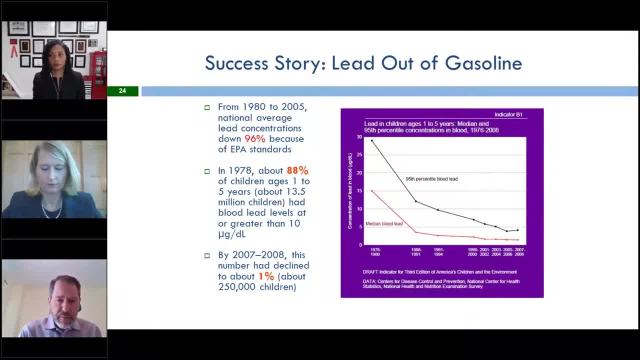 enormous health improvements. as you can see from the graph here, In 78,, about 88% of children between the ages of one and five years had blood lead levels at, or greater than, 10 micrograms per deciliter, which is kind of this measurement of level of concern. And by 2007,- 2008,, this number 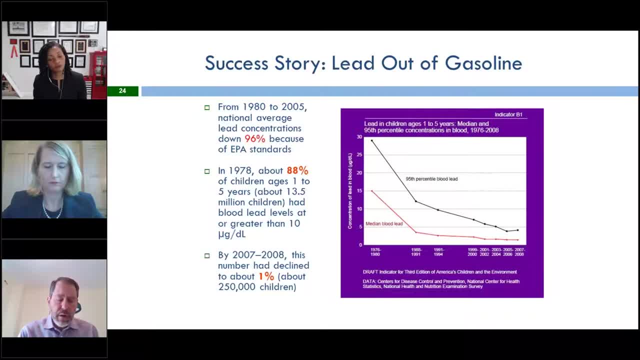 declined to about 1%. So right now I mean there are lead issues, but they're mostly either from water lead pipes, lead in pipes, or from people who live near things like lead smelters. This has been a big health improvement And even some economists have said that part of the large 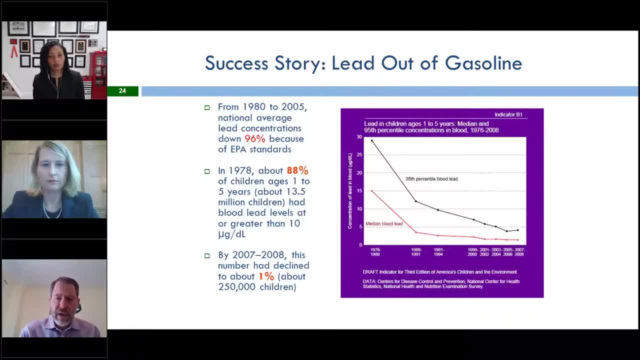 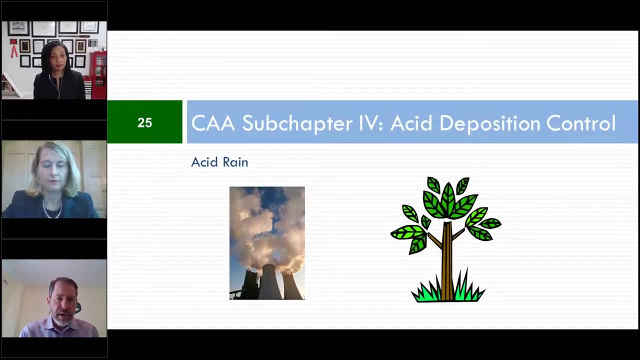 decline in crime between the 80s, 90s and today is in due in part to this reduction in lead poisoning, because lead poisoning affects the brain and ability for self-control and ability to learn. Next slide: Acid rain. Next slide, chapter four. So this is acid rain control. 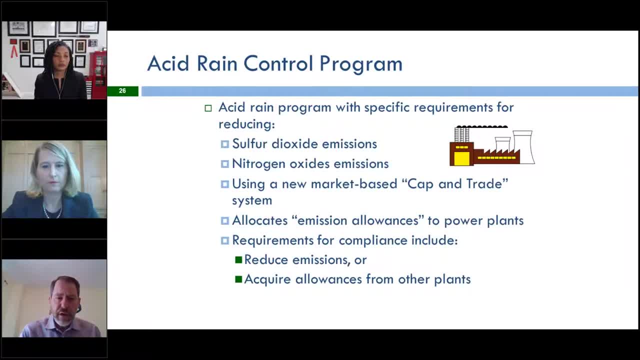 program. It has specific requirements for reducing sulfur dioxide and nitrogen oxide emissions using a cap-and-trade system for power plants. It allocates emission allowances to these power plants, And so a facility might get 100,000 allowances, which meant that they could emit. 100,000 tons of sulfur dioxide, And so we put continuous emission monitors on their stacks so we knew exactly how much was going out, And at the end of the year, the facility had to have 100,000 allowances for their 100,000. tons of emissions Each year. that number of emissions, the allowances that they got would go down. So they had to either reduce emissions or they had to acquire allowances from other facilities. So if they put on a scrubber they wouldn't get 10% reduction, they would get maybe. 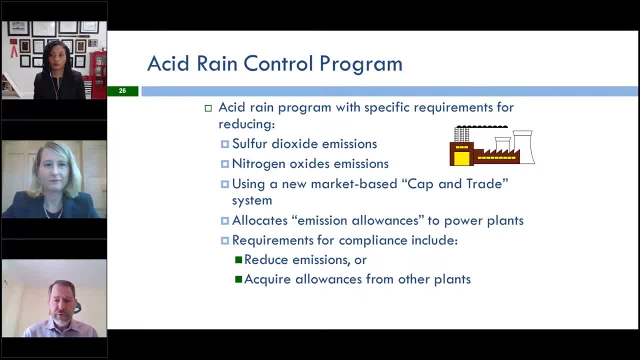 a 90% reduction, And so if they only needed, in the first few years, 10% or 20% reduction, they had a lot of extra allowances they weren't using. They could sell those to other facilities so that they, instead of putting on a scrubber, would just buy these allowances, or they could bank. 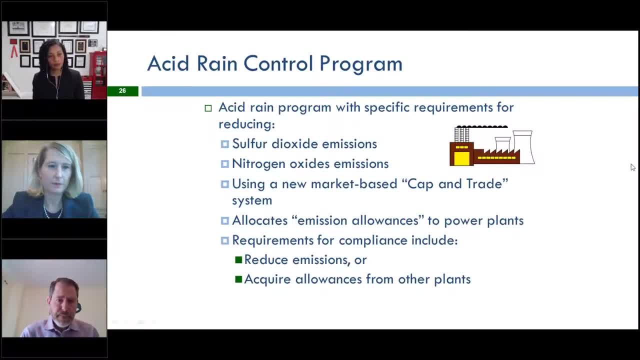 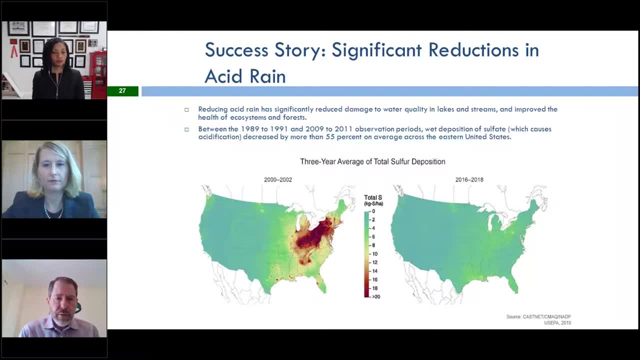 them for future use. Next slide: This program was extremely successful. We got enormous reductions. We had an increase in sulfur and nitrogen oxide emissions, much less acid pollution in the lakes and streams of the Northeast. We also, as you can see in the slide, where you have the three-year average of total sulfur, 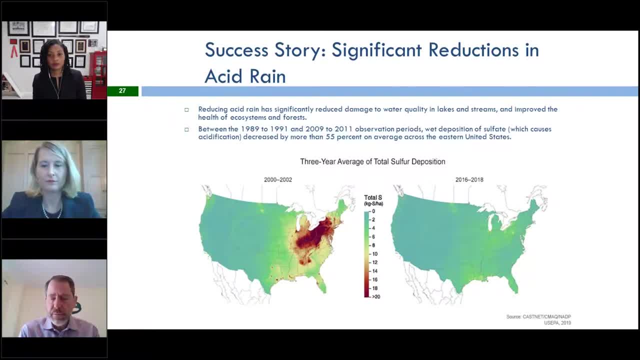 deposition dropping dramatically, decreasing by 55% on average across the Eastern US, But it did more than improve environmental quality. We had an increase in sulfur and nitrogen oxide emissions, much less acid pollution in the lakes and streams of the Northeast, But it did more than improve environmental. 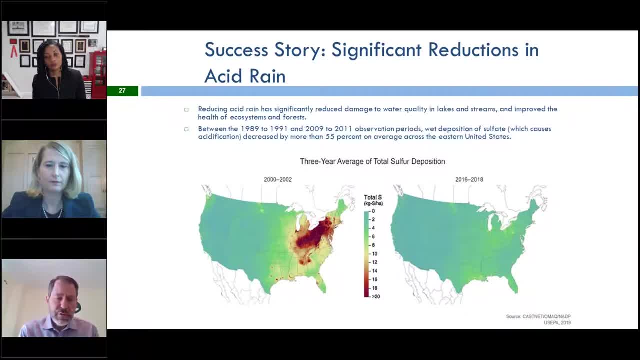 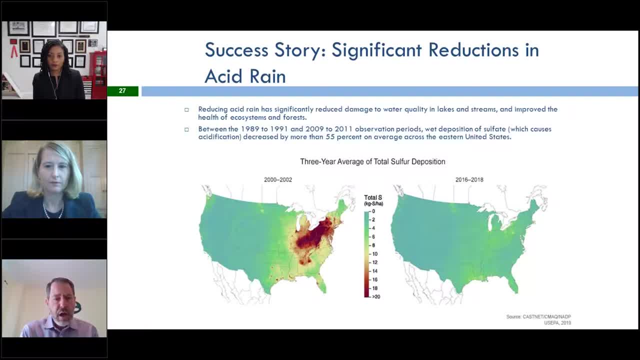 which are among the most dangerous air pollutants that there are in terms of a public health point of view, And, in fact, the Acid Rain Program. there is this thing called the Thompson Report, which analyzes from the Office of Management and Budget how much emission reduction there's. 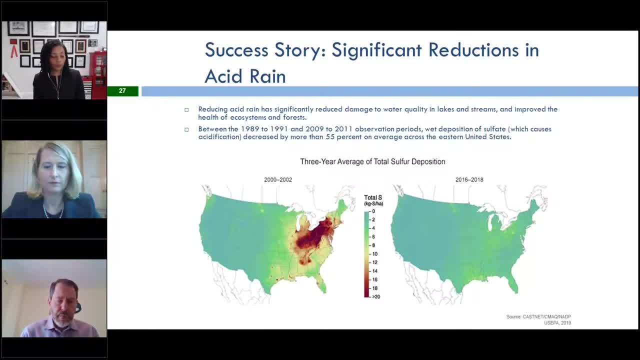 been in those areas. Next slide, Next slide. I'm sorry how much benefit we've gotten from regulation And, in part because of the massive benefits of the Acid Rain Program and the Clean Air Act as a whole, the Office of Air and Radiation has more benefits from regulation than the. 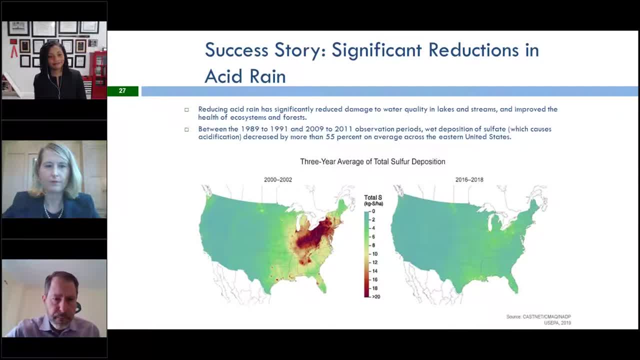 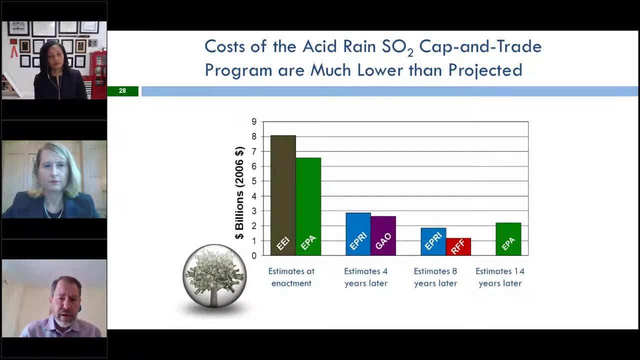 entire rest of the federal government. Next slide. We also got these reductions way more efficiently than was expected. Because of this marketplace system, people were able to trade and get emission reductions for a lot less money. You can see about a quarter of initial estimates. 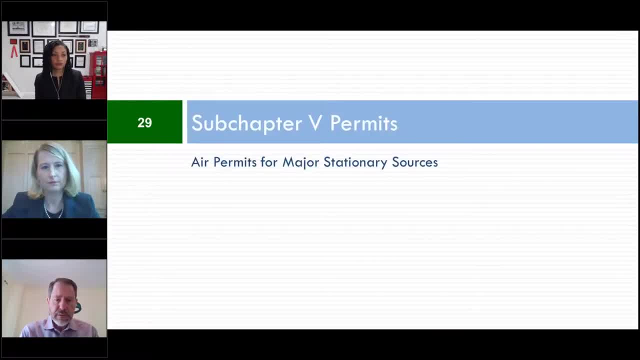 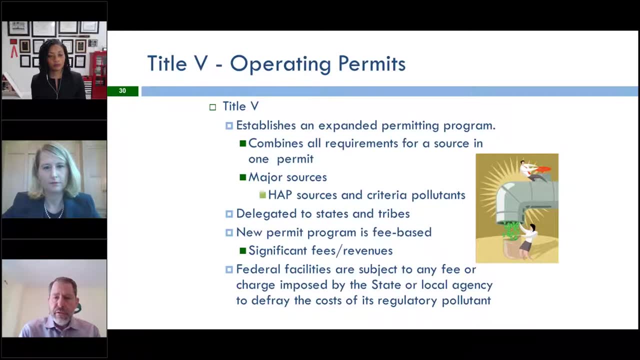 Next slide. Okay, Permits Next slide, please. So Title V established operating permits for facilities It combined – the permits were great because they would combine all their requirements for a source in one place. It was for major sources, which perhaps, as I said, was 10 times any toxic or 25 all combined. 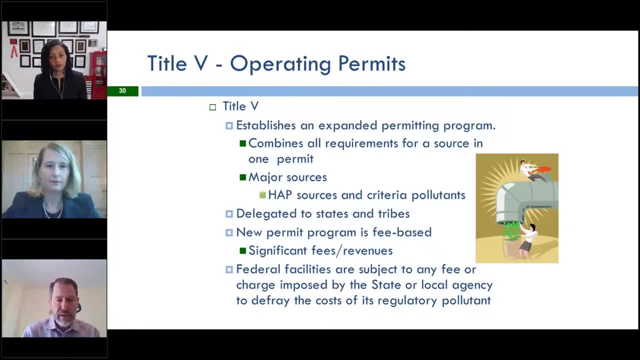 toxics, or 100 times for criteria pollutants related to the now The title –. that permit program was delegated to states and tribes And there were permit fees attached And those permit fees had to be significant enough to pay for the program. So when states created their program they had to send it to the state. 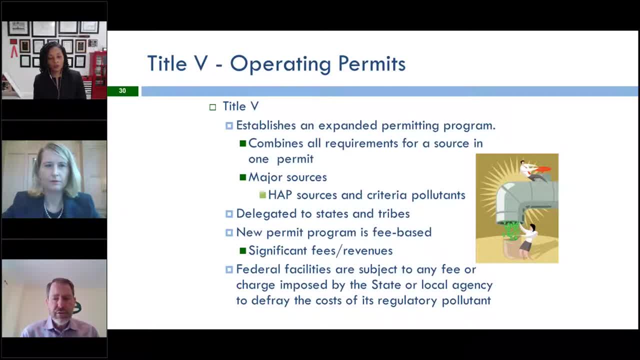 They had to send it to EPA for approval And one of the main issues- because states were trying to have the permit fees be low, because politicians didn't want the facilities to have to pay a lot- was they had to demonstrate that they were raising enough money to pay for the program. 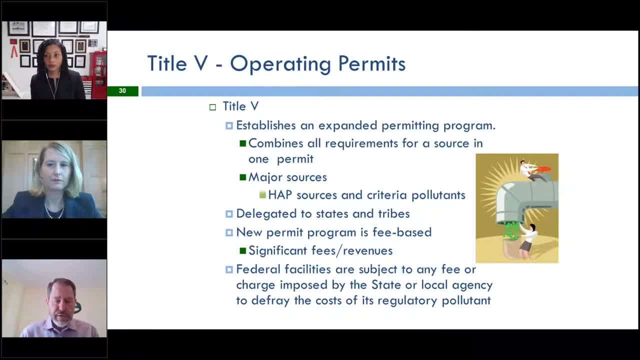 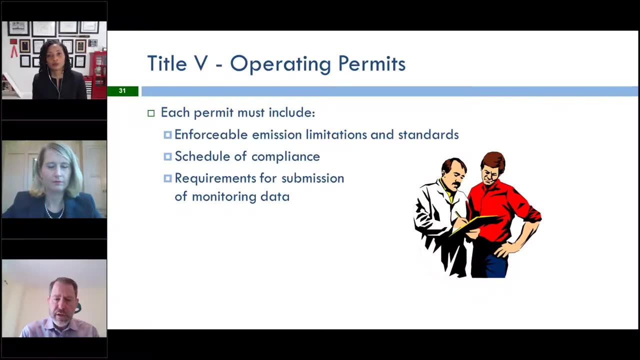 Federal facilities are not subject – are subject to separate fees to defray the cost of regulation Next slide. So each permit must include enforceable emission limitations and standards, a schedule of compliance and requirements for submission and monitoring data. A lot of what we know about emissions from facilities come from these reports that are 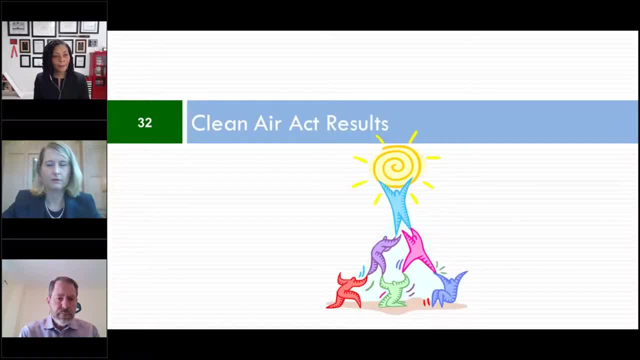 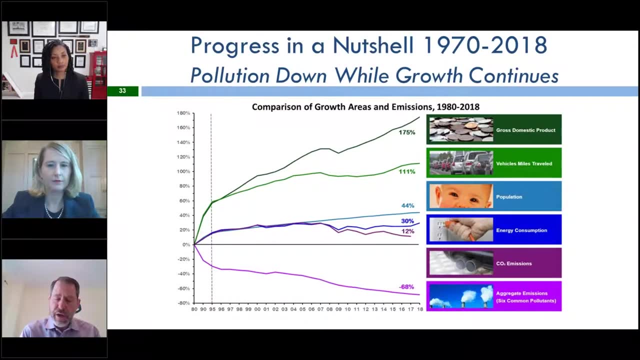 required in the permit. Next slide: Okay, So let's quickly talk about some results of the Clean Air Act. This is one of EPA's favorite slides. It compares: It's the growth of the economy from 1980 to 2018.. 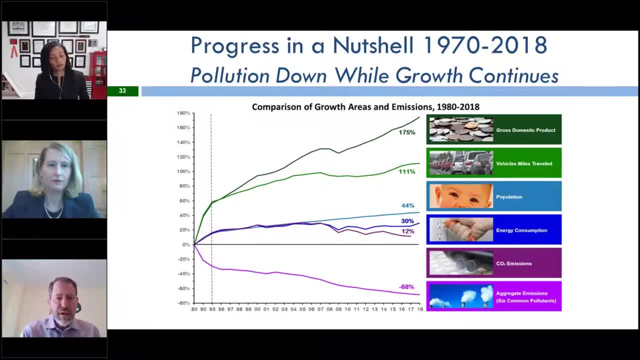 And you can see. the gross domestic product has increased almost 200 percent, Vehicle miles traveled over 111 percent, The population's increased by 44 percent. Energy consumption and carbon dioxide emissions are up although they're – at least those are- trending down a little. 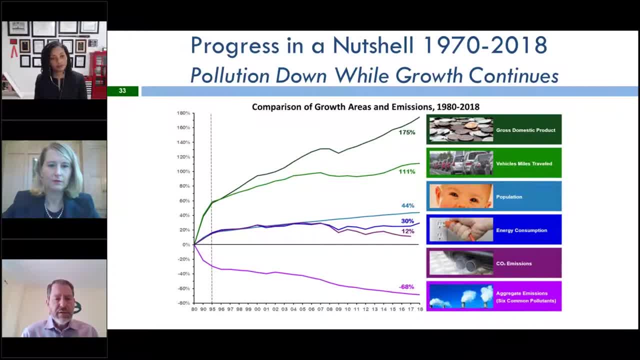 So all these things that you would expect would result in pollution. despite all of this, economic growth, increased activity, more people- Next slide: The aggregate emissions of the six common pollutants related to the NACs are down 68 percent. Next slide. 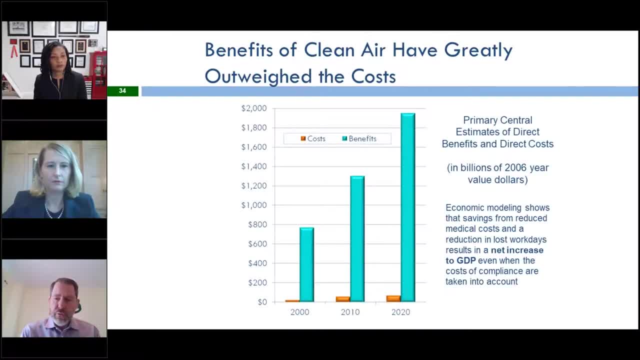 It was a requirement in the 1990 Clean Air Act amendments that we do a heavily reviewed study of the benefits of the Clean Air Act, which have greatly exceeded the cost. So you have here a slide for the central estimates of direct benefits. Next slide: 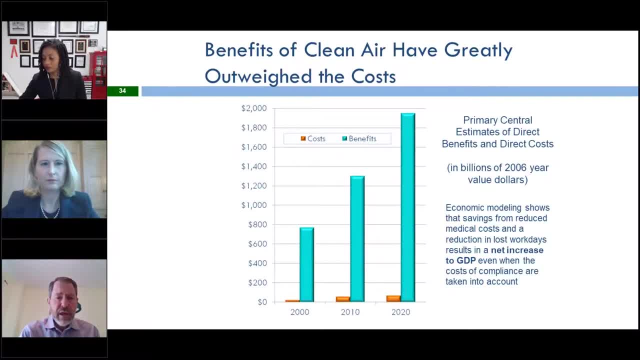 Next slide, Next slide. So you have direct benefits of cost in billions of dollars. So you're talking about this year, almost $2 trillion in benefits for around $60 billion in cost. Most of those benefits are the monetized value of the over 200,000 lives saved a year from. 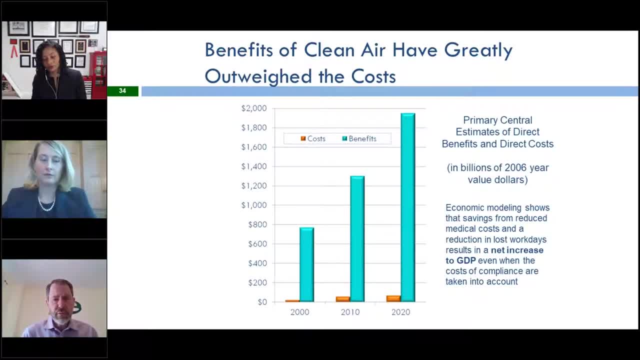 the Clean Air Act. but the economic modeling shows that just in terms of the health benefits of people. So first slide. So if you're going to work, not being sick so they can't go to work, the medical costs of people going to the hospital or for asthma attacks or not being able to go to work because 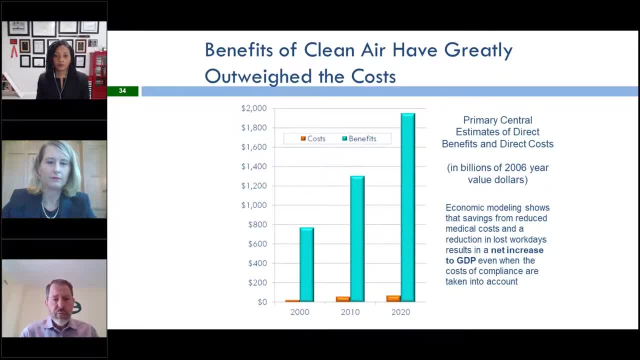 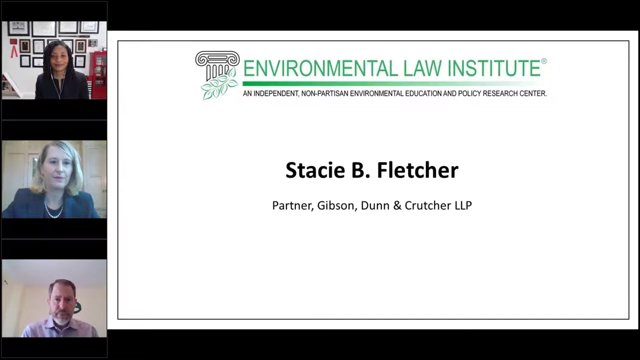 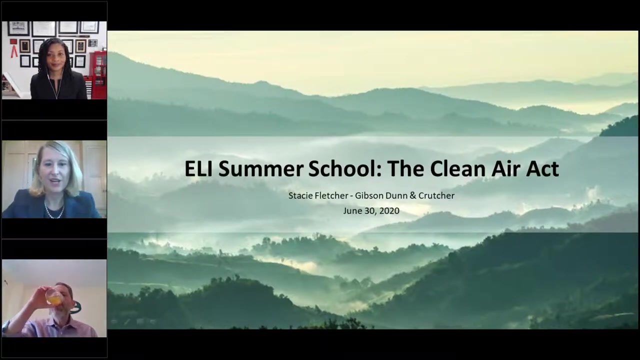 their children are sick. that economic value alone, excluding any of the value of the health impact or the improved environmental quality, those economic benefits alone more than offset all the cost of the Clean Air Act. Next slide, Next slide. that's it. Thank you so much, Larry. We will now turn to Stacy. Well, hello everyone and thanks. 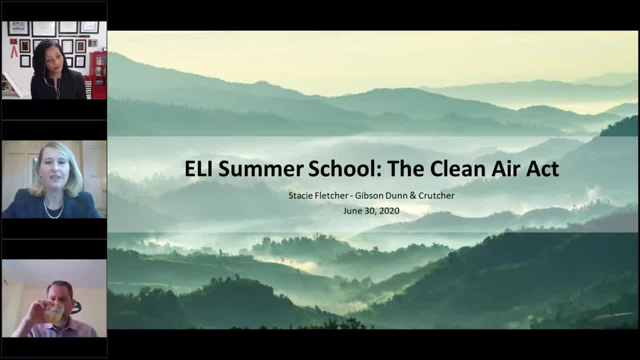 for joining us. I hope you can hear me, okay, Caitlin. Perfectly Great, thank you. Well, Larry has provided such an excellent overview of the Clean Air Act and its conceptual framework, so he's a tough act to follow. What I'm going to do in my presentation is take a deeper look at three 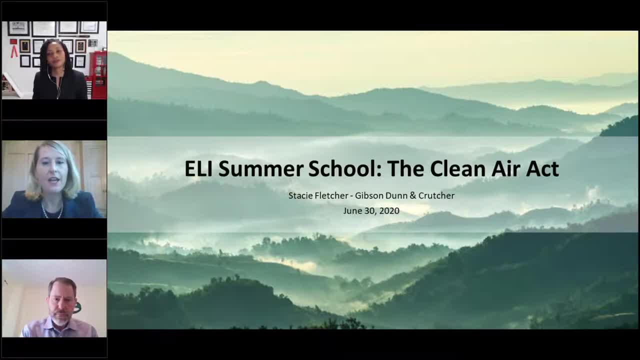 key Clean Air Act programs for stationary sources and states and talk about how those programs are implemented in practice. So, in particular, I'm going to focus on practical tips for determining the applicability of a Clean Air Act program to stationary sources and also how to determine the 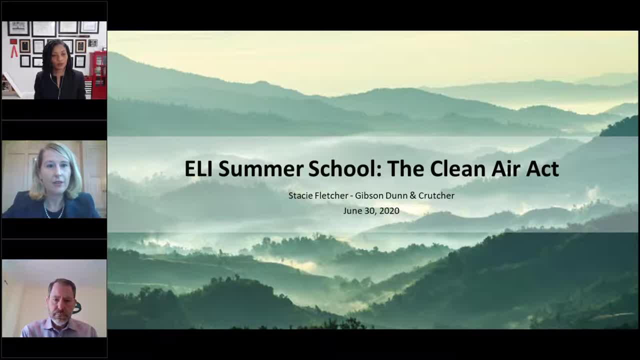 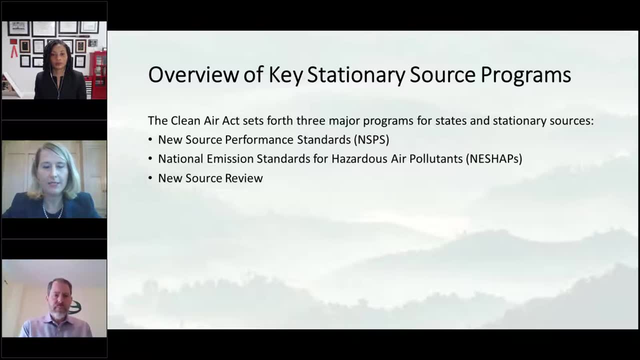 relevant requirements that could apply. Could I have the first slide, please? The three programs that I'm going to focus on today are: New Source Performance Standards, which we call NSPS, the National Emission Standards for Hazardous Air Pollutants, called NESHAPs, and New Source Review. 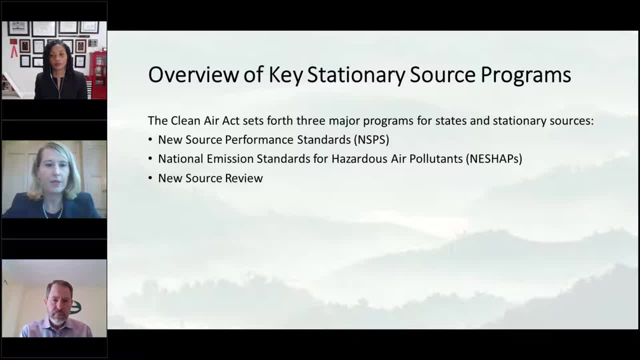 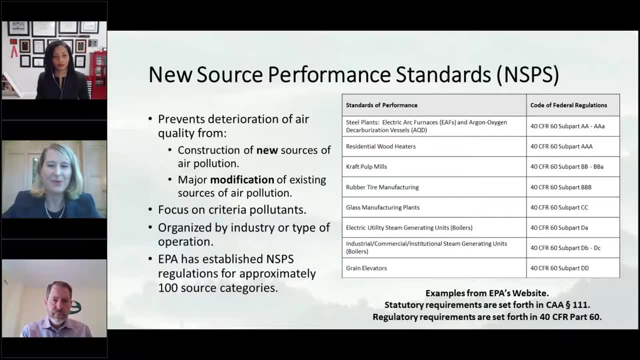 For stationary sources and their states. these are key programs from a compliance and enforcement perspective. So next slide, and you can go ahead and continue. We're going to start with New Source Performance Standards. New Source Performance Standards- New Source Performance Standards, or NSPS, address criteria: pollutants in their precursors. 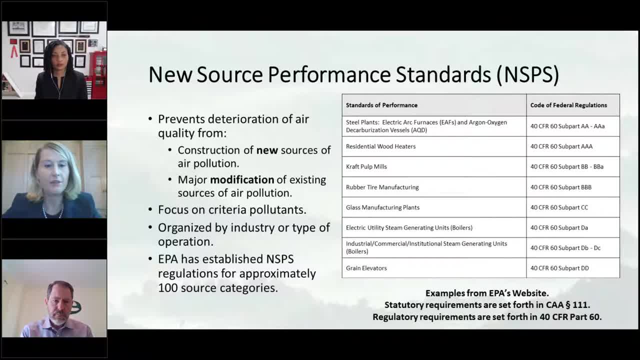 such as VOCs, and are aimed at preventing deterioration of air quality from new and modified sources. NSPS regulations are generally organized by industry, So you'll see an example here, on the right-hand side of the slide, that EPA develops NSPS regulations for paper mills. 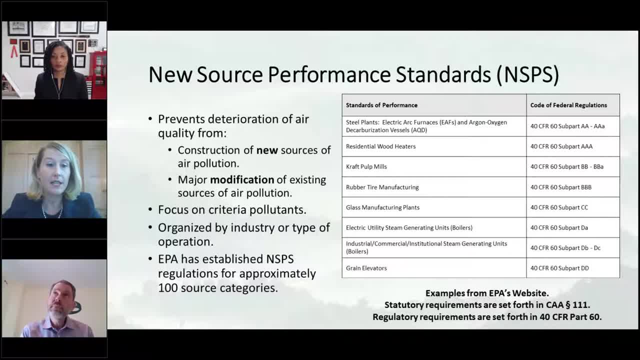 glass manufacturers, boilers, refineries- These are just to name a few, but generally they're organized by type of air. New Source Performance Standards, areico- These are품. Currently there are 100 source NSPS regulations and they can be found at 40 CFR, Part 60.. 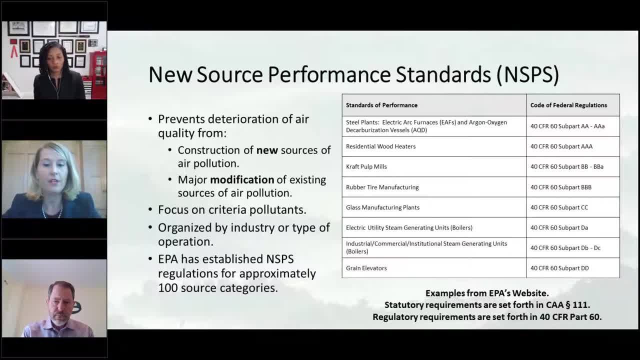 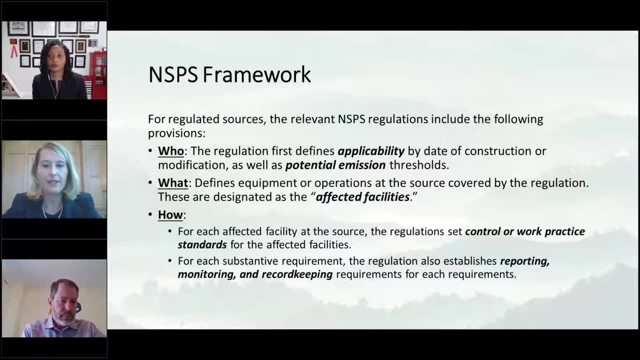 In general, they're organized, as I said, by industry or operation, with each subpart having its own alphabetic designation, as you can see from the right-hand side of the slide. Can I have the next slide, please, For each particular NSPS? that's the self-contained source or type of operation governed by this. 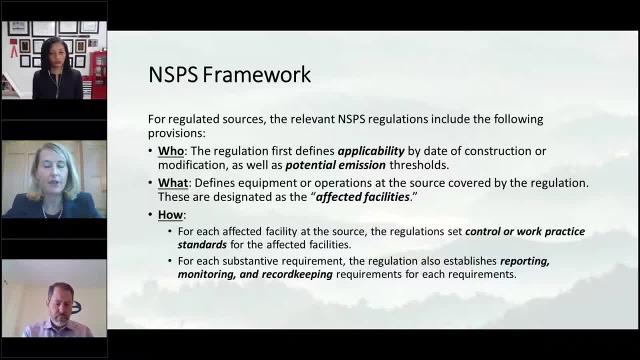 program. the regulation is generally self-contained and follows the following framework. First, the regulation defines applicability. This will be based on the date of construction or modification and also the potential emissions from the regulated sources. We'll discuss potential to emit later in this presentation, but for present purposes I 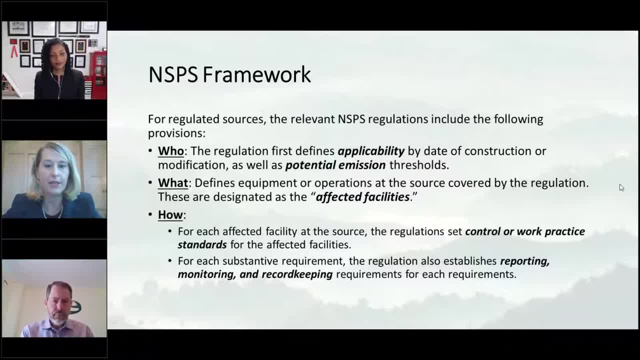 just wanted to flag. It's a two-pronged test for NSPS applicability. Second, the NSPS defines source and operation. This is how the regulation defines operational costs and or operating costs and the terms of each fiscal year and the terms of the last fiscal year. 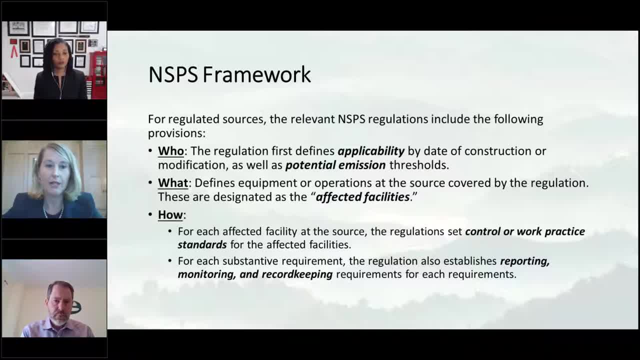 The rules are basically the same. I'll talk about those in a little bit. So the NSPS is defined as the number of operating costs that should be covered within that facility, not the cut cost of the facility. And then the items that are indicated in the regulations are the cost of equipment, whether 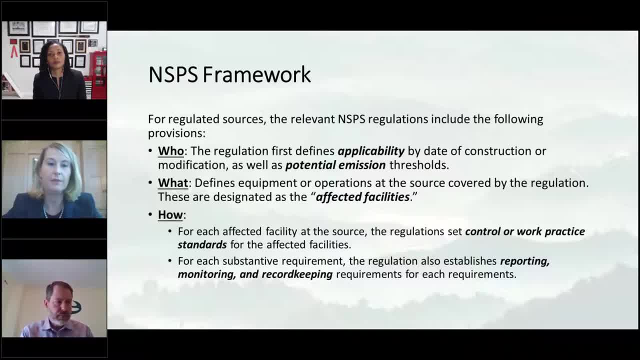 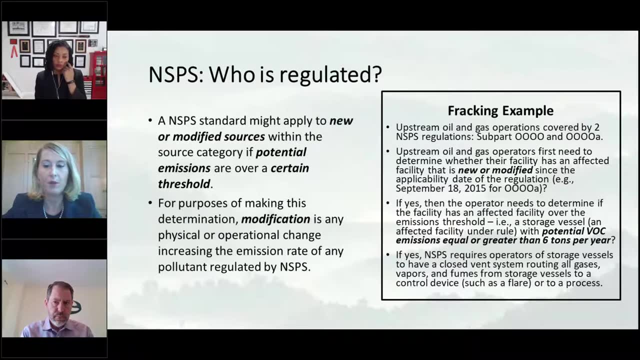 it's the facilities or the services and also the cost of any kind of equipment. So I'll show you what the rules are. The rules that facility, those are known as the effective facilities within the nsps. third, for each effective facility, the nsps will have the substantive requirements. 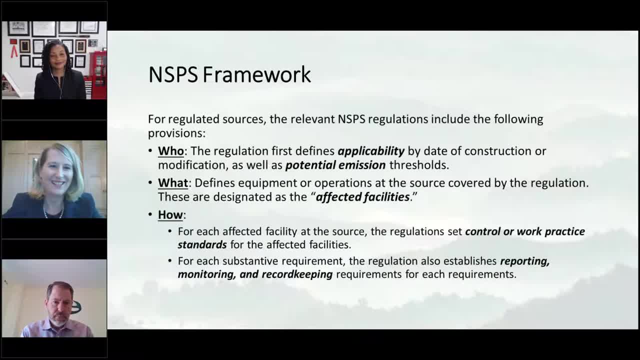 oh, um, you can go back one side. sorry, i think i will have the substantive requirements and how you determine compliance for each of those effective facilities. so, for example, that will look like a numerical limitation, such as a concentration limit expressed as ppm or ppb, or it could be the efficiency of a control that says if you have these types of emissions you have. 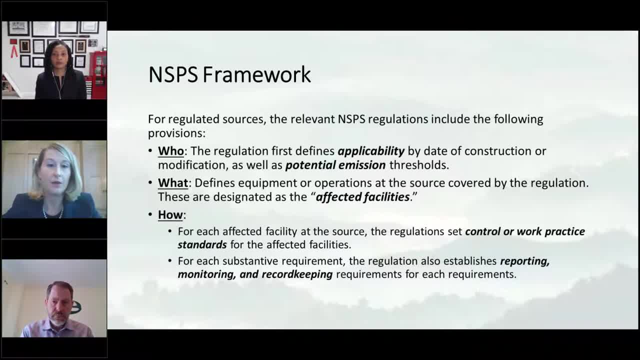 to route it to a control device and that has to have a certain percentage of efficiency, like 95 or 98 efficiency destruction for your emission. just one other beginner tip if you're starting to look at the nsps regulations and determine if it applies to your operations or facilities. 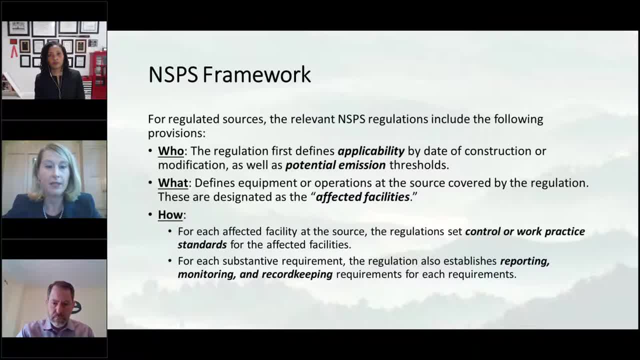 you also want to couple your review of the industry specific nsps with subpart a, that's a general section at the beginning of nsps. that will provide a lot of the basic requirements applicable to all the subsections and they should be read together. so, for example, subpart a will often supply reporting or testing obligations. 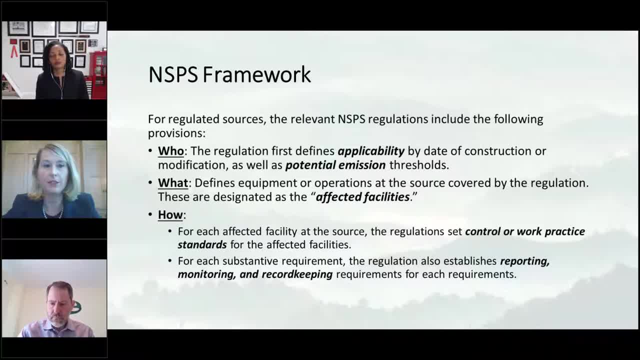 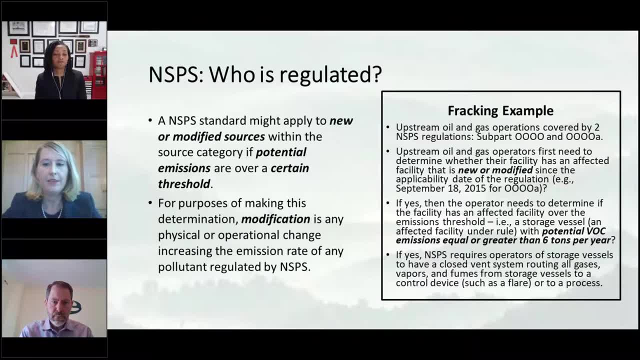 if those are not further specified within the individual nsps section. next slide, please. here i wanted to provide a specific example of how you'd go about determining if you have a regulated source. so first you check whether your industry or type of operation is covered by an nsps. 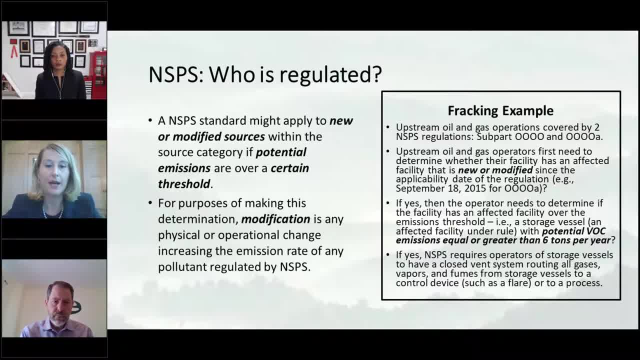 if you go to epa's website, so the example i had two slides back. they have great tables that show the impact of industry and operations and you can click on it and get the copy of the regulations. but another way to tell is to obtain the industrial code that covers the facility and to 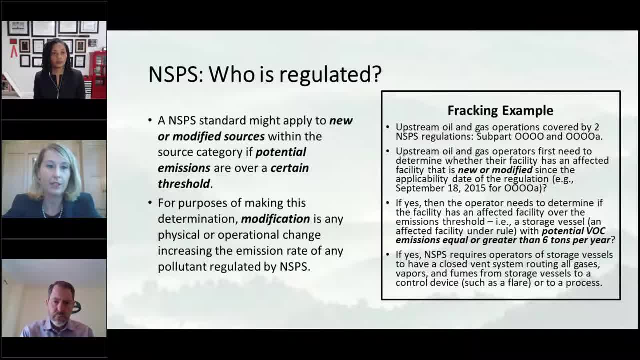 compare that to the applicability tables at the beginning of nsps regulation. if you have a match based on that, the rule will tell you what the effective facilities are within your operations or facility. so that's again the specific equipment or operations that will be covered. then you determine whether your effective facility was constructed or modified by the. 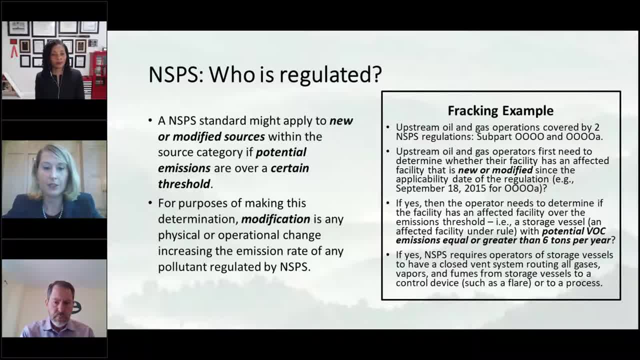 applicability date. that again will be set forth in the specific nsps issue. and then, finally, if you've said yes to all those questions so far, you'll need to determine whether the effective facility is potential to emit or over a threshold set in the rule. So 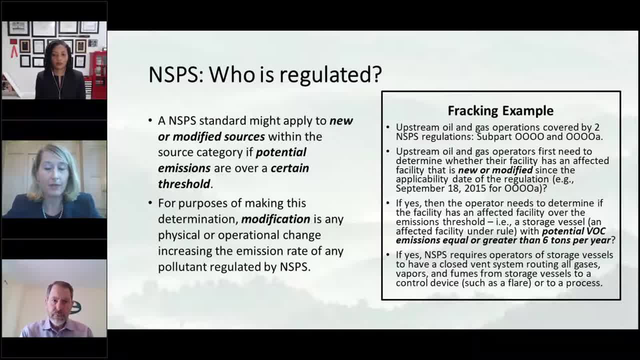 applying that to the example on the right, say you're working with a fracking company that's involved in upstream oil or natural gas production. That type of operation is governed by NSPS, Quad O or Quad OA. Looking at those regulations, the effective facility at the fracking site includes a number of things like: 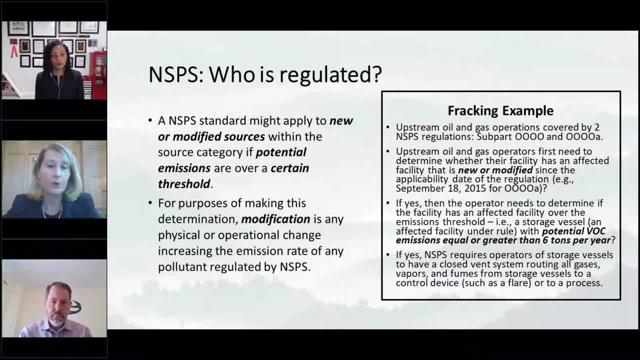 compressors and storage vessels. For purposes of this example, I picked storage vessels. The applicability date for Quad OA, which is the more recent NSPS regulation here, is September 18, 2015.. So you would take a look at your storage. 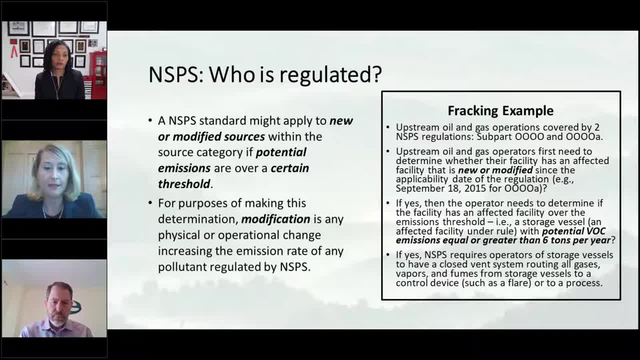 vessel, determine whether it had been constructed or modified after that date. If the answer is yes, then you need to determine whether it had the potential to emit over the threshold in the rule, which in this case is six tons per year of VAT. 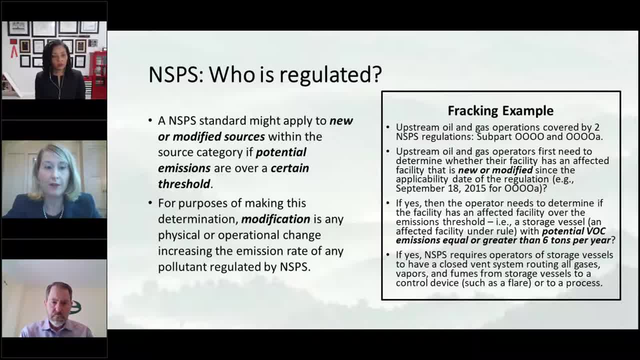 If you get to the end of that inquiry and you've determined it's applicable, then the rule will tell you that for storage vessels you need to route the emissions back into a process or to a combustion device that destroys the emissions to 95% rate. The rule will also tell you that there are a number of work. 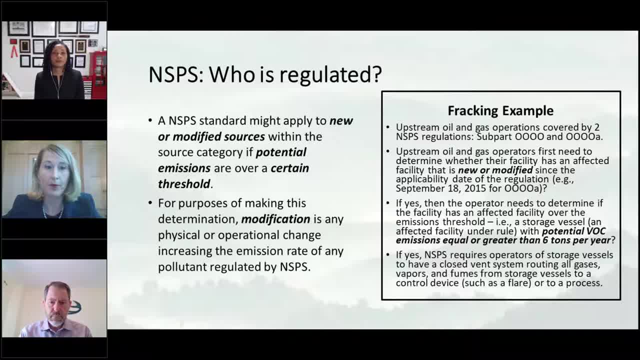 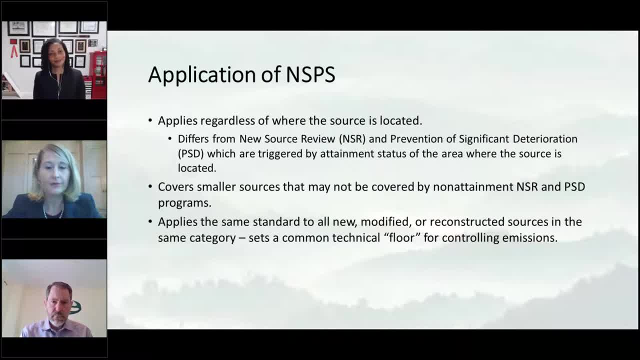 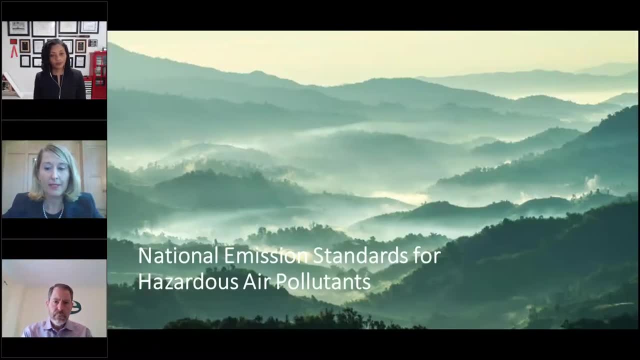 practice requirements and reporting requirements that apply at that point. Next slide: please A couple of broader points about NSPS before we move on to the next program, Unlike some of the other programs that I'm going to cover today and that Larry covered in the intro presentation- NSPS- 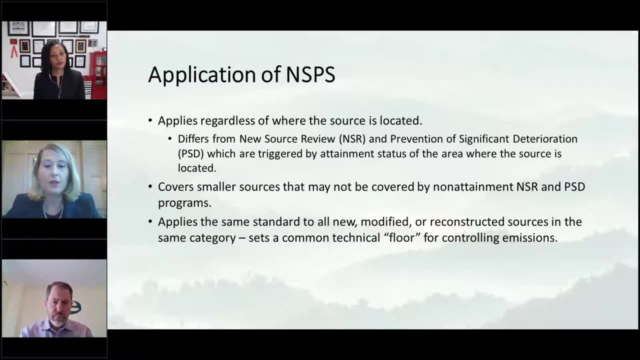 applies the same regardless of geographic location. So as Larry introduced the NSPS- sorry, the NSR- permitting program requirements vary based on whether the facility is in an attainment or non-attainment area, So NSPS doesn't work like that. it's uniform across the country, And so for that reason, we're going to talk a little more about that in our next webinar. 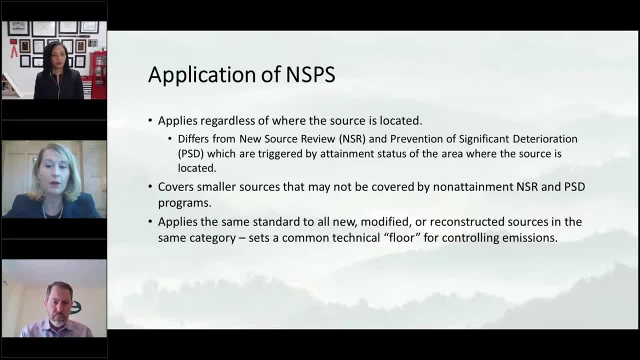 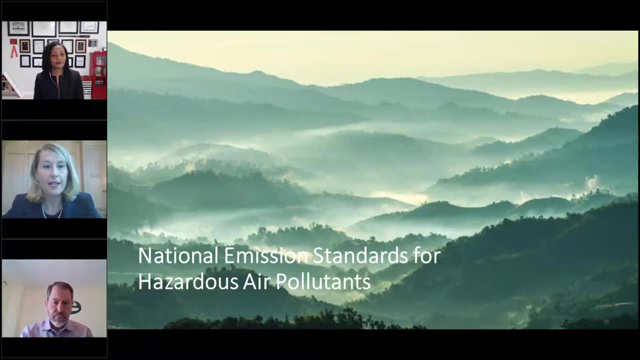 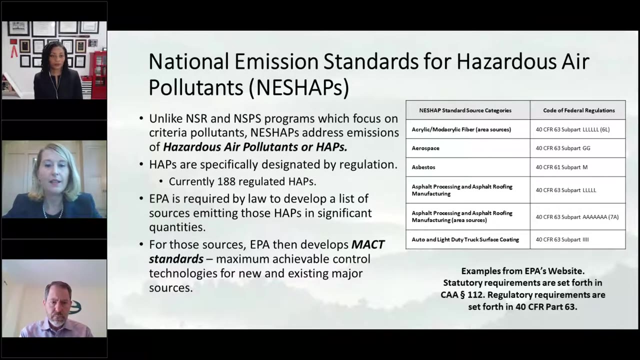 way to think about NSPS is that it creates a technical floor to ensure that similarly situated facilities are operating with comparable emissions and technology. Okay, next slide, please. So the next program I'm going to cover is the National Emission Standards for Hazardous Air Pollutants, or NSHAP, As Larry introduced, unlike the other two programs in 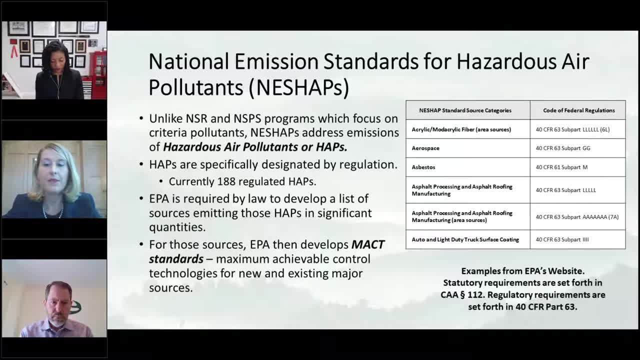 today's presentation. this program, NSHAP, covers hazardous air pollutants or air toxics, as opposed to criteria pollutants and their precursors. There are currently 188 regulated HAPs or hazardous air pollutants. Examples include benzene, toluene, xylene. EPA has a 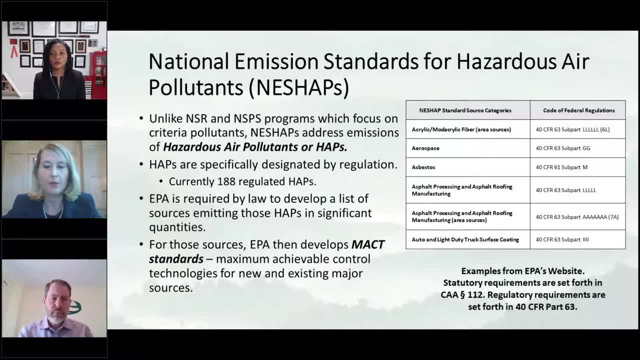 statutory obligation to set the NSHAP requirements for sources emitting HAPs, so that the NSHAPs are regulated by industry or type of operation. So, similar to what we just saw for NSPS, the NSHAPs are organized by industry or type of operation For those sources that are regulated. 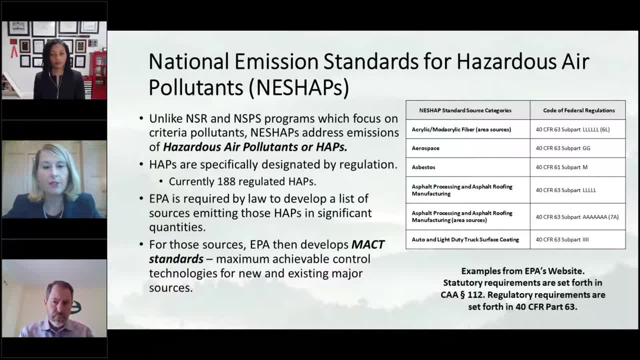 by a NSHAP, they must apply MAC or Maximum Achievable Control Technology to address the hazardous air emissions. MAC is such a key feature of this rule that sometimes NSHAPs are called MAC rules, and that's particularly true if you're referring to a specific subsection. So, for example, if you're referring to a specific subsection, if you're referring to a specific subsection. so, for example, if you're referring to a specific subsection. so, for example, if you're referring to a specific subsection. for example, if you're referring to a specific subsection. so, for example, if you're referring to a specific subsection. 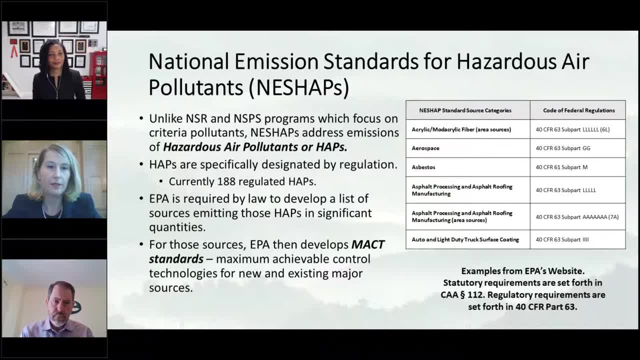 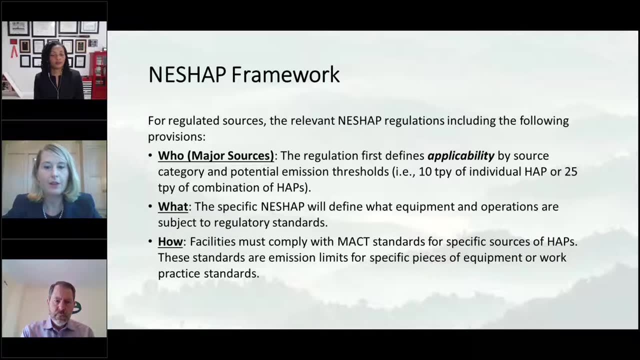 people would call the MON, which is one of the specific subparts, the MONMAC, as opposed to the MON-NHSHAP, or use those terms interchangeably. Next slide, please. Much like the NSPS example that I covered earlier. 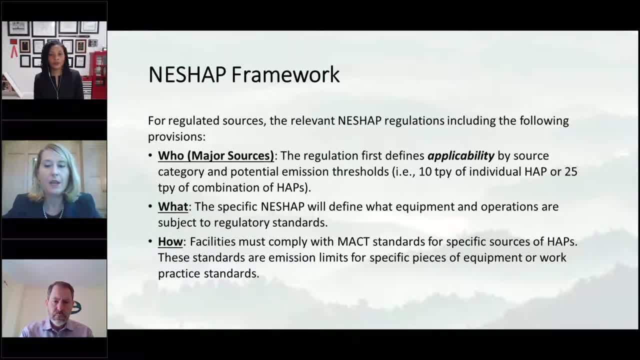 NSHAPs are fairly self-contained rules and they can tell you what sources are regulated, what equipment and operations are going to be subject to the standards under the rule and the standards for those regulated equipment and operations, what the relevant standard is and how to demonstrate compliance. 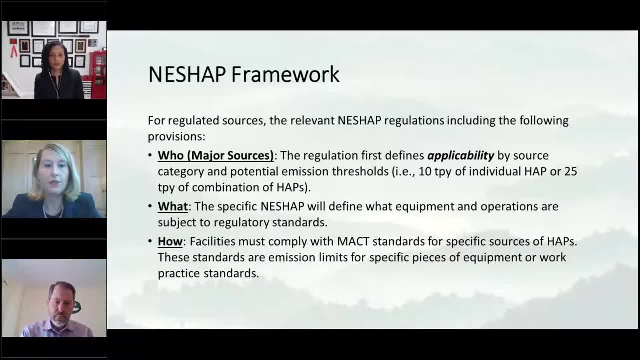 A little bit different from the NSPS. the NSHAPs do tend to divide equipment into different groupings. so, rather than having one standard that applies after you cross the threshold for applicability, sometimes NSHAPs will have various categories of regulation, but that's just. 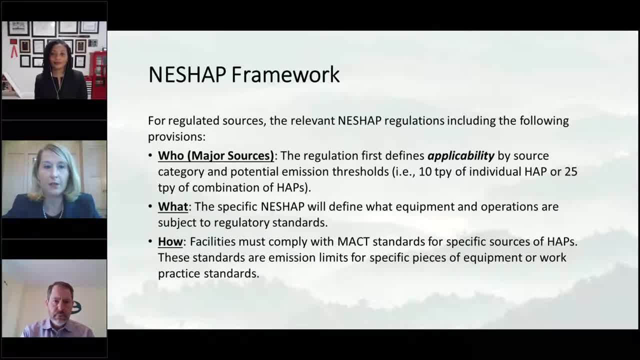 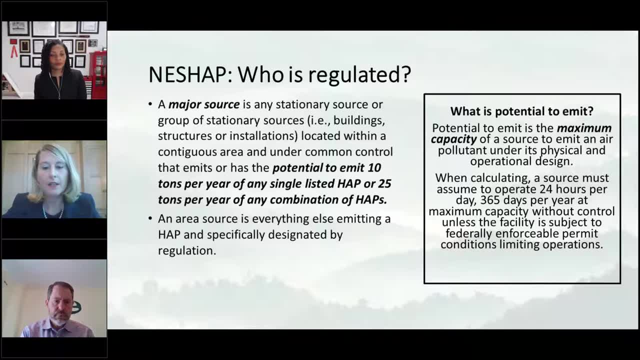 the general way. it works the same way as NSPS in terms of how the rules are organized. Next slide, please. All NSHAP standards, as Larry mentioned earlier, define major source applicability. the same way, A major source for purposes of a NSHAP is any stationary source or group of stationary sources. 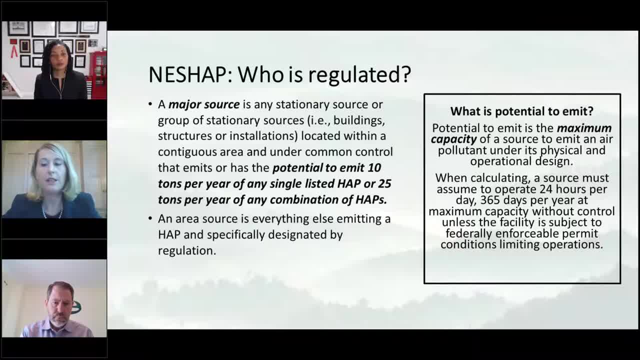 that emits, or has the potential to emit, 10 tons per year of any single listed HAB or 25 tons per year of any combination of HABs. So, for example, if I was working with a facility that had the potential to emit 11 tons of benzene, that is a potential major. 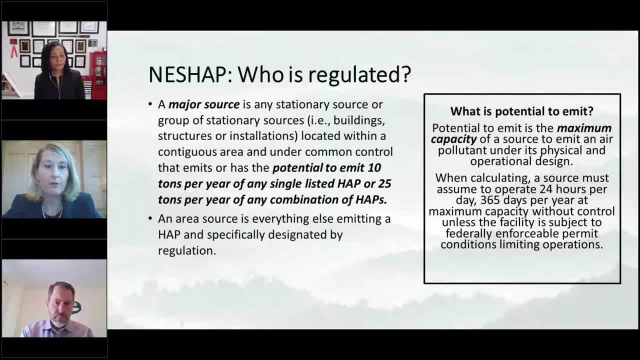 source for purposes of this program. You could also have a major source if your facility had a potential to emit 9 tons of benzene, 9 tons of toluene and 9 tons of xylene, because you would be adding them all together and you would be over the 25 ton per year. 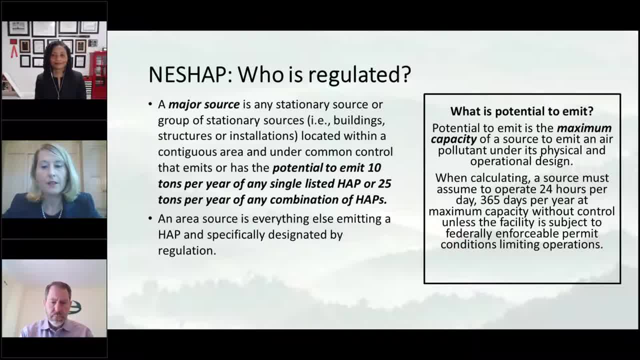 Then there's often- and I've mentioned this because I think it's an important part of the rule- to not overlook- the regulation goes on to talk about everything else, which are facilities that emit hazardous air pollutants that don't qualify as a major source under 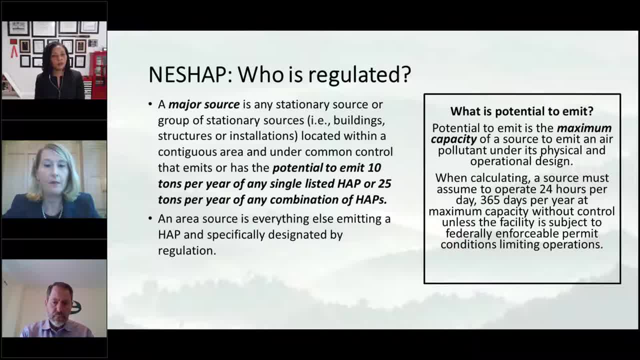 those PTE thresholds. Those are area sources and they have separate requirements that you should also evaluate when you're looking at the requirements for hazardous air pollutants. One thing that I've highlighted on this slide that's common to all the programs that we're: 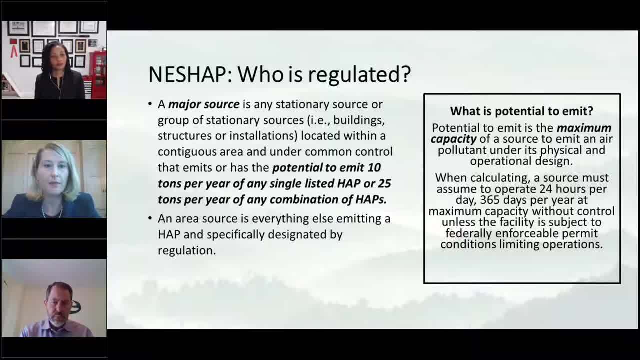 talking about today for stationary sources under the Clean Air Act is the concept of potential to emit is relevant for the applicability determination. The potential to emit is the maximum capacity of a source to emit an air pollutant under its physical and operational design. When you calculate the potential to emit, 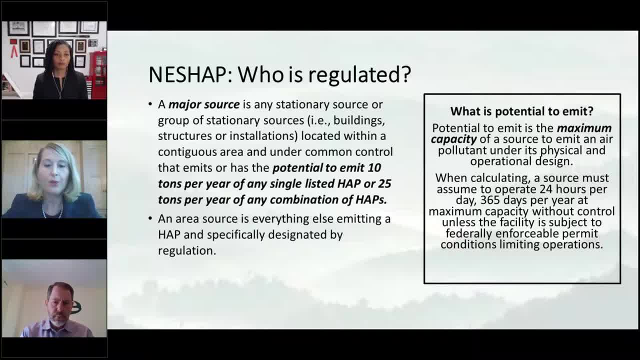 a source must assume to operate 24 hours a day, 365 days a year at maximum capacity, without control, unless the facility is subject to a federally enforceable state permit limit which addresses or limits operations. These permit conditions that you can consider in PTE or potential to emit calculations will: 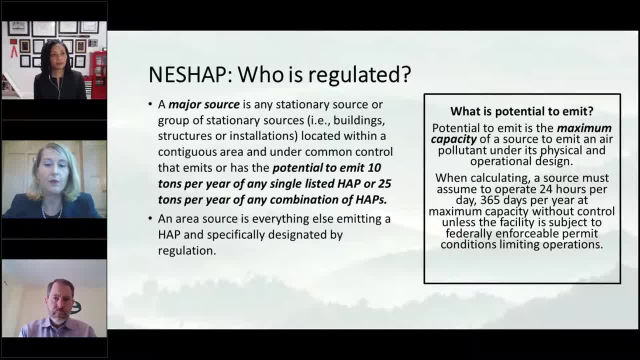 appear in state permits, but they must satisfy certain legal requirements before they become federally enforced. The PTE standard is a standard that is not a standard that is enforceable and therefore can be considered as limiting PTE. Next slide, please Okay. 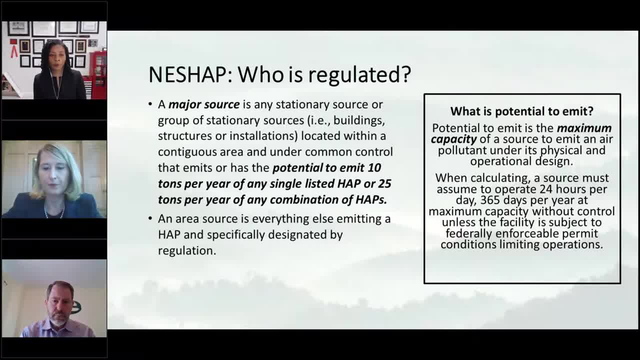 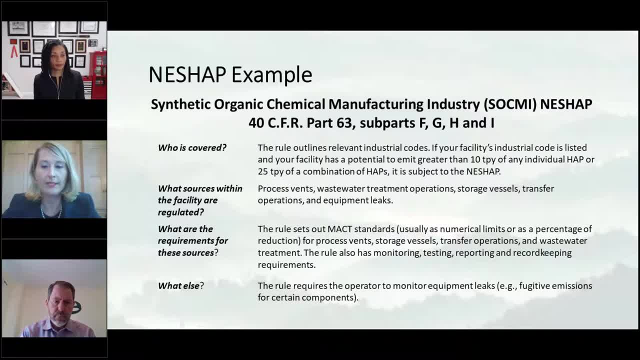 So, just like on the NSPS slide, I wanted to provide a practical example of what the MAC looks like or the NSHAPs look like in practice. So here I picked the NSHAP standard that governs the chemical manufacturing industry. It's called the SOCNIMAC. And you can see here how the NSHAP standard is based on the NSHAP standard that is used for the chemical manufacturing industry. And you can see here how the NSHAP standard is based on the NSHAP standard that is used for the chemical manufacturing industry. 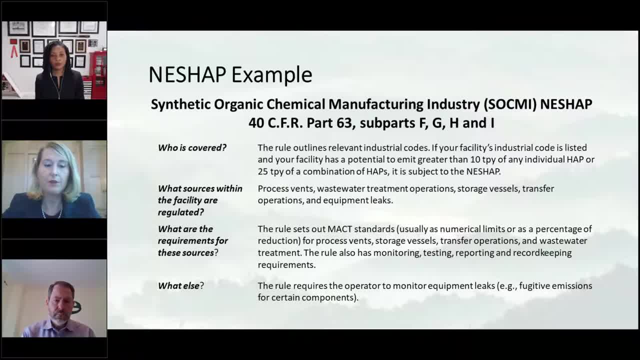 So this is where the rule defines who is covered. You first look to see if you meet any of the potential to emit thresholds. if you have the industrial code, that would be all under this particular regulation, Then under this particular NSHAP, the regulated sources are the process vents that are actually 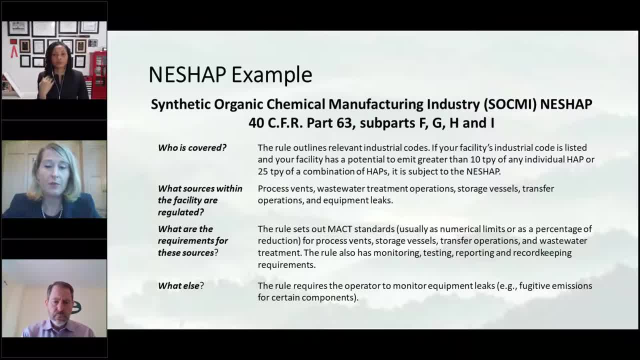 used in chemical manufacturing, along with the facility's wastewater storage tank and equipment leaks, And so, within the rule, you determine your – which of these types of equipment are used in chemical manufacturing, along with the facility's wastewater storage tank and equipment leaks. 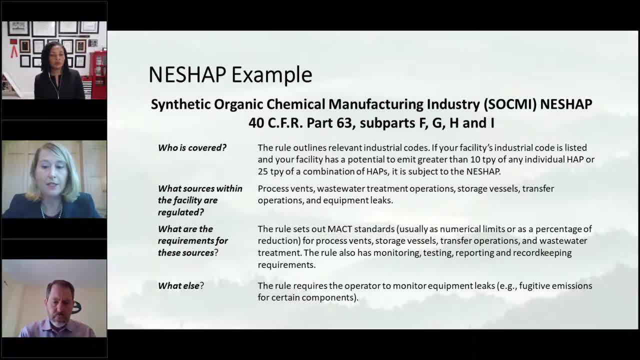 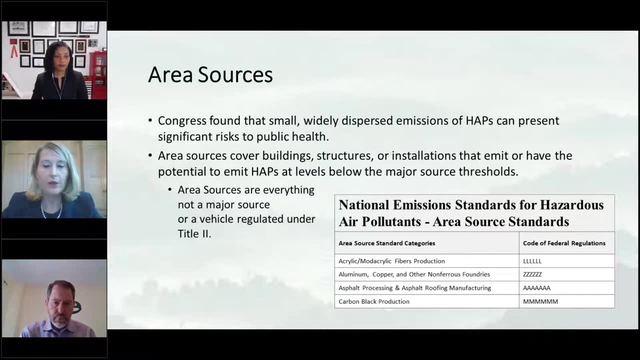 And the rule will tell you for each of them what the relevant standard is for control and how you demonstrate compliance, including monitoring and reporting. Next slide, please. Finally, as I alluded to earlier, the NSHAP standards also address sources that emit HATs. 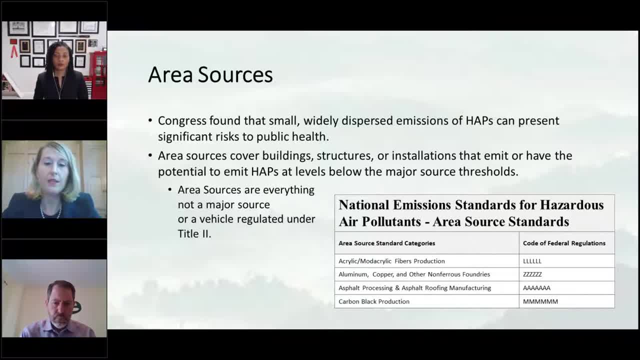 that fall below the PTE or the potential to emit thresholds, and these are called area sources. Finally, as I alluded to earlier, the NSHAP standards also address sources that emit HATs but fall below the PTE or the potential to emit thresholds, and these are called area sources. Finally, as I alluded to earlier, the NSHAP standards also address sources that emit HATs but fall below the PTE or the potential to emit thresholds, and these are called area sources. Finally, as I alluded to earlier, the NSHAP standards also address sources that emit HATs but fall below the PTE or the potential to emit thresholds, and these are called area sources. 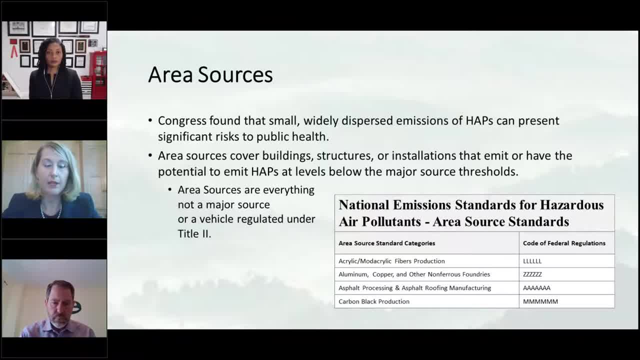 Area sources are organized in a similar manner to the NSHAP, but they're less onerous because the MAC standard doesn't have to apply. in terms of the relevant control technology and the limits, The key point here is just to remember to check for area source requirements if you're evaluating. 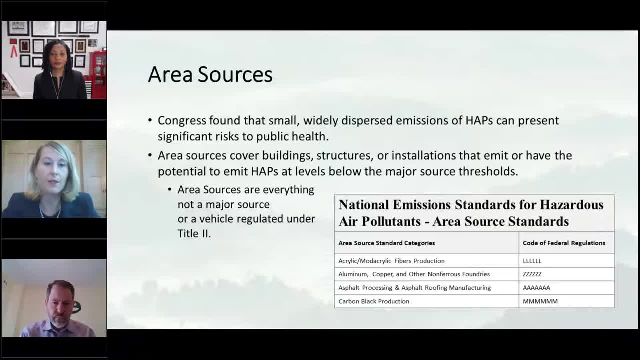 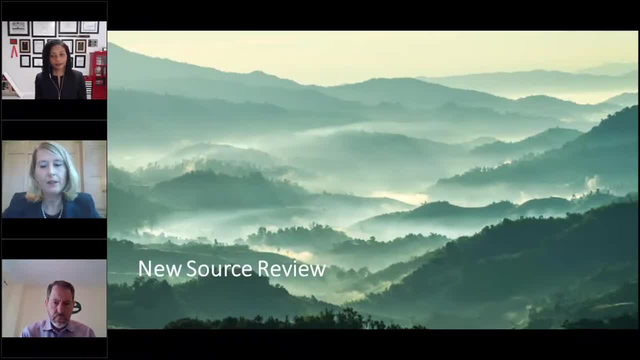 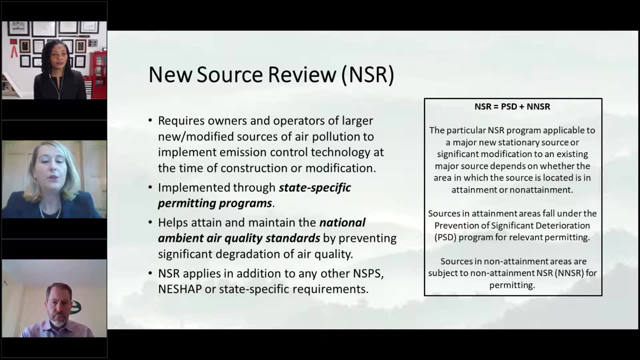 the potential regulatory requirements for a source, even if it doesn't qualify as a major source. Next slide, please. Finally, I will cover new source review. Next slide, please. New source review requires owners and operators of new and modified sources to obtain permits. 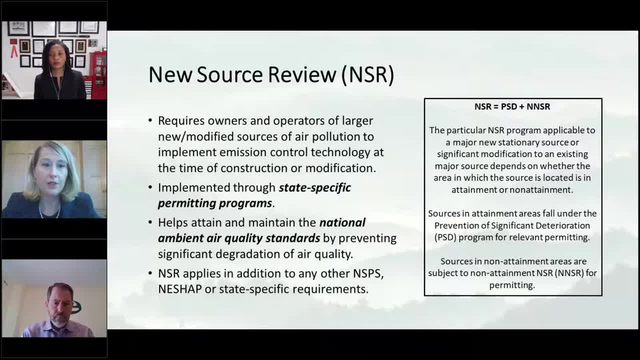 with appropriate limits and control technology prior to new construction or modifications. The purpose of this program is to maintain the NACs, or the National Ambient Air Quality Standards that Larry discussed earlier. NSR is implemented through a state-specific permit program, So similar this program, but also the other two I've been talking about, are generally. 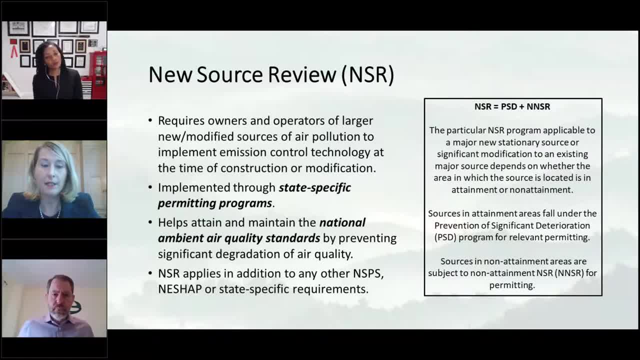 outlined at the federal level but incorporated into state SIPs, the state implementation plans that Larry talked about earlier. so you have to check both sources, And so here the important part is that NSR is a state-specific permitting program, so you need to check there in the first instance to determine the relevant requirements. 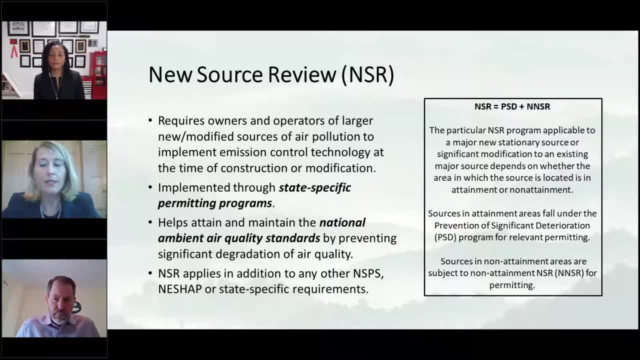 And in that regard NSR is somewhat customized because it's implemented through a permit program. Next slide, please. The program is implemented through a permit that will apply to that specific facility in general, as opposed to the other programs where the rule will tell you what is the numerical. 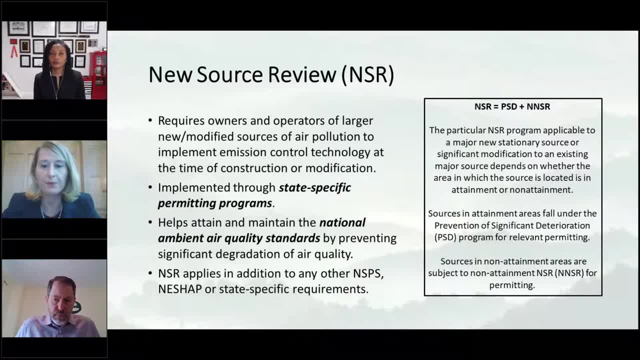 emissions limit, no control technology that you need to use. Another key element of the NSR program is that it can vary based on the area that you're operating or constructing or modifying a source, And here this is again. the distinction that Larry talked about earlier is the difference. 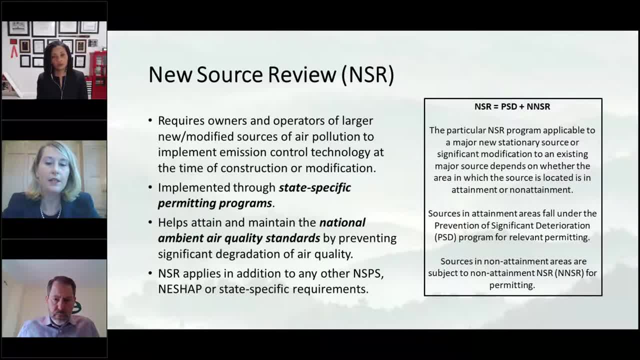 between attainment and non-attainment areas. Next slide, please. Sources that are in attainment for the NACs can secure state permits for construction and modification under the PSD the Prevention of Significant Deterioration Program. Sources that are operating or will operate in non-attainment areas for the NACs. 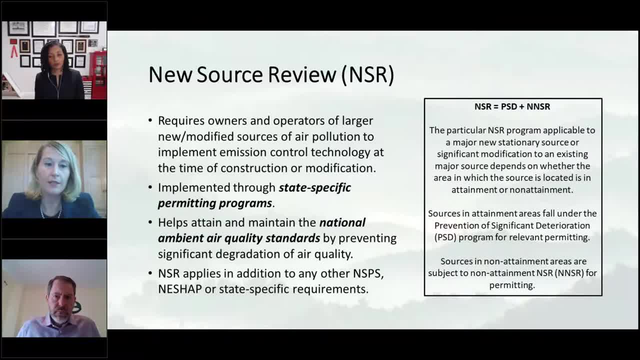 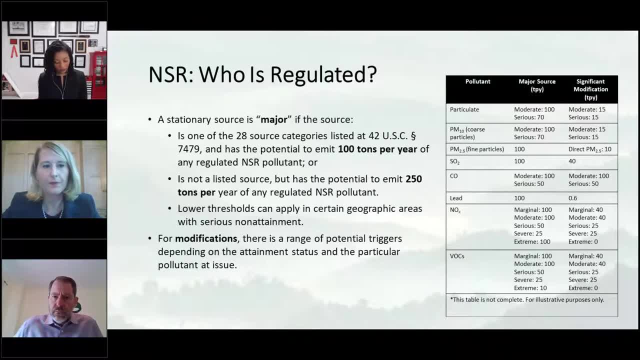 will need to secure non-attainment NSR permits from their relevant state and local permitting authorities. Next slide, please. The applicability of the NSR program, and specifically whether the facility will need a permit for construction or modifications, turns on potential to emit much like the other programs. 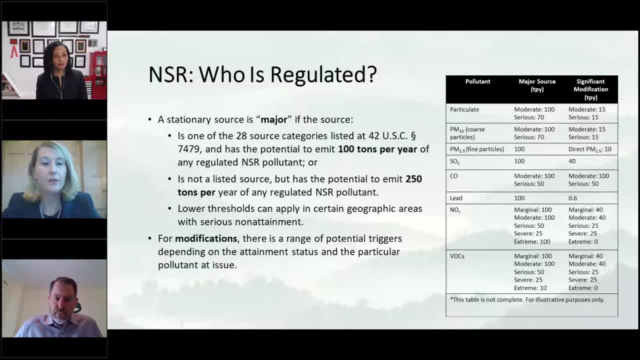 that I reviewed today, But the thresholds vary so it's a little bit more complex to determine whether you need a pre-construction permit under this program For new construction. the Clean Air Act has a list of 28 sources and these are broad categories. And for those 28 source categories identified by the Clean Air Act, the potential to emit standard is 100 tons per year of any regulated NSR pollutant. If your source is not listed in the Clean Air Act, then the trigger is 250 tons per year. 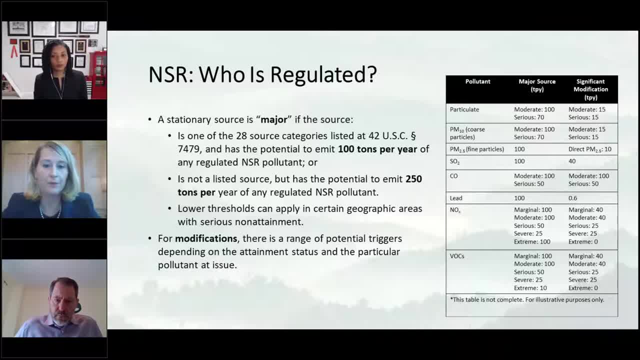 PTE or potential to emit for an NSR pollutant. For modifications, the potential to emit threshold is a little bit more tricky. The table to the right sort of demonstrates that the potential to emit threshold is a little bit more tricky. The table to the right sort of. 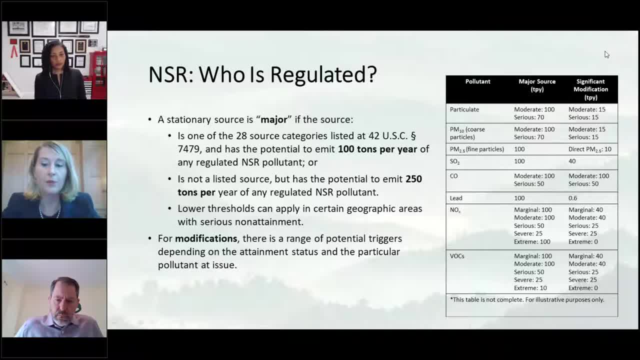 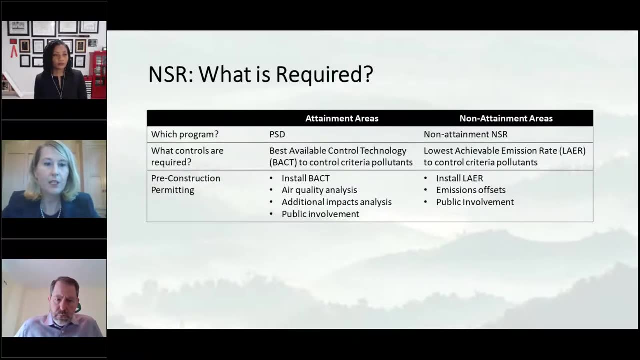 demonstrates the variety, but generally, the thresholds for modifications will depend on the specific pollutant, as well as the area where the facility is located and its attainment status. Next slide, please. So, as I mentioned earlier, the requirements for NSRPSD permitting. 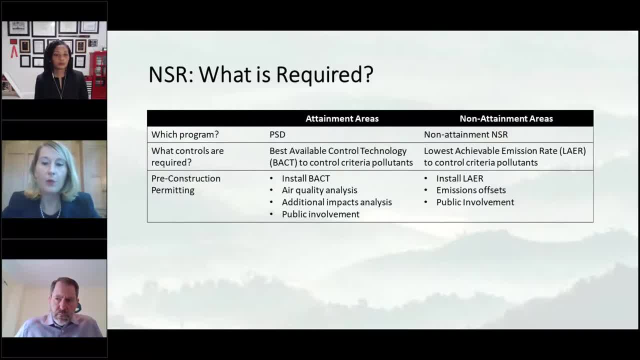 are outlined at a high level in federal regulations, but there are more specific details in the state implementation plan, So it's very important to consult with the state regulations for this and all the programs that we discussed today. in general, for sources in attainment area who are going undergoing psd, they must secure a 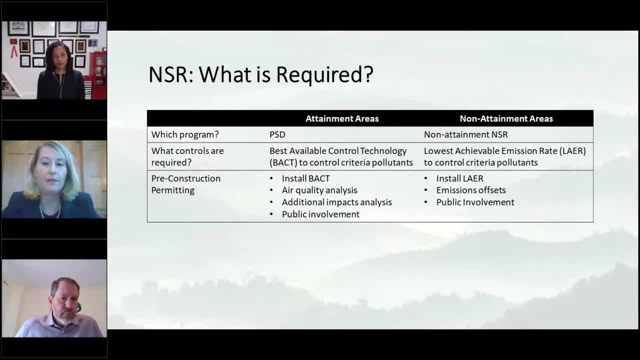 pre-construction permit for the proposed project that will utilize best available control technology or back for its emission units. the rule also requires psd sources to conduct air quality analysis to ensure that they won't increase emissions in a way that will impact air quality, and the permitting process under psd is subject to a public 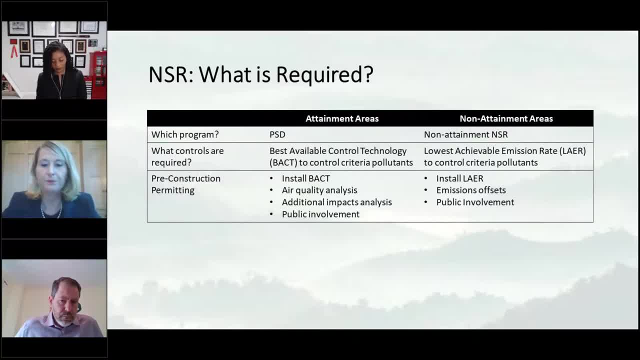 public involvement, public comment and hearing process for sources that are in a non-attainment area. they also will secure a pre-construction permit from their state or local government, but it will undergo a more rigorous process because they're in non-attainment. the area is in. 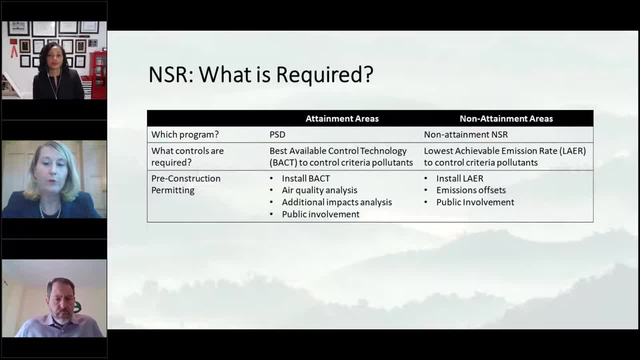 non-attainment. the state permitting agency will be evaluating the facility's proposed construction or modification for compliance with technology that can achieve the lowest achievable emission rate, so a very stringent standard. the facility also, as larry alluded to, must obtain emission offsets from other sources or within their own fence line. 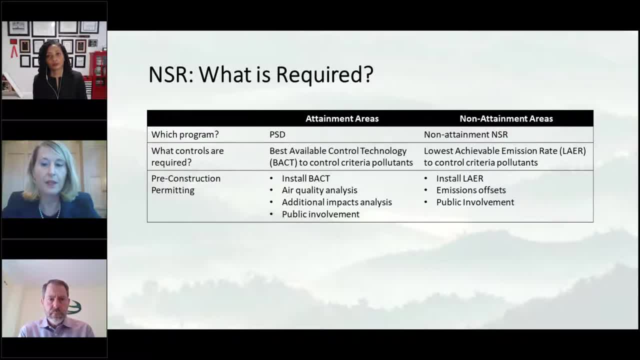 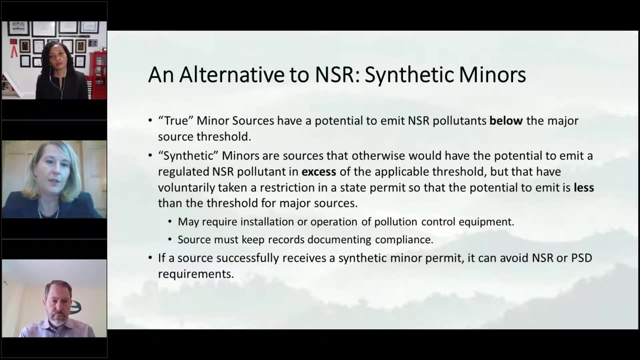 to make sure that there's no increase in emissions as a result of the project and, like psd, this permitting process is a public process that involves a public comment and potentially a hearing. next slide, please. finally, i wanted to close out this discussion with nsr with a comment about. 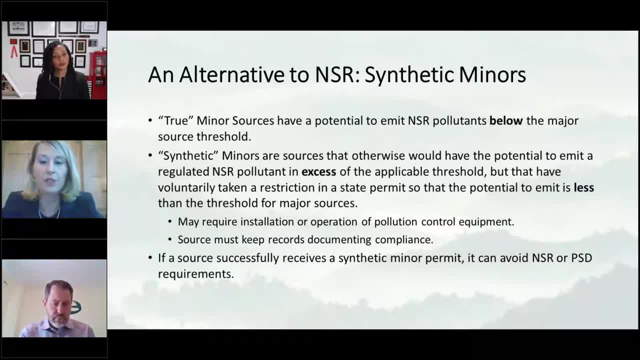 a very common alternative that a lot of sources use, which is to become a synthetic miner. as you can probably infer from this presentation, the nsr permitting process is very onerous and it takes a lot of time and resources for both the state agency as well as the source. 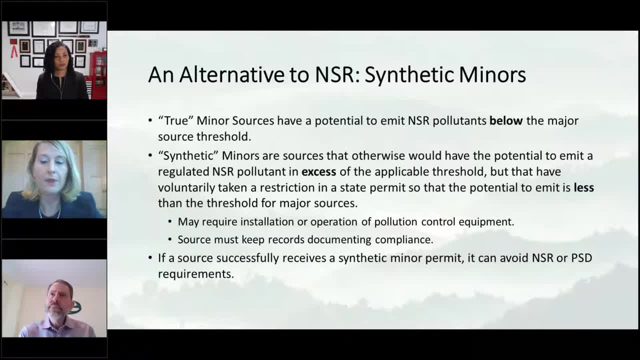 so to achieve similar air quality objectives, many sources who have a potential to emit a regulated pollutant above the emissions thresholds in the statute will voluntarily take restrictions on their operations in a state permit that the epa can enforce, thereby limiting their potential emit and also taking them outside of the definition of a major 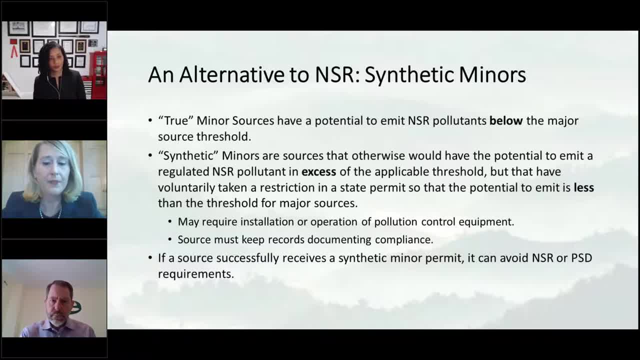 source. this is called a synthetic miner and it's an option available, i believe, in almost every state agency in the state. this could require the source to install a control equipment, um and to have permit limits that might not that regulate the operation controls it could can involve them. 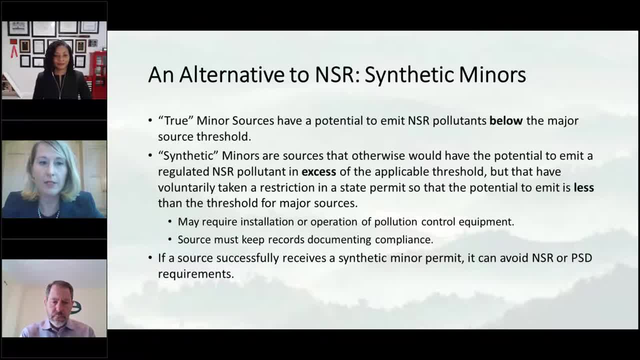 taking operational limits. there are a number of record keeping and reporting requirements associated with this approach. so it's it's definitely a um, an approach that is protective and can obtain many of the benefits of psd permitting, but it does kind of um create a more um streamlined process for permitting in an option that many sources will elect to do. 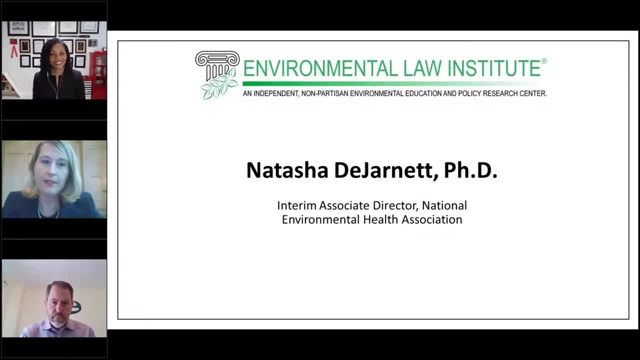 so that is my overview of nsps, nishaps and the new source review program. thanks so much. thank you so much, stacy. we'll now turn to natasha. well, thank you very much. um, it was wonderful to learn from stacy and larry. i also want to. 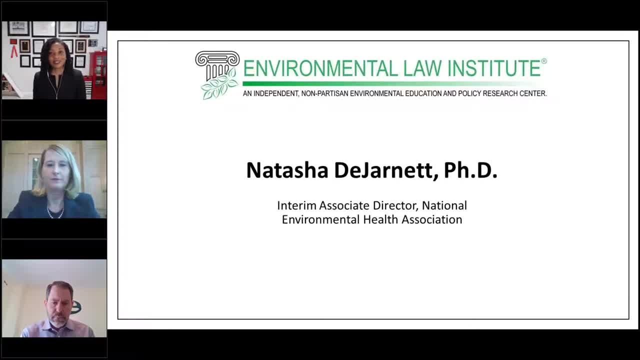 thank you, caitlyn, as well as the environmental law department and the nsr permitting committee and the environmental law institute and the organizers for the kind invitation um so honored for this opportunity to speak to the amazing group. i also want to take some time to acknowledge um any frontline workers that are working to prevent or mitigate the spread of covid. 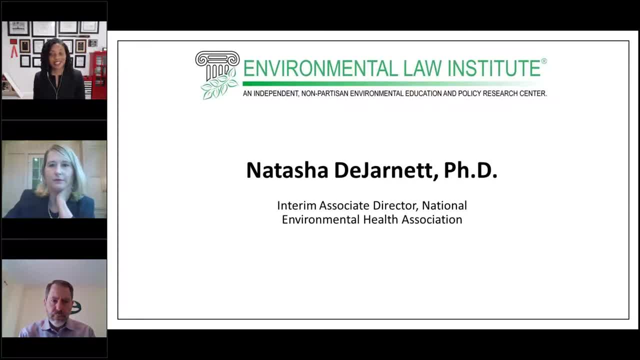 as well as the essential workers who put their selves at risk throughout this pandemic, to meet everyone's needs. in addition, i want to acknowledge those that are in the global movement to call for justice and equity. um, i want to acknowledge those that are in the global movement to call for justice and equity. 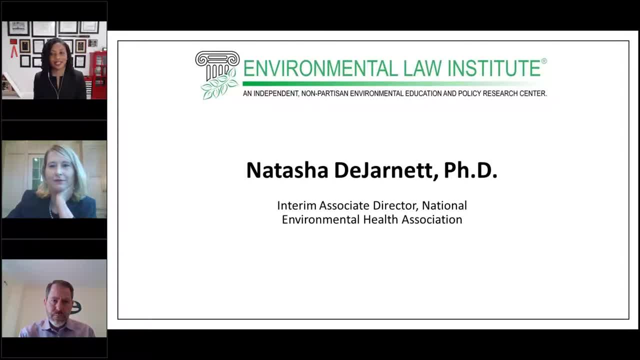 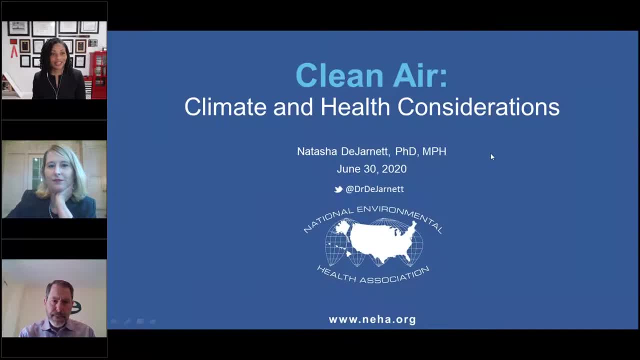 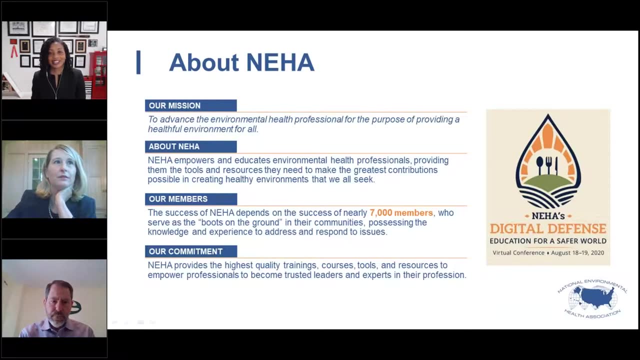 for all those reasons, i am not taking for granted this amazing opportunity, uh to speak with you today. so today i will be sharing about uh- clean air under the auspices of climate and health consideration. so, before i step into the many ways that climate change harms health, i'd like to share. 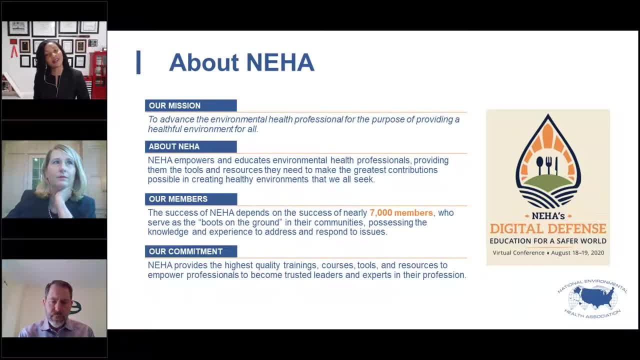 with you just a little bit about the national environmental health association, also known as niha, environmental health professional, with the purpose of providing healthful environments for all. environmental health professionals actually make up the second largest segment of the public health workforce, ensuring, in particular, that we have clean air to breathe as well as safe water to 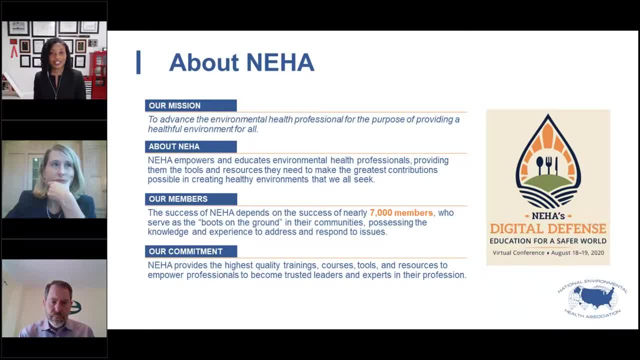 drink safe food to eat and are in environments that are free of disease carrying vectors and public health pests. niha has nearly 7 000 members, and our members are predominantly working in the public sector, um in all levels of government, including federal, state and local, as well as all seven uniformed services, as well as folks that 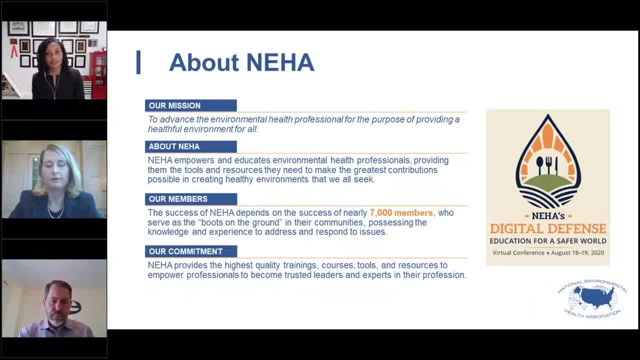 work in academia as well as industry. we have a long and successful history providing education and training, as well as being a resource within the environmental health community. our members work in many areas that are both directly and indirectly related to climate change, which i will give you some examples. uh, as this can, as we proceed. uh, first, i also want to 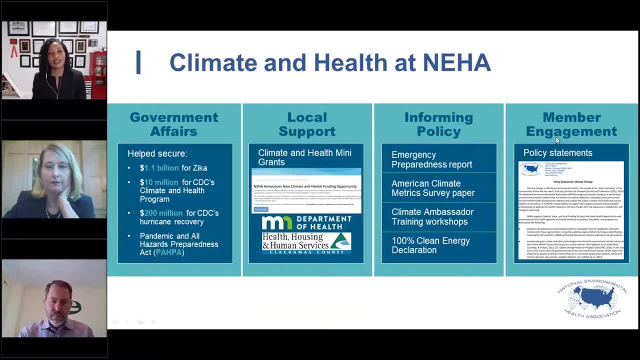 to give you a snapshot of climate and health at niha government affairs. at niha, advocates on behalf of the environmental health workforce. our solution to environmental challenges like climate change is to invest in credentialed environmental health professionals in the workforce. as such, we have. 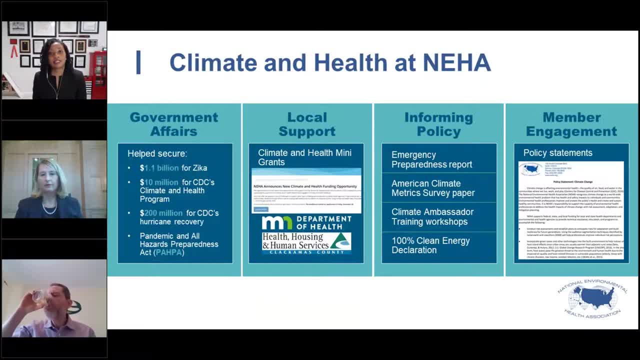 helped secure funding for zika, for cdc's climate and health program and for recovery from the 2017 storms uh, where we had three storms, uh all, or three major storms all make landfall in the us. in addition, we work to ensure that the voice and expertise of environmental health professionals 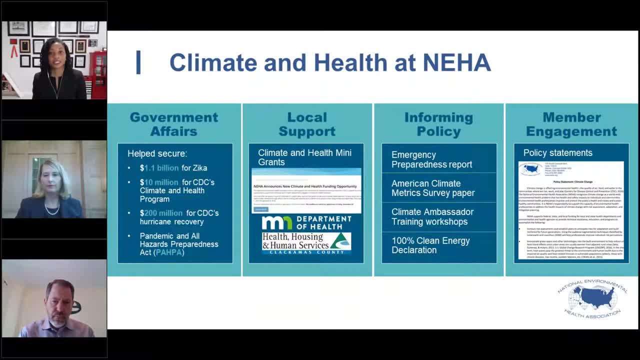 was reflected in the pandemic and all hazards preparedness act which was signed into law last year. this was environmental health professionals at the table to ensure that every community is prepared for environmental health hazards in the event of natural disasters, which, unfortunately, are becoming all too common with climate change. 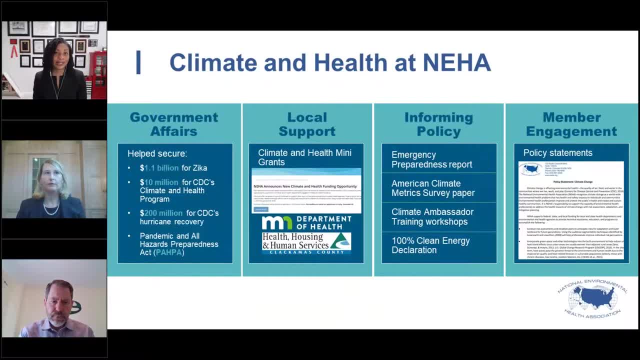 with funds from cdc, we've provided support for climate and health adaptation activities for the minnesota department of health and a tri-county region in the portland oregon area. in addition, this year we plan on funding two additional health departments that are approaching climate and health adaptation from a health and all policies framework. 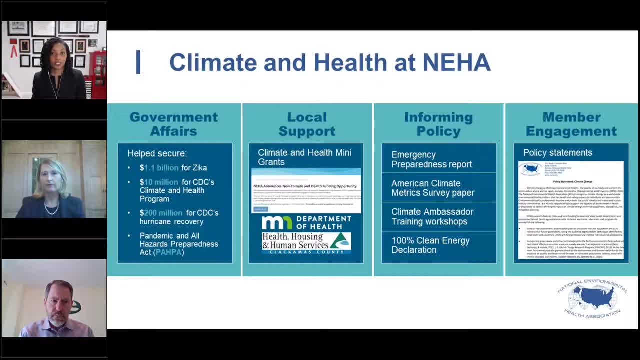 with funding from eco america. this has allowed us to do much work to inform policy, so we have developed a report on climate change and emergency preparedness that explores the environmental health workforce role. in addition, with eco america, we've published three years of the american climate metrics survey. 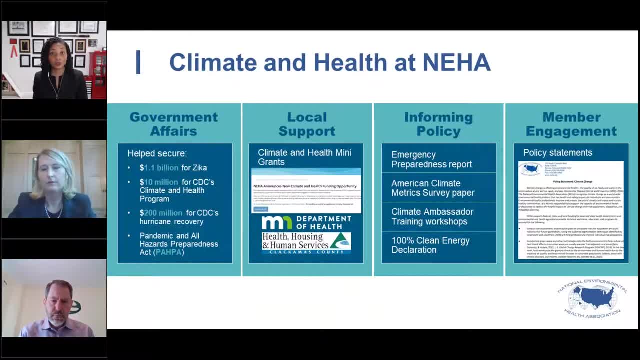 which was conducted on our membership over multiple years. in addition, eco america has hosted a climate and health ambassador training during niha's annual educational conference for the last two years and i'm really excited to share with you that niha's board unanimously declared that by 2030. 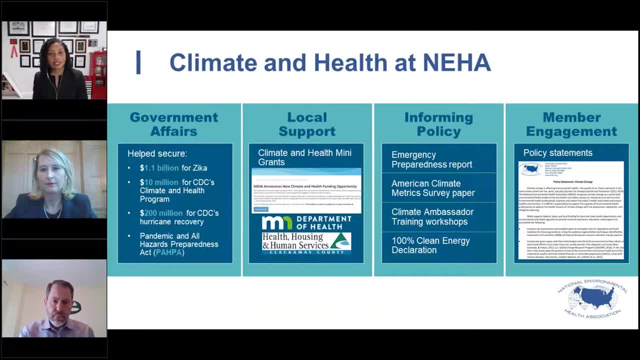 2030, NEHA will be 100 percent clean energy. Lastly, our members are very engaged in climate and health. We have a climate and health program committee and they spearhead the development of policy statements. We have a statement on climate change that sunset in February. 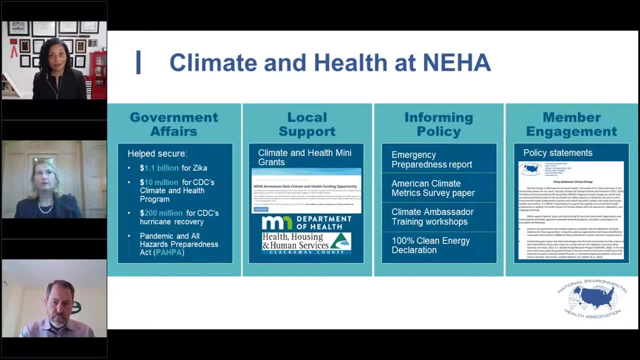 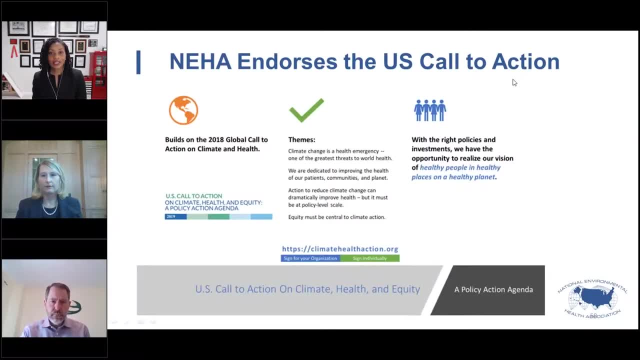 of this year. We have submitted an update to this statement to our board and we'll find out mid-July if this is accepted. In addition, I wanted to share with you that NEHA endorses the US Call to Action on climate, health and equity policy Agenda. 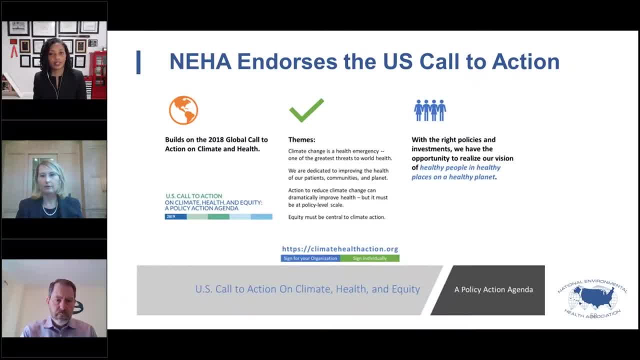 This builds on the 2018 Call to Action on climate and health Ng. new Call to Action. among the themes include that equity must be central to climate action, So I encourage anyone that is interested in learning more, more or signing up for their organization. 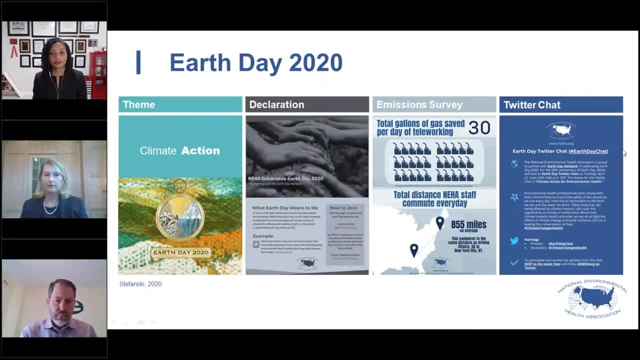 or for themselves to visit climate actonorg. This year we celebrated the 50th anniversary ofIZ%i estar bien en tu estado participando en el processo de la agenda de Integración culturesquítica. anniversary of Earth Day. I'm really proud to share that Environmental Law Institute. 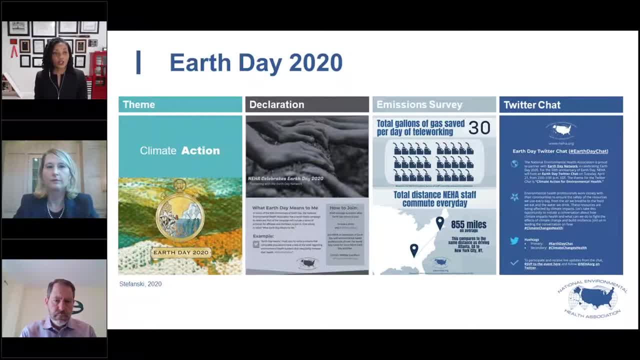 was a partner. As such, part of our Earth Day activities and our staff were to complete an emissions survey. Now this took on a different scent because we've been teleworking since mid-March, but we had the original intent to have a one-day universal telework for our 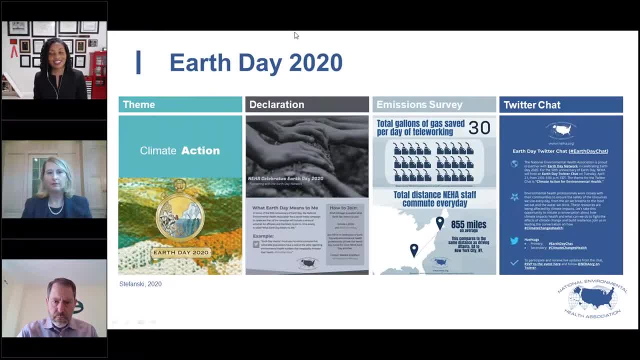 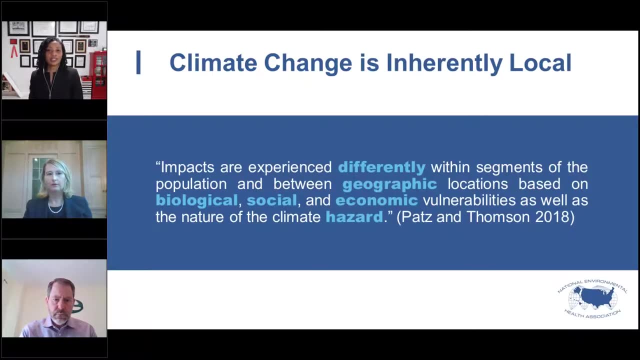 staff. We completed the survey under those auspices. We're going to publish those results in the Journal of Environmental Health very soon. Our Executive Director, Dr Dave Dijak, frequently describes environmental health as being inherently local. The same can be said of climate change. The impacts are experienced differently and 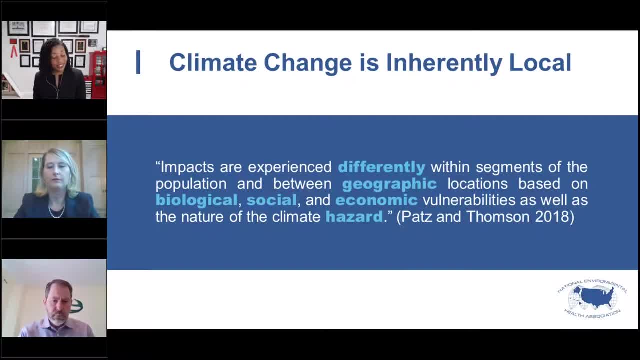 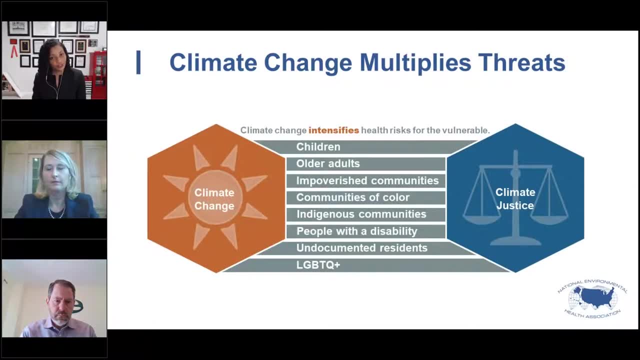 they can be within different segments of the population, by geography and even by neighborhood. Today, I want to help paint a human face on climate change. As we get into the different ways that climate change impacts health, with special focus around air quality, I wanted to share with you some of the populations that are most susceptible. First and foremost, 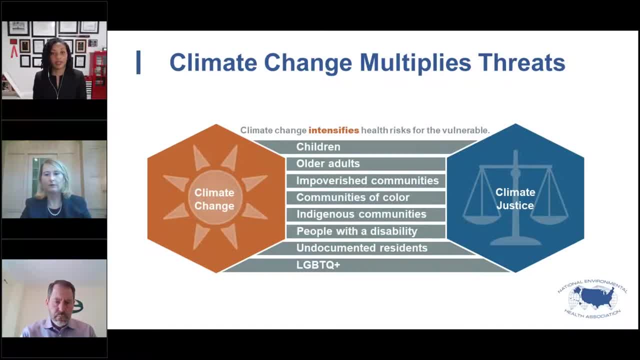 we are all at risk to the health threats of climate change. These health threats are vast, but there are some groups that are more vulnerable to these health threats. Climate change is actually a threat multiplier for them, exacerbating some inequities that some of these groups may already exist. For children, I'm going 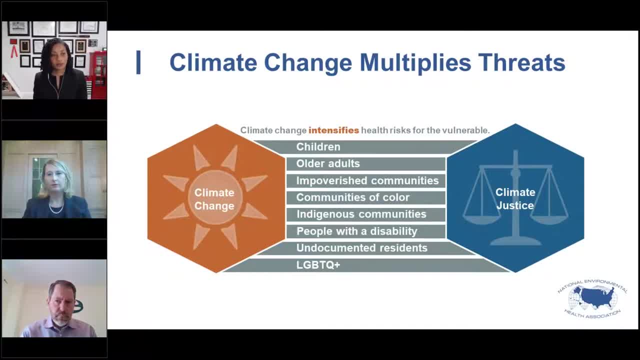 to come back to them later with a bit of additional evidence. We'll start with older adults. Older adults are more likely to have pre-existing illnesses that may make them more susceptible. In addition, older adults are more likely to be socially vulnerable. They may not receive the air quality alerts or they may not receive the extreme heat alert. 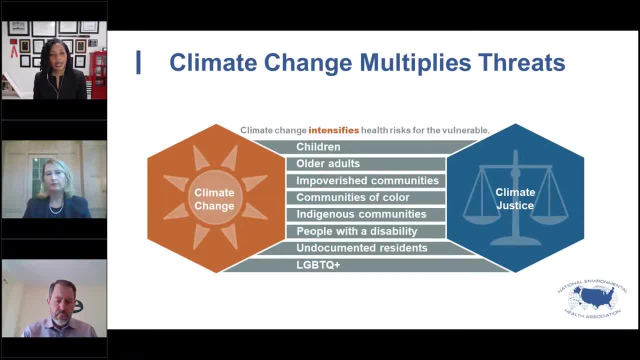 or calls for evacuations. This makes them far more susceptible when it comes to climate change events. We have impoverished communities and communities of color all across the US that are also at higher risk, because these communities are more likely to live on the fence lines of industrial polluters, meaning that they bear a higher burden on the environment. 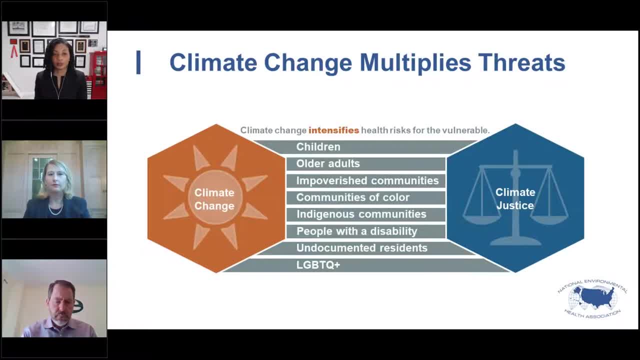 So we're going to talk a little bit more about that in just a moment. In addition, we have indigenous communities. like many other communities in the US have really strong ties to the land. These ties can be very strong cultural ties very strong. 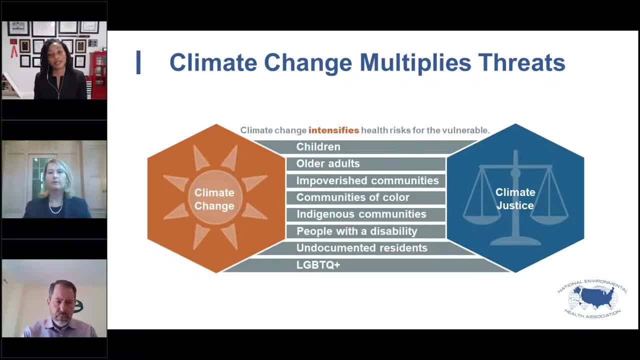 religious ties. Climate change is changing the land around them and even displacing some of our indigenous communities, leaving them, leaving their threats, multiplied. when it comes to climate change, We have people with a disability who may not be able to relocate as easily or as quickly. 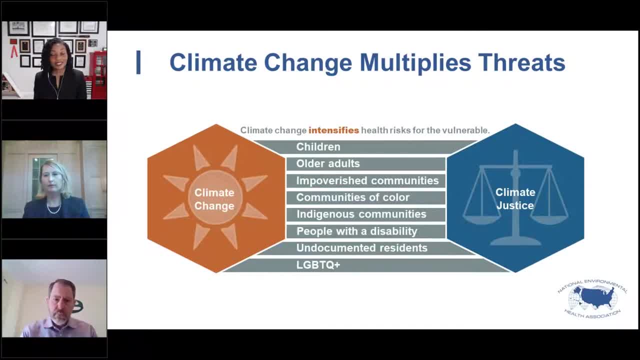 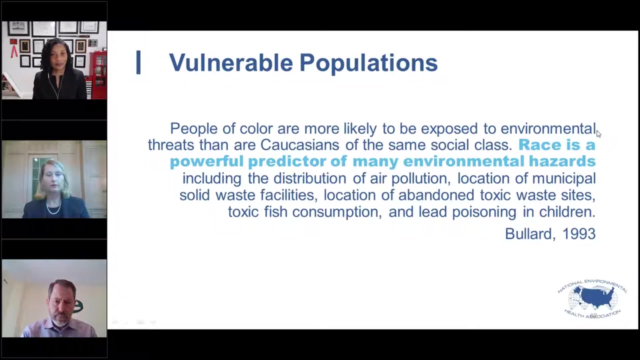 We have undocumented residents that may not feel comfortable in going to shelters when it's time to evacuate for fear of deportation. And then we have LGBTQ populations, who have expressed concerns also with storm shelters for fear of discrimination or worse. So, as we consider climate action, 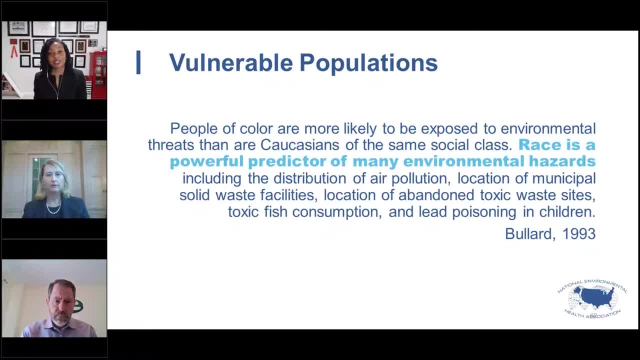 as we look to air quality, we must know that justice needs to be at the center of climate action, or else, even with the best of intentions, there are gonna be some groups that are going to be left behind. So I just wanted to add a little bit further evidence. 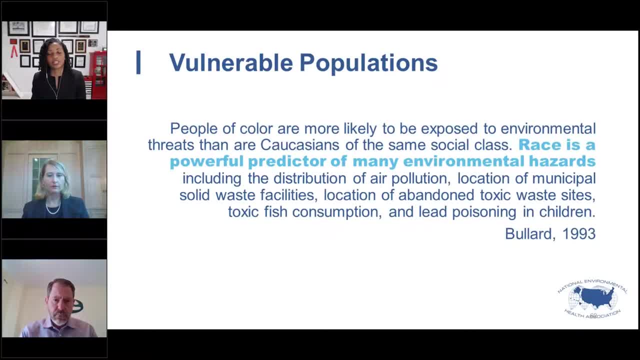 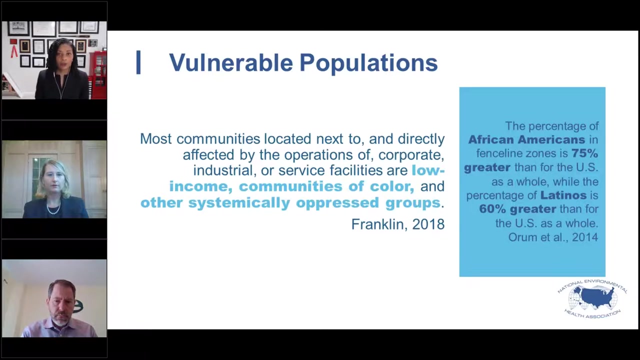 as a quote from Dr Robert Bullard, who is the father of environmental justice, and what he shared in 1993 has been reassessed and validated multiple times since then. that race is the most powerful predictor of where environmental hazards are located. In addition, low populations or communities, 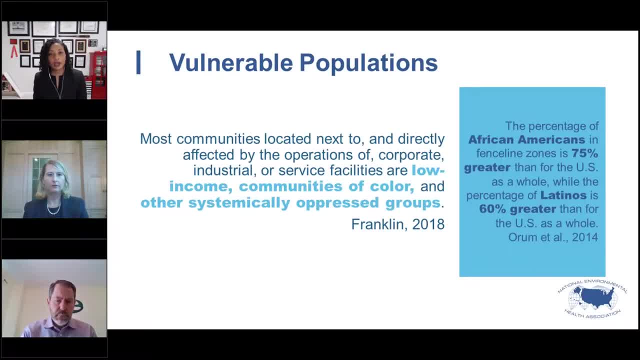 that are low income, communities of color and other systematically oppressed groups are more likely to live next to industrial facilities or industrial polluters, And then the percentage of people that are living in these fence line zones is 75% greater and Latinx populations is 60% greater. 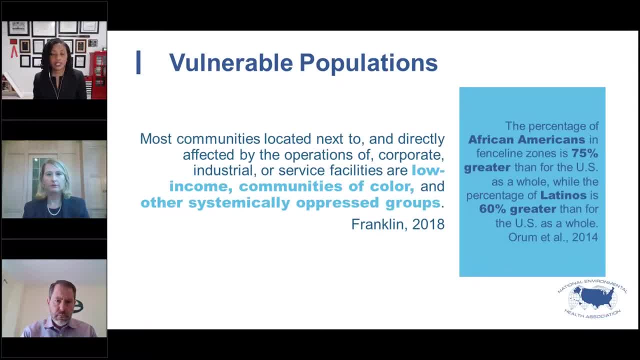 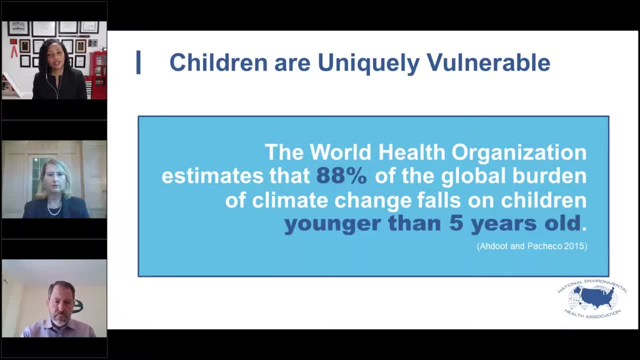 than when compared to the rest of the US for living in these fence line zones. So these are some key vulnerable populations I wanted to make sure we keep in mind as we discuss clean air, as well as climate and health. In addition, I wanted to share with you 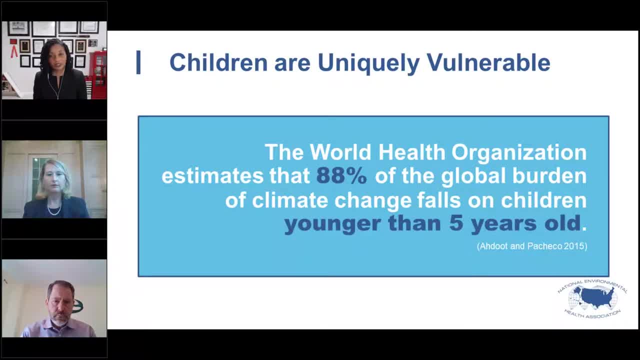 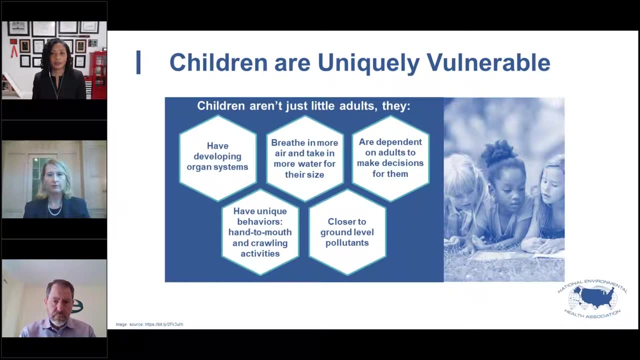 about the unique vulnerability of children. I think this particular statistic that's shared is heartbreaking. The World Health Organization estimates that 88% of the global burden of climate change falls on children younger than five years old, So children disproportionately suffer from the health impacts of climate change. 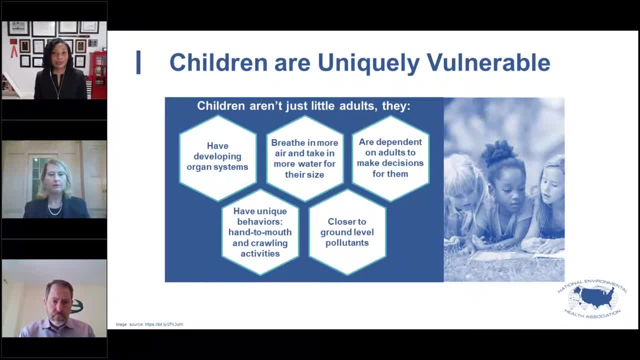 And it's for multiple reasons. Children aren't just little adults. They have developing organ systems, And so exposures at the wrong stage of development can be particularly detrimental for children. In addition, children breathe in more air and take in more water for their size. 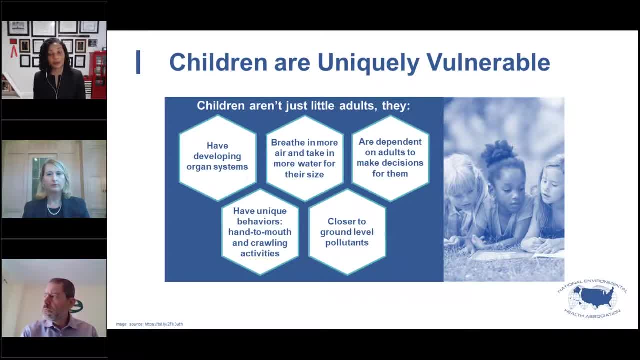 This leaves them more exposed by comparison to adults. So they're not just little adults, They're much more exposed. In addition, they are dependent on adults to make decisions for them, for their wellbeing. Children also have unique behaviors. They have hand-to-mouth activities. They have oral exploratory habits that can allow them to ingest more pollutants or be more exposed. And then they're also shorter, They're closer to the ground and they spend more time playing on the ground, So they're closer to ground level pollutants. 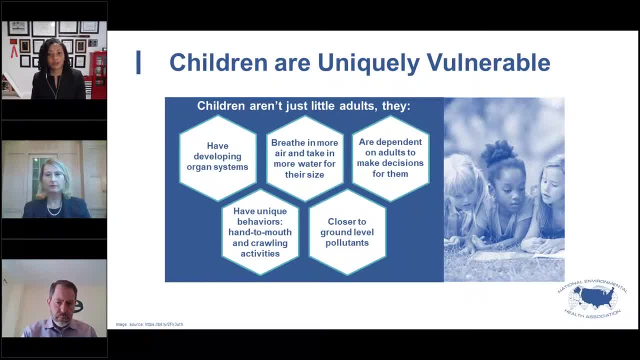 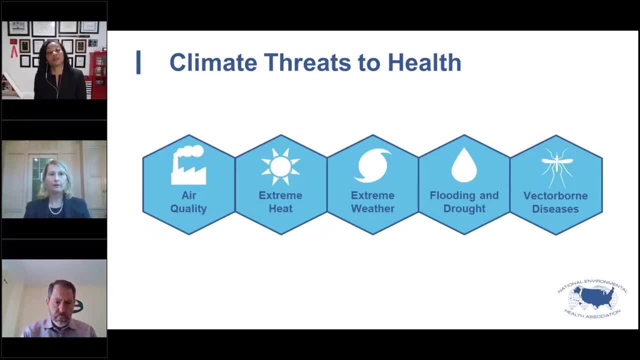 leaving them further, more exposed. So climate change impacts all of our health, but children are uniquely vulnerable. I wanted to give you a few faces as we go into a deeper dialogue around the ways that climate change impacts health Within this I'll share with you. 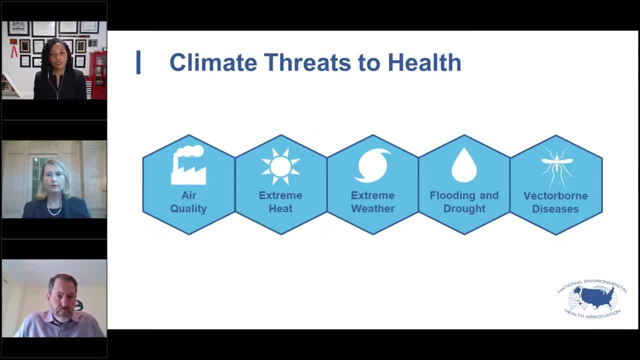 among these five different climate and health threats. I'll also share with you some populations that are uniquely vulnerable to some of these specific aspects. I'll also give you some cues on policy into action: the ways the environmental health workforce is turning policy into action. 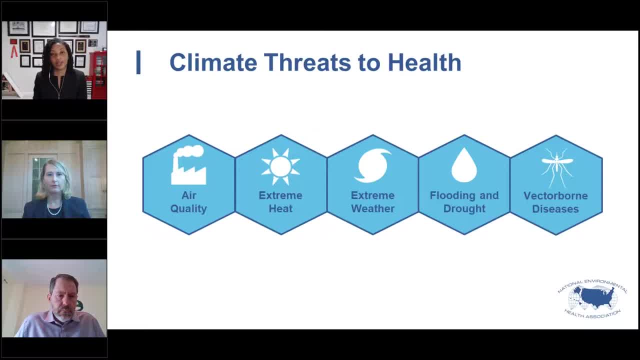 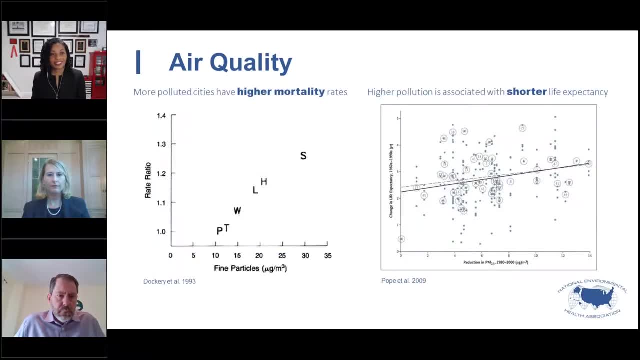 in terms of how they are carrying out climate and health adaptation among these different threats to health. I may have gone too far, though, Sorry, I got way ahead on the slides. That's just a preview of what is to come. Here we go. 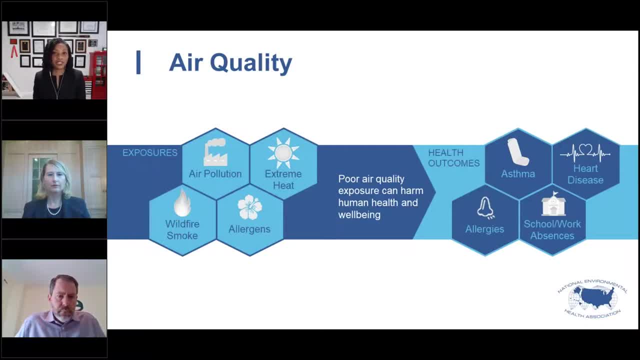 We're in the right place now. So we all deserve clean air to breathe, and climate change is decreasing the quality of the air that we breathe. We have increased carbon dioxide levels in the atmosphere and that is trapping heat and pollutants below, much like a blanket traps heat. 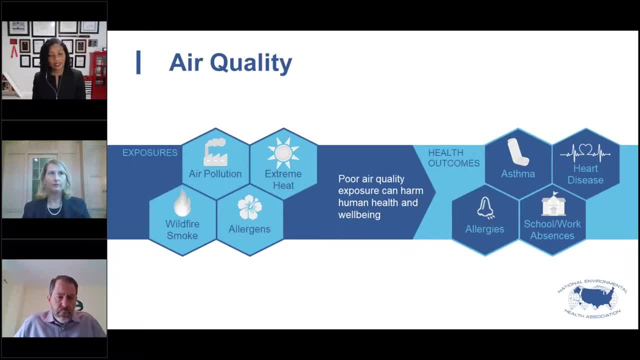 And so air pollution is certainly a threat to air quality. In addition, extreme heat threatens air quality. We have environments that are more conducive to drought. We also have environments that are much more conducive to wildfire, And this wildfire smoke is a threat to health. 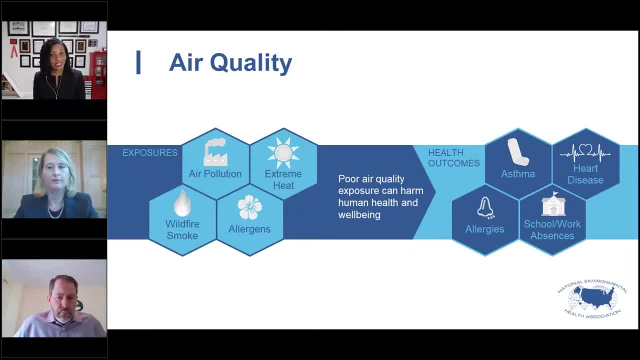 In addition, we have a longer hot or warm season and thereby a longer and more intense pollen season, So this increases our exposure to allergens like pollen. In addition, we have environments that are more conducive to flooding in some regions, So this can leave behind in the aftermath of flood mold. 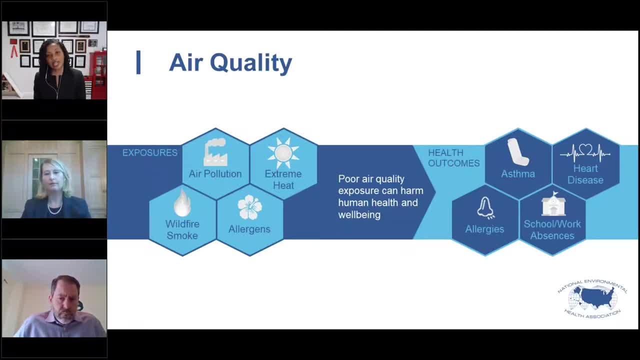 in our homes, our schools, our workplaces. So mold is another key. It can be a major source of allergen that can decrease the quality of the air that we breathe. So these exposures, especially air pollution, extreme heat, can increase our risk of asthma. 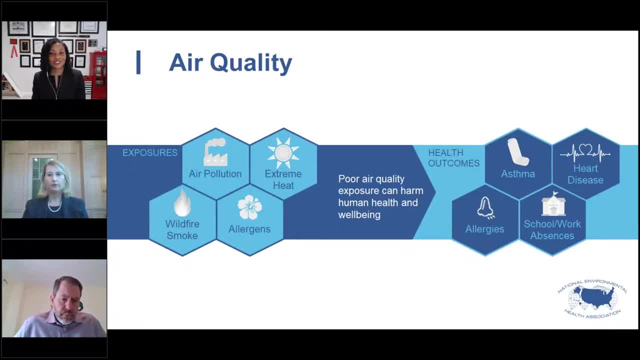 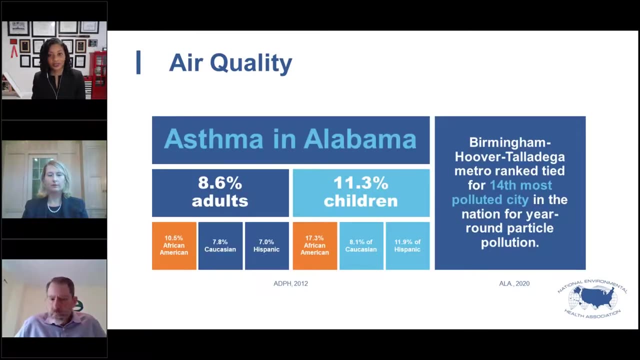 as well as heart disease. In addition, I've made the case that climate change can be bad news for allergy sufferers, And these aren't just nuisances. These can cause school and work absences or can decrease productivity in school and at work. 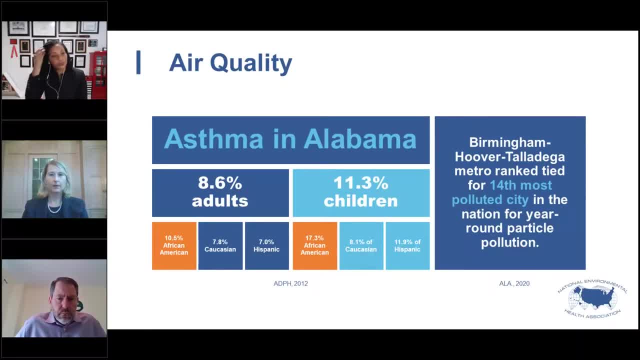 I just want to give a snapshot for an example to hone in on some disparities. looking at asthma, in the state of Alabama, 8.6% of adults had asthma in 2012.. That's similar to the national prevalence of asthma, but it's a bit higher for African-American adults. 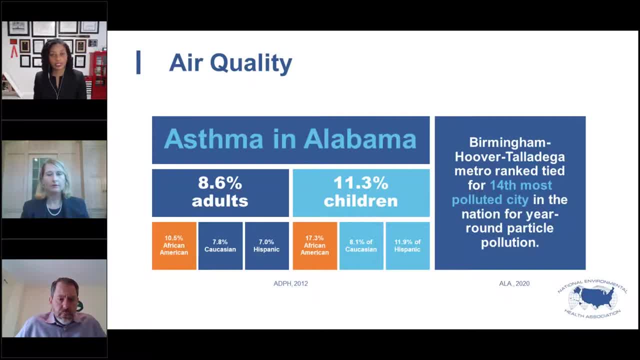 and asthma, as you can see here, close to 11%. Then when we look at children, children have more asthma prevalence And, as you can see, they're more likely to have asthma Alabama compared to adults. But when we look at African-American children, 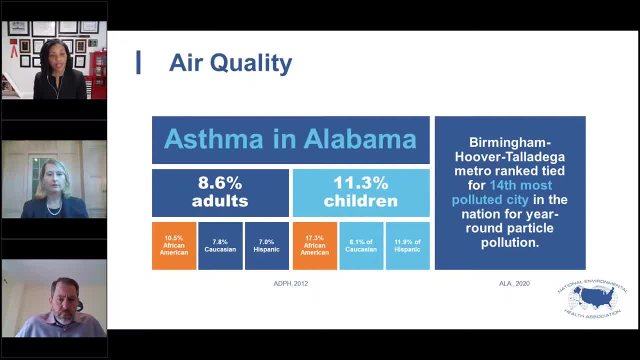 we see much higher prevalence of asthma among African-American children, just over 17%. Then we look more recently at the American Lung Association state of the air report for 2020.. And they reported that the Birmingham, Hoover, Talladega Metro area ranked tied. 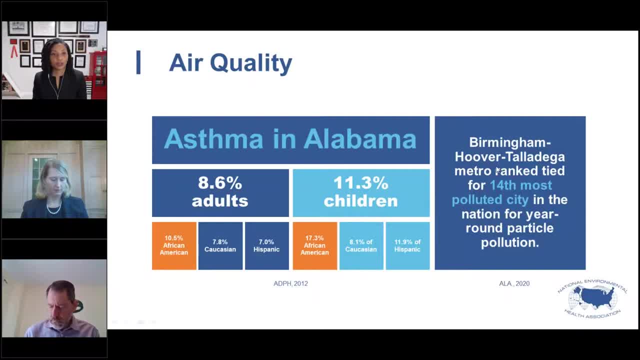 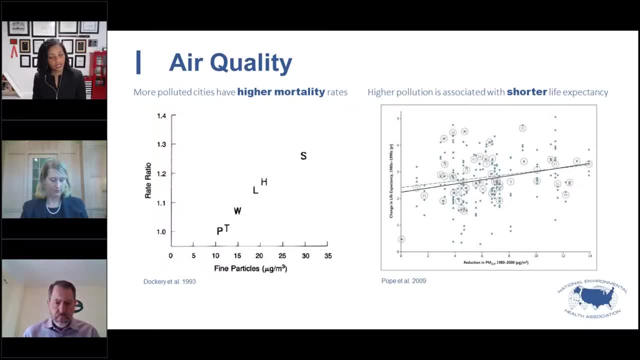 for 14th most polluted city in the nation for year round particle pollution. Now I want to take you back to our roots of understanding around air quality and health. So the Harvard Six Cities Study is a favorite among toxicologists to share. Harvard Six Cities Study taught us: 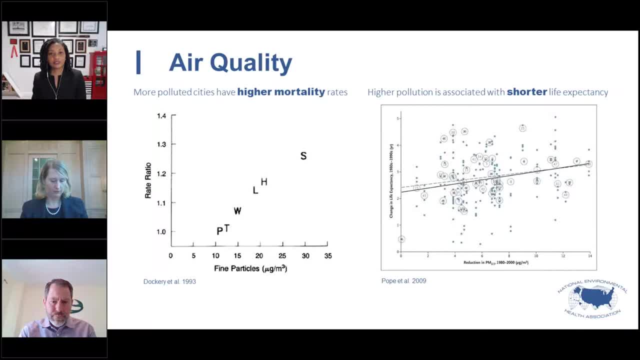 that more polluted cities have higher mortality. You can see here: as the fine particle exposure increases, the mortality rate also increases. More recently, higher pollution has been associated with shorter life expectancy. Arden Pope and others in 2019 demonstrated that as the pollution levels increase, 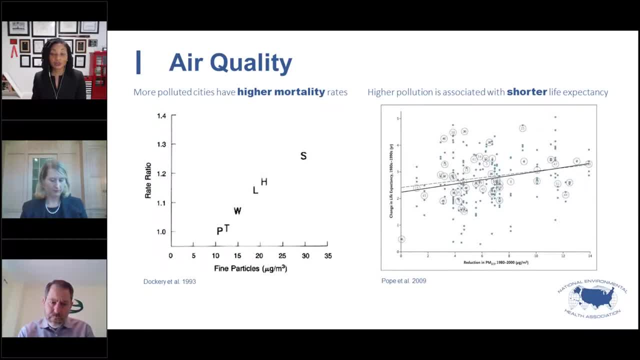 the life expectancy. I'm sorry this was linked with shorter life expectancy. What's really interesting about this study is they actually came back just a few years later and looked at a time period where there's still an increase in air quality. How do I say this properly? 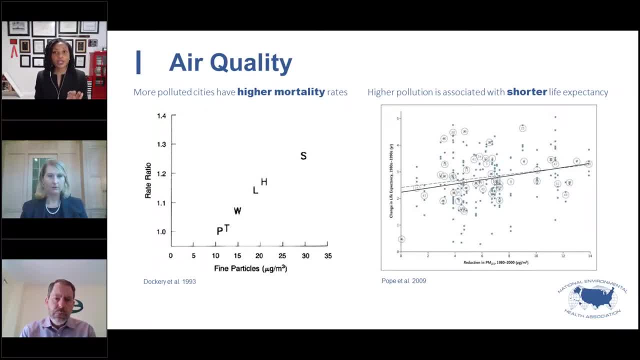 There's still lower pollution, but it's to a lesser degree than the period that's referenced here, And even with smaller decreases in pollution, they still were able to demonstrate significantly increased life expectancy. I hope I haven't confused everyone. I'm happy to take any questions there. 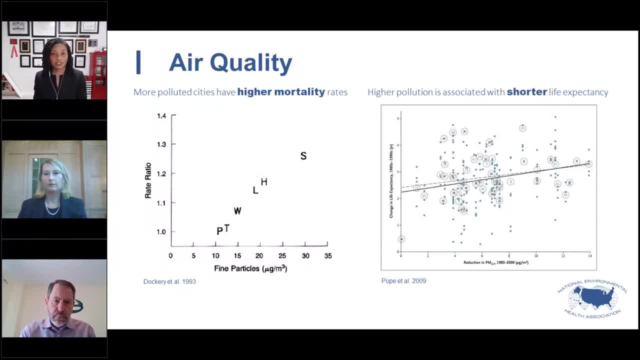 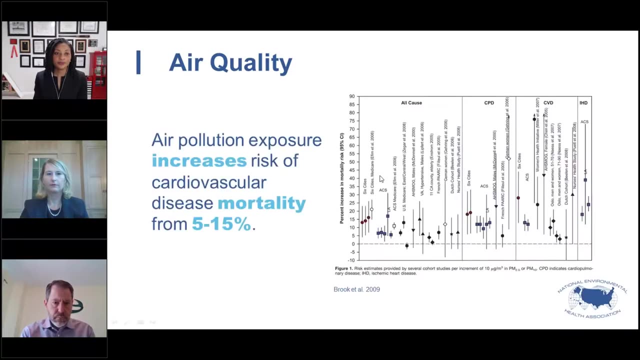 The main point is that higher pollution as associated with shorter life expectancy, and even if we're looking to the benefit of this, even with smaller decreases in pollution, there's still significantly increased life expectancy. I spent a lot of time in the area. 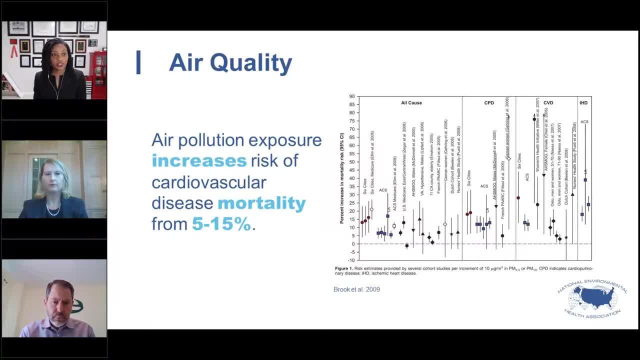 of environmental cardiology, And so I'm really excited to share with you some of the evidence behind the relationship between, you know, the environmental cardiology and the environmental health, And so I'm really excited to share with you some of the evidence behind the relationship. 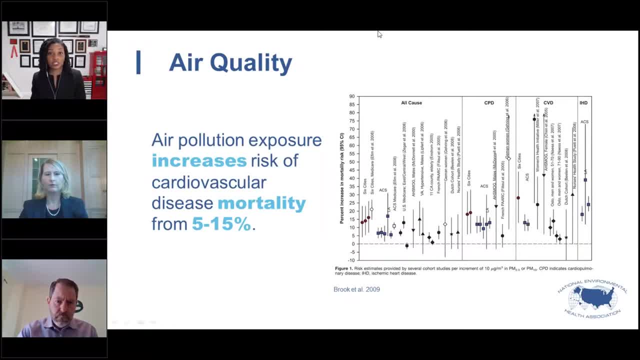 between air pollution and cardiovascular disease. Air pollution increases risk of cardiovascular disease mortality from five up to 15% And if you see this figure here- I hope you're able to see the mouse on the screen. It looks like you are Looking at all cause mortality overall there. 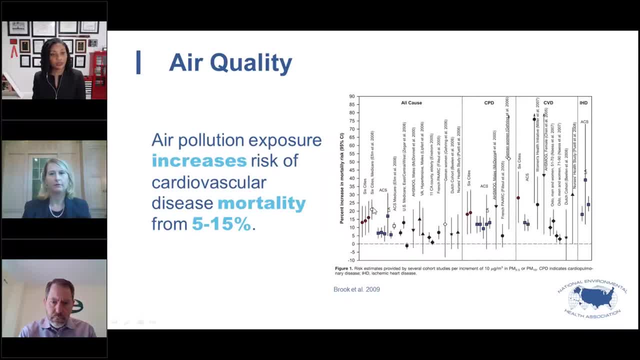 for multiple studies, there is an increase in mortality associated with increased exposure to pollution. I think I've made a good case for that Before this slide, but certainly when you see them all side by side, many are significant and increased. Look at cardiopulmonary degree. 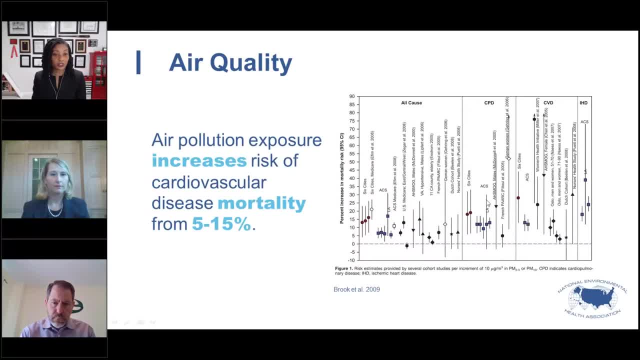 a site- cardiopulmonary disease- you see it to a bit of a stronger degree. But then when you look at heart disease, cardiovascular disease, you see it to an even stronger degree And if you narrow that even to ischemic heart disease. 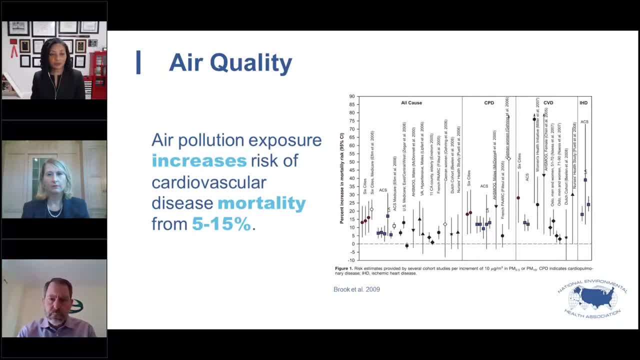 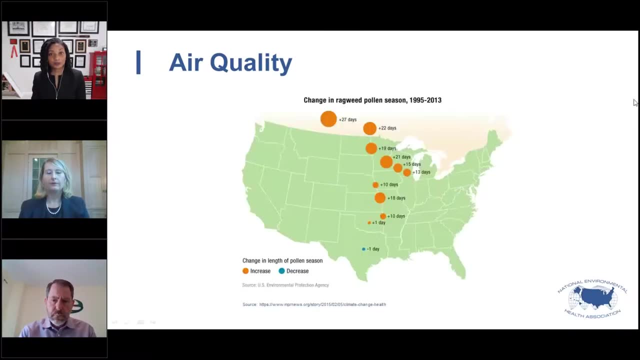 even stronger associations. So the association between air pollution and respiratory disease has been well-defined for quite some time, But when we actually looked a bit closer, that relationship with cardiovascular disease is even stronger. In addition, I just wanted to share with you some evidence on the increased pollen. 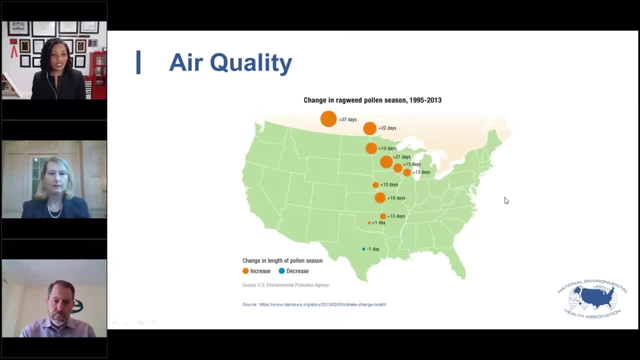 that we're being exposed to. So, looking here at the US and in Canada, we can see that from 1995 to 2013,- this was reported in the 2016 US climate and health assessment as done by the US Global Change Research Program- that there was an increase of 27 days. 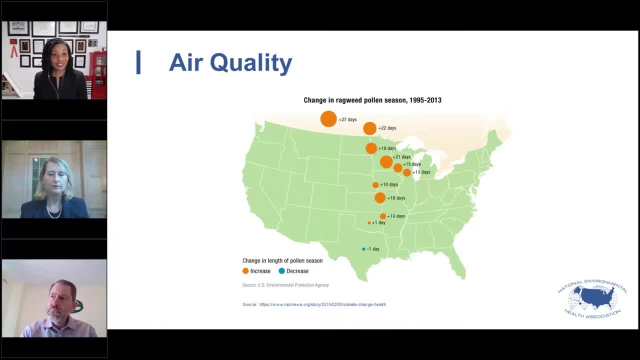 and 22 days in parts of Canada of ragweed pollen. Those days as well as in Minnesota as well as Wisconsin, ranging from 19 to 13 additional days of ragweed pollen season. We're going through the Midwest, 10 to 18 days. 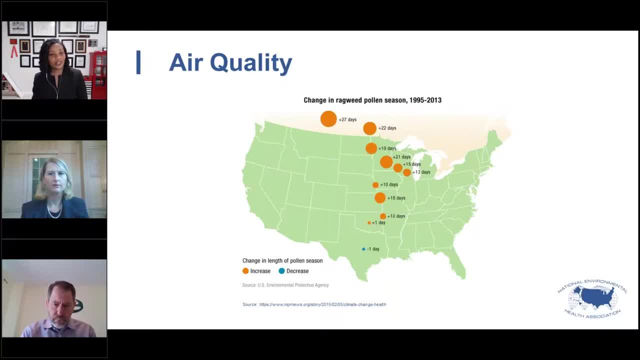 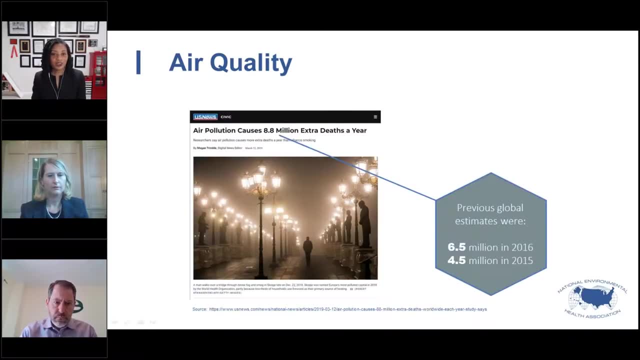 and then we're going through the United States 18 additional days: one additional day in Oklahoma and one less day in Texas. So, bringing all things together, air pollution causes excess deaths. This study, released in 2018, demonstrated over 8 million. 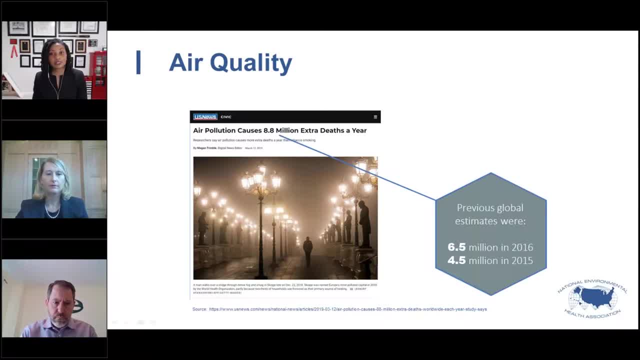 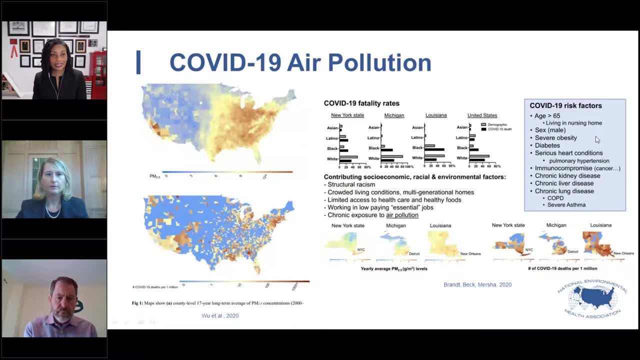 additional deaths per year, And this is an increase over previous reports, from 4.5 million in 2015 and 6.5 million in 2016.. We can't ignore the current scenario, Both climate change as well as COVID-19. 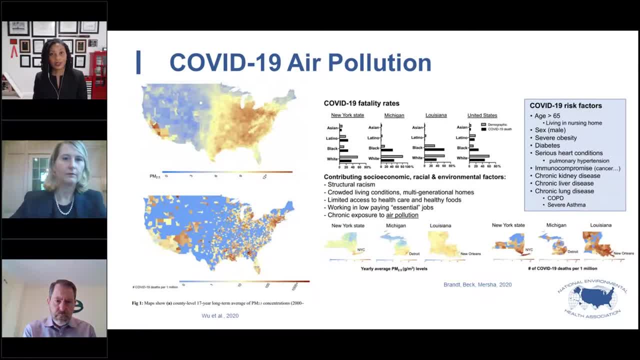 have been declared global health emergencies by the World Health Organization. But, as I shared with you before, climate change is the great threat multiplier And there's evidence that climate change may make COVID-19 worse. So research here. the two maps of the US: 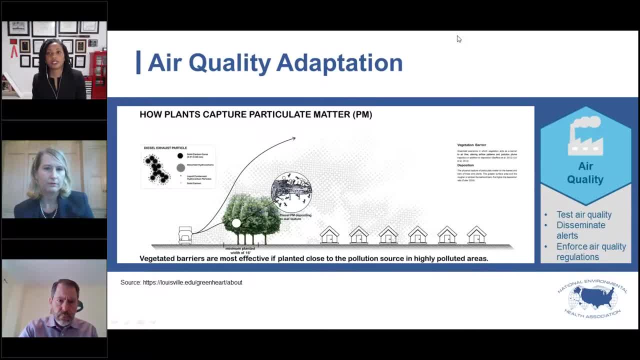 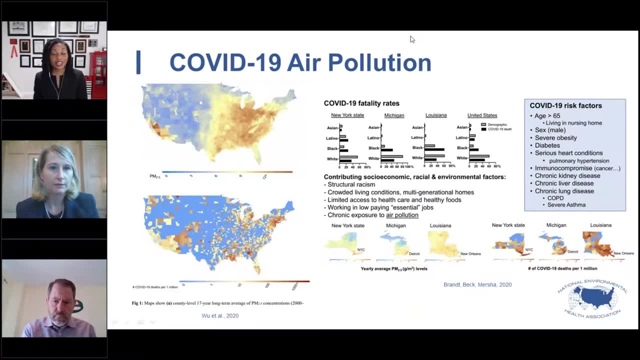 come from Dr Francesca Nominici and others from Harvard University, And they're uh-oh sorry I've skipped past it. There we go, And their research suggests that even a one microgram per cubic meter increase of particulate matter. 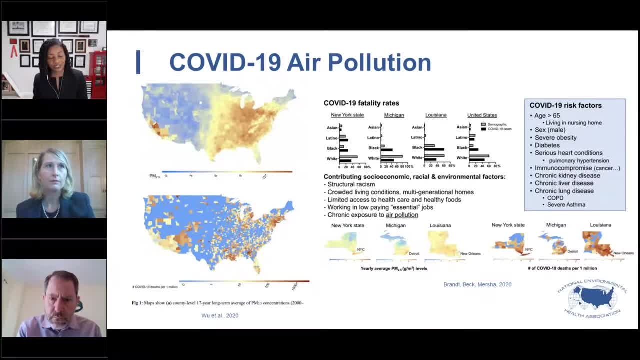 fine particulate matter is associated with an 8% increased COVID-19 death rate, meaning that more polluted cities may have more COVID mortality. Furthermore, Brandt and others also lay out a case for further investigation between the relationship between air pollution and COVID-19. 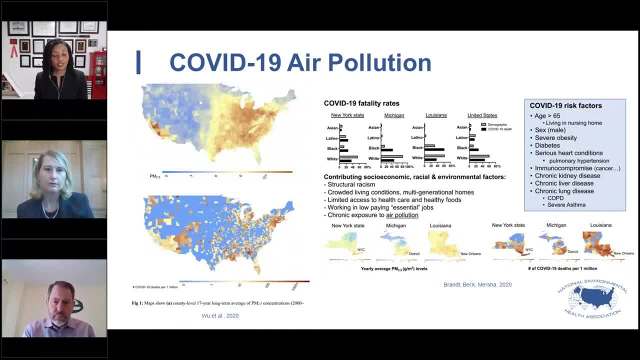 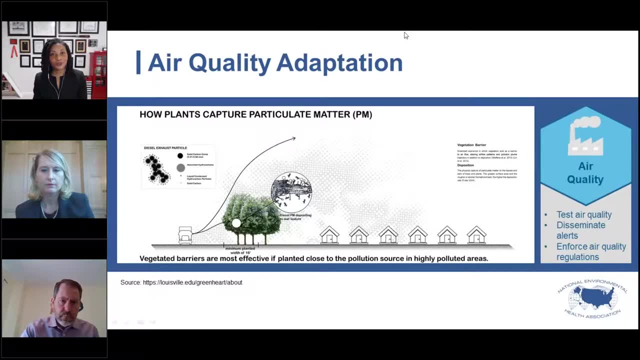 mortality with the underlay of COVID-19 mortality disparities by rates. I don't want to leave you in the dark place of the heavy understanding of the different ways this impacts health. I would like to share with you some of the things that we've been doing in the last couple of weeks. 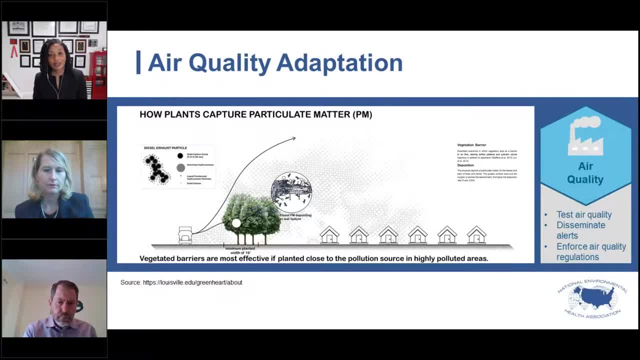 to help you understand the impact of COVID-19 on your health, And I want to share with you a feel-good story about what one community is doing. My colleagues at University of Louisville have partnered with the Nature Conservancy to launch the Green Heart Study. 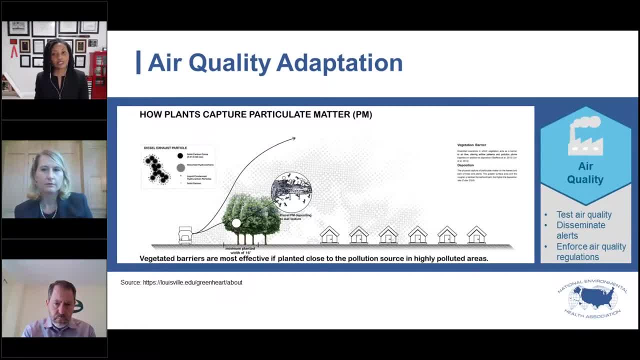 And what they're doing is they're looking at cardiovascular disease markers before, Then they're planting trees, And then they're looking at cardiovascular disease markers and risk following the planting of these trees as an intervention, as a defense against UV rays. It should be presented as an example of how 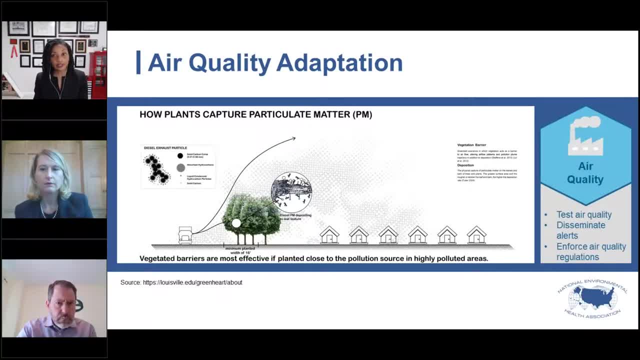 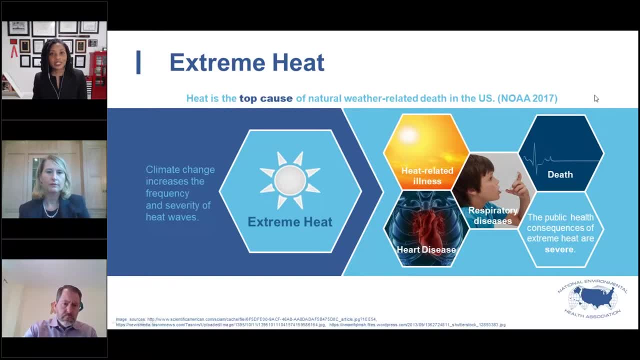 we should be taking that approach. Some of the things that are taking place in the environmental health workforce policy into action include testing air quality, disseminating air alerts and enforcing air quality regulations. So changing gears In 2016,, the US Climate and Health. 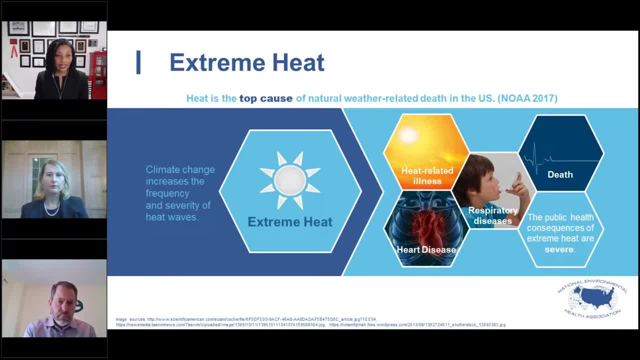 Assessment that is completed by the US Global Change Research program reported that climate change has increased in frequency and intensity of extreme weather events is the top cause of natural weather related death nationwide. So extreme heat can be particularly dangerous for children, as they're more likely to be playing outside. 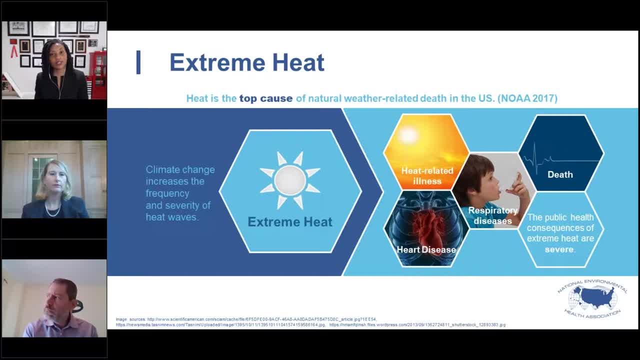 as well as for elderly, as they might be more likely to live in an air conditioned environment and be socially isolated. So this threatens our health by increasing our risk of heat related illness, like heat exhaustion, heart disease and respiratory diseases, as I shared before. 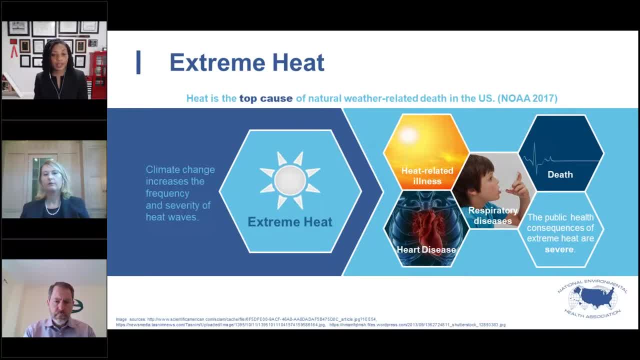 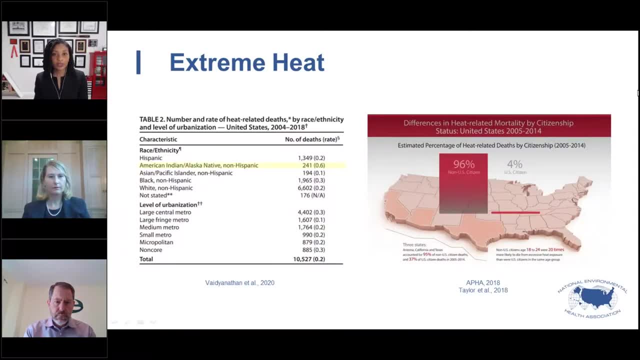 And additionally heat stroke, which can be deadly if not tended to very quickly. So the public health consequences of extreme heat are severe. I wanna point out two populations to you that are quite susceptible when it comes to extreme heat. Just in the last couple of weeks, CDC's morbidity. 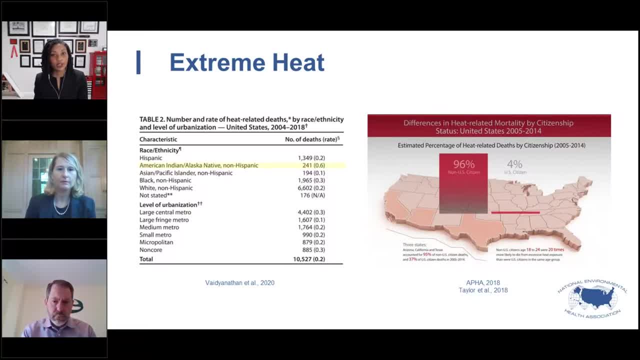 and mortality weekly report released some evidence around extreme heat in the US And if you see here in table two they're sharing the number and rate of heat related deaths by different races and ethnicities And you can see that for whites or Caucasians. 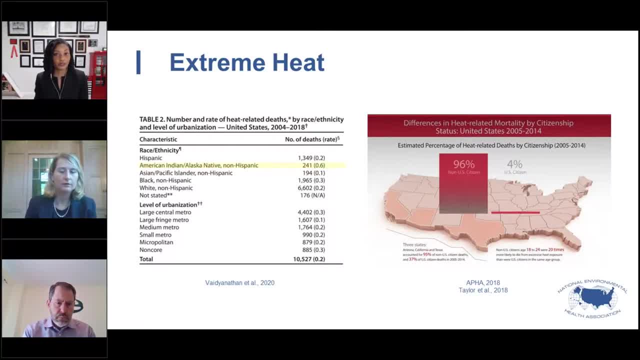 whites or Caucasians have the highest number of deaths for heat related events. However, if you're looking at rates, you see a disparity here where American Indians and Alaska natives, the rate of heat related deaths is much higher for them compared to the other populations assessed. 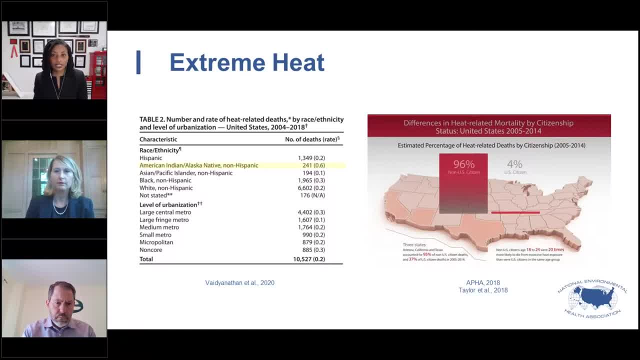 In addition, I wanted to share another population here in the US that's susceptible, And those are non-US citizens. This study published by the American Journal of Public Health. they had a special supplement on climate change and environmental justice in 2018 that examined deaths by citizenship status. 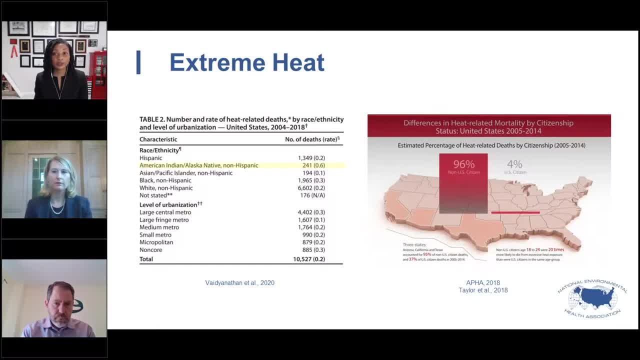 And they found that 4% of the deaths were among US citizens, Meanwhile 96% were non-US citizens, And there were three states in particular- Arizona, California and Texas- that were responsible for 95% of the non-US citizen related deaths. 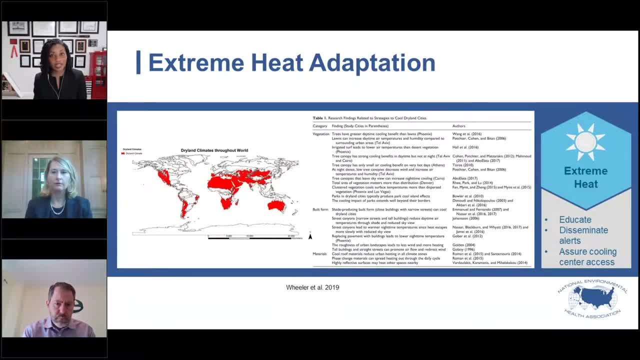 So there's much work that the environmental health is doing to adapt One that I shared with you: tree planting, also building shade, and then partnering with planners so that we can have communities that have health at the center. In addition, the environmental health workforce 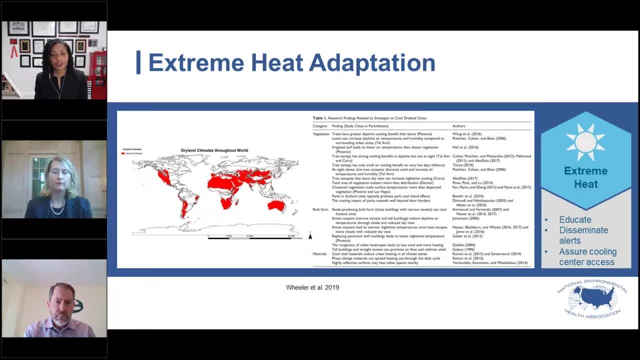 works to educate communities, disseminate alerts and also ensure access to cooling centers. Having cooling centers is very beneficial, but they're not as beneficial if we can't ensure that people are able to get there and cool off on those extremely hot days. 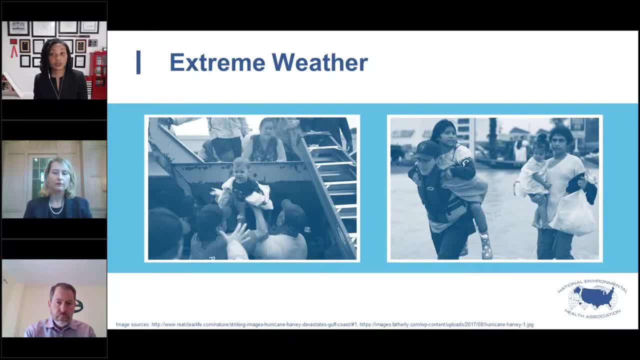 With increased carbon dioxide in the atmosphere. this is increasing service water temperatures and making the frequency and intensity of extreme weather events more frequent and more extreme. 2017,, as I shared before, was a record-breaking year for hurricanes, with hurricanes Harvey, Irma and Maria. 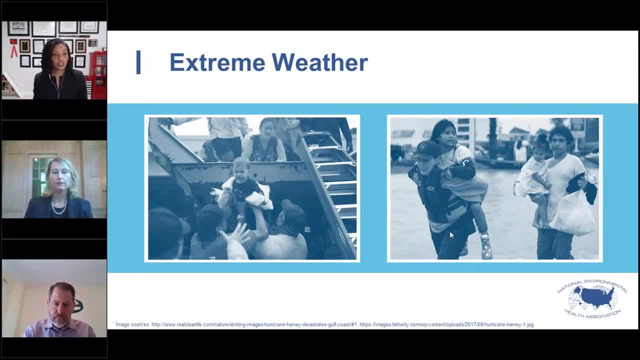 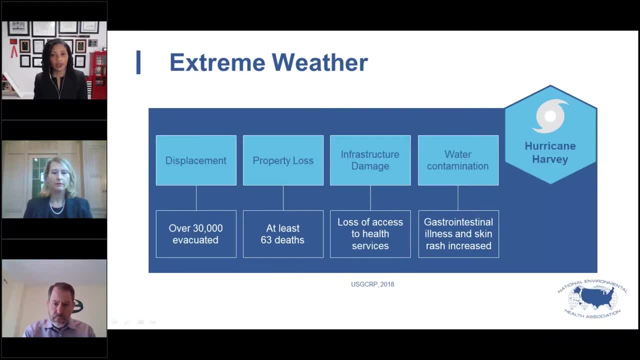 all making landfall here in the US. These photos show some of Hurricane Harvey's youngest victims. I wanted to take you into a bit of a case study on Hurricane Harvey. There were over 30,000 people that needed to be evacuated, So these people were displaced from their homes. 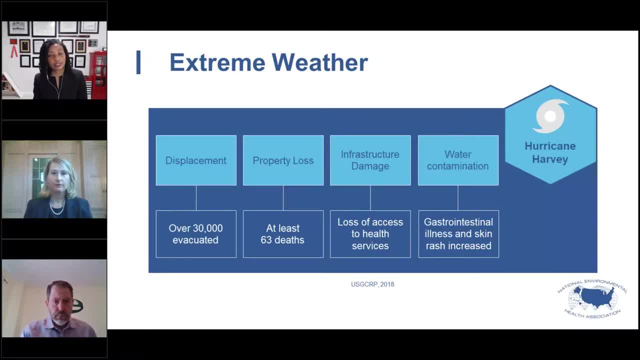 and they were evacuated. So these people were displaced from their homes. So these people were displaced from their homes. There were at least 63 deaths. There was significant infrastructure damage, considering to roadways and more. When this happens, this can interfere with our access. 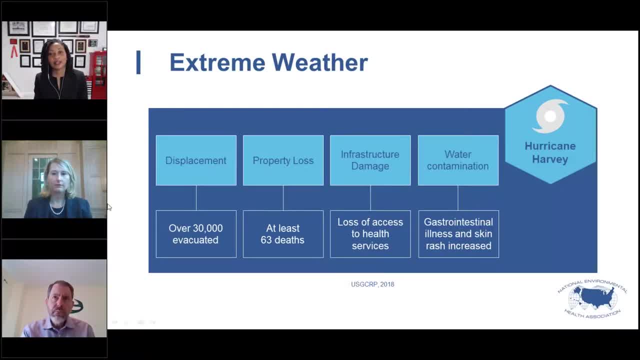 to needed medical services And at such a time as that, the need is even heightened to be able to access hospitals, to be able to access doctors and to be able to even get prescriptions filled for prescriptions that are needed to maintain life. In addition, there was significant water. 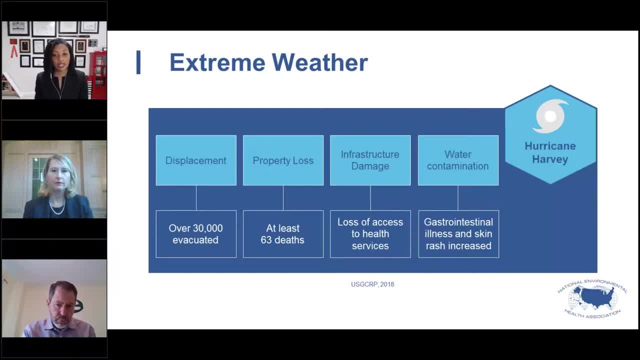 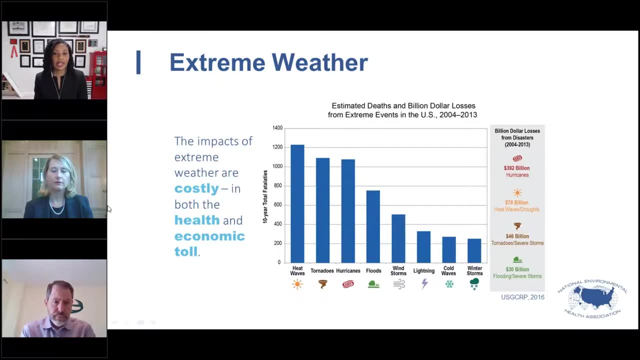 contamination that was reported there through breaches at industrial facilities, And the population reported increases in gastrointestinal illness as well as skin rash. So this particular figure displays that the impacts of extreme weather are costly in both the health toll as well as the economic toll. 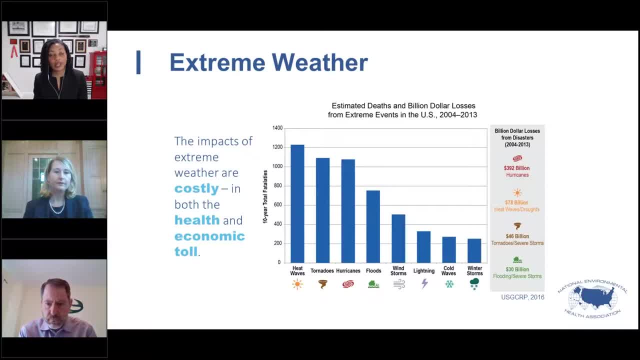 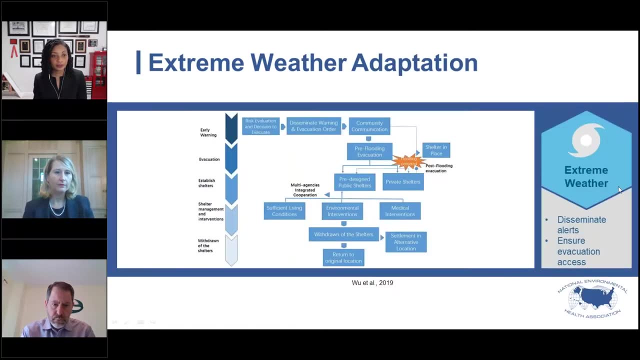 So these are storms, These are climate events that exceeded a billion in losses in the US And of course you can see, the mortality is highest, once again, for extreme heat, followed by tornadoes, hurricanes and floods. And so much of climate and health adaptation. 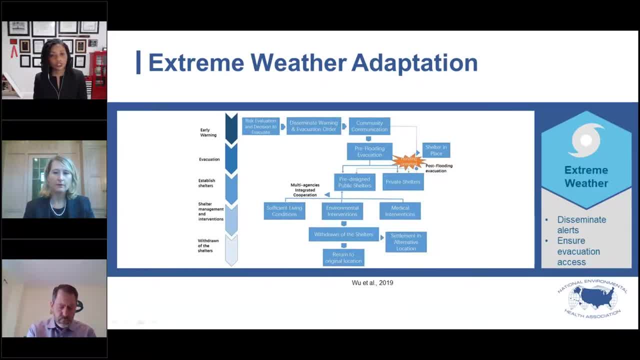 is preparedness when it comes to extreme weather, So ensuring that people have evacuation plans and are able to evacuate, And so the more that people evacuate, the more that they have the safety to further one evacuate And the sooner before the event that one evacuates. 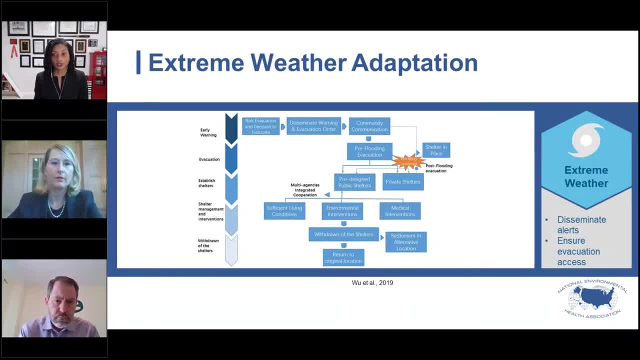 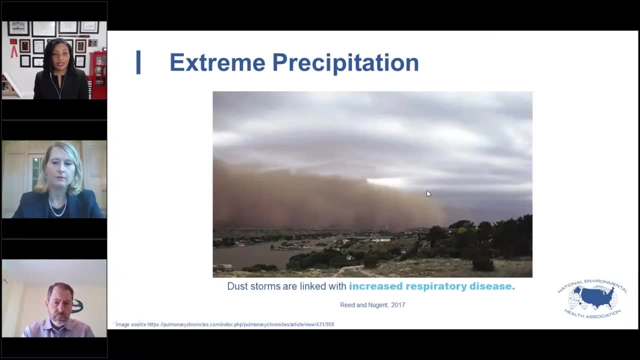 has very positive effects on physical and mental health. So the environmental health workforce is part of helping disseminate these alerts, making sure they're received widely. And also similar to being able to access cooling centers, being able to actually access evacuation and shelters. 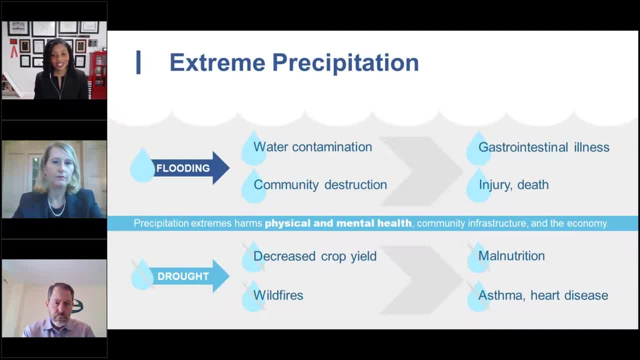 I went too far once again, All right. so transitioning into extreme precipitation, On one hand we have more extreme flooding And the other hand we have more extreme drought. So with flooding we have water contamination, as was an example in Houston. 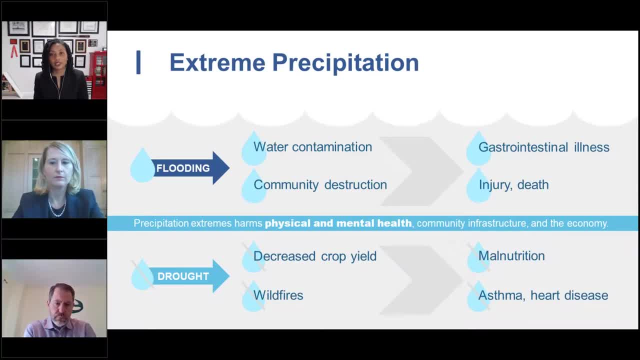 This can increase risk of gastrointestinal illness. There's a study that looked at waterborne disease outbreaks in the US and they found that over half of waterborne disease outbreaks in the US were, you know, preceded by an extreme rainfall event. We also have community destruction that results. 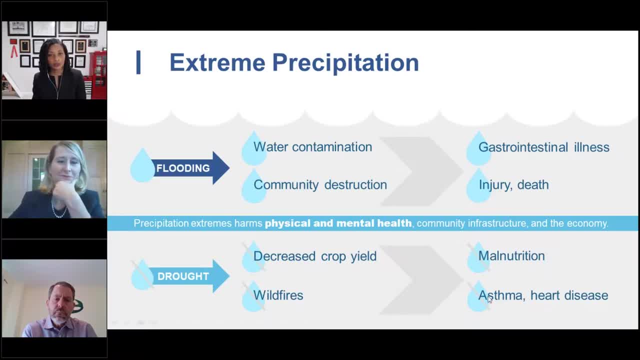 that can lead to injury and death. When we look at drought, we see effects to agriculture, for example, so there can be decreased crop yield. This can actually contribute to malnutrition, which is something that we're seeing internationally. In addition, drought contributes to environments. 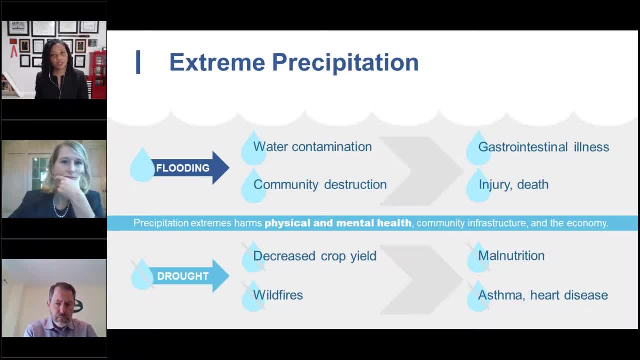 that are more conducive to wildfires, and the exposure to that wildfire smoke can once again increase risk of asthma and heart disease. So the extremes of precipitation harm physical as well as mental health, but in addition to that, community infrastructure as well as the economy. 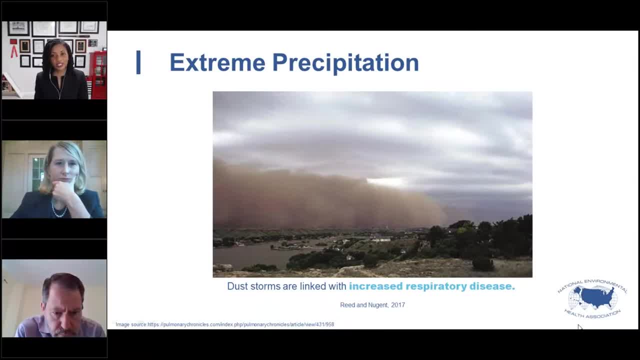 So this is an example of dust storms and these are coming from the Midwest, or this photo is from the Midwest, And dust storms can increase respiratory disease. This can be brought about by drought, or drought can make more conducive conditions for dust storms. 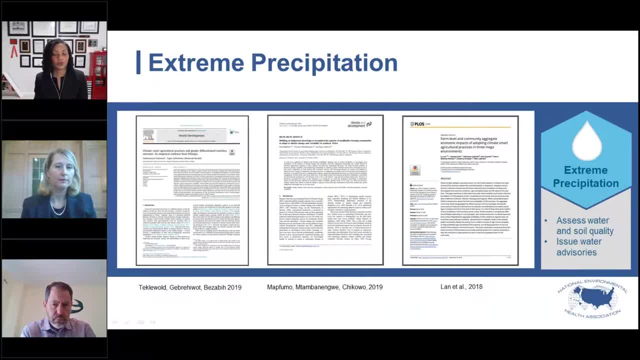 So we have to look out for certain vulnerable populations when it comes to dust storms. Then I wanted to share just briefly some activities of the environmental health workforce policy into action. when it comes to extreme precipitation, We provide resources and education for climate, smart practices for agricultural workers. 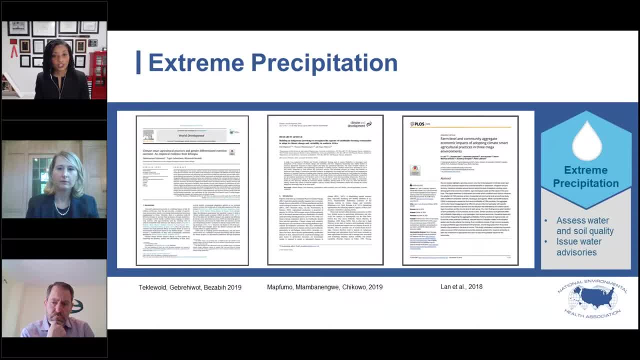 farmers, in particular teaching around crop diversification, soil and water conservation. These together can actually improve household diet diversity and even impact gender differences, especially internationally. Other things that we do here in the US include the assessment of soil and water quality. 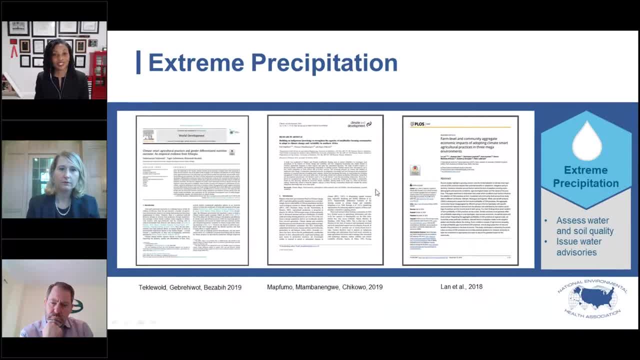 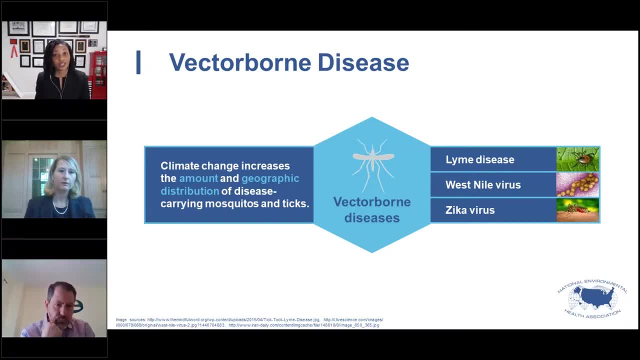 as well as issuing those soil water quality advisories. So the last of the climate impacts to health that I wanted to share with you about is vector borne disease. Climate change is increasing the amount and geographic distribution of disease, carrying mosquitoes and ticks, including changes to the distribution of Lyme disease. 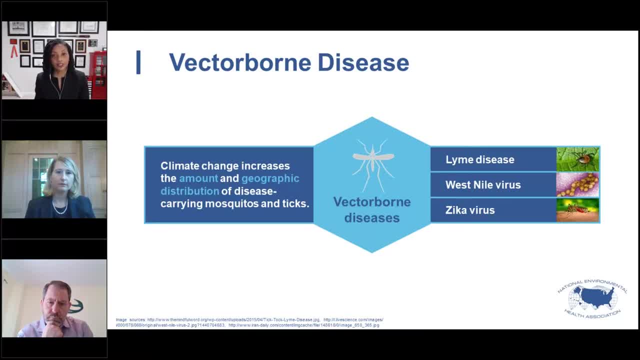 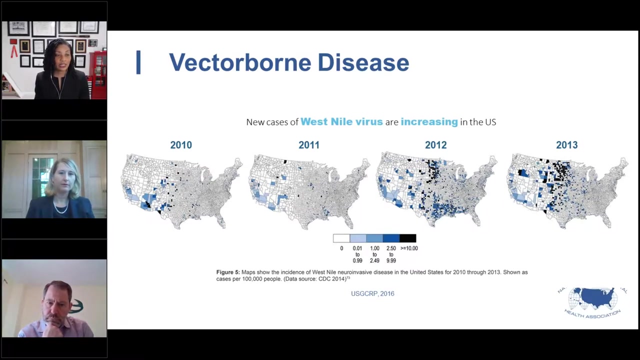 across the US, West Nile virus and even Zika virus. One moment, I think there's a little lag on advancing this slide. There we go. So this depicts West Nile virus across the US and demonstrates an increase from 2010 to 2013,. 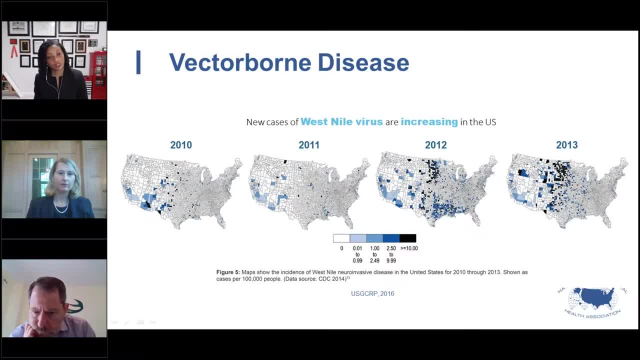 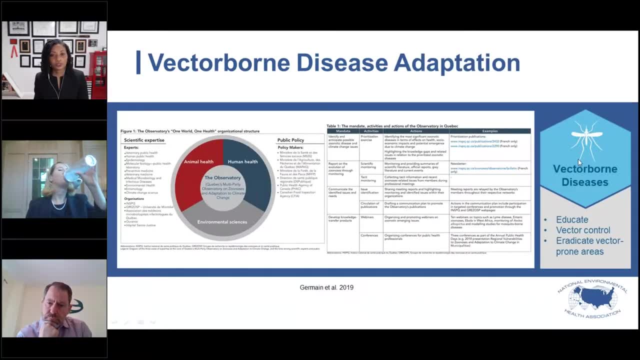 but it also demonstrates a difference in the geographic distribution of West Nile virus in the US and in the region, which is about three times the population of West Nile Next slide. So the environmental health workforce utilizes one health approach that brings together policymakers. 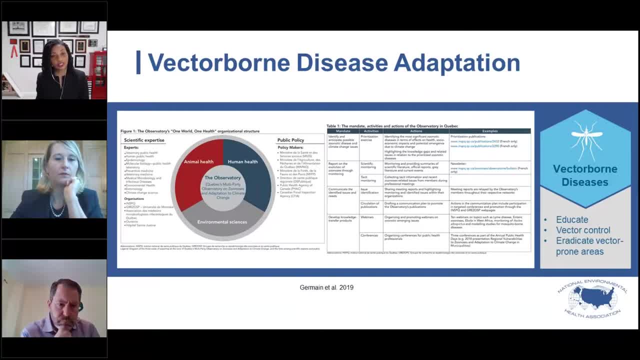 decision makers, folks with expertise in vector borne disease management together, among others, but particularly for vector borne disease, to address adaptation in this space and protect communities from vector borne disease. workforce works to educate- In Maine, for example, the environmental health workforces. 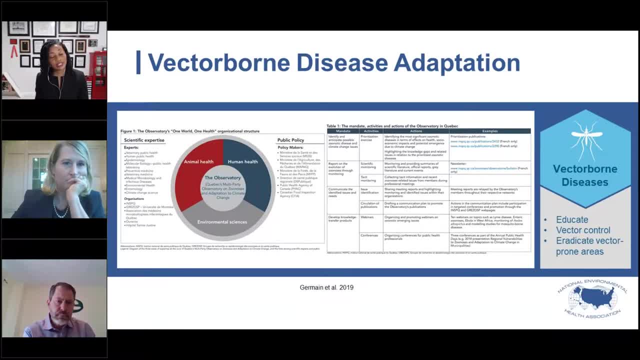 work to educate physicians that they're going to see increases in Lyme disease. in practice, Vector control is a very popular area within the environmental health workforce. Within NEHA's membership, vector control is the second largest specialty area And, you know, the core of public. 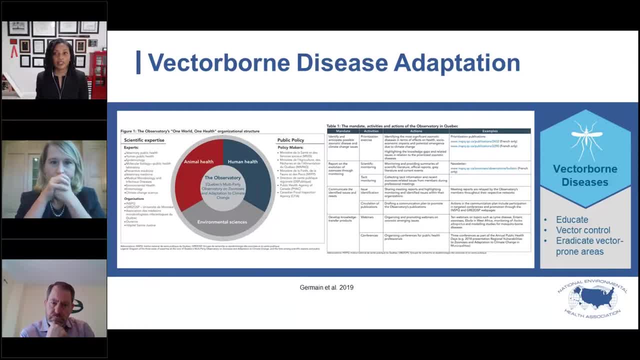 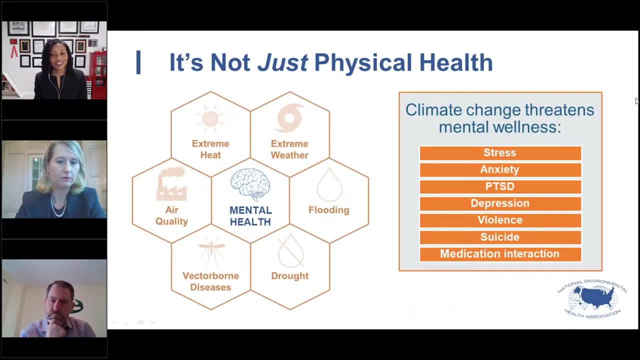 health is prevention, And so eradicating areas that are vector prone- so that would be areas that have standing water, areas with trash that lingers, for example- these would promote vectors, So being able to eradicate those can help prevent vectors. I want to highlight to you: 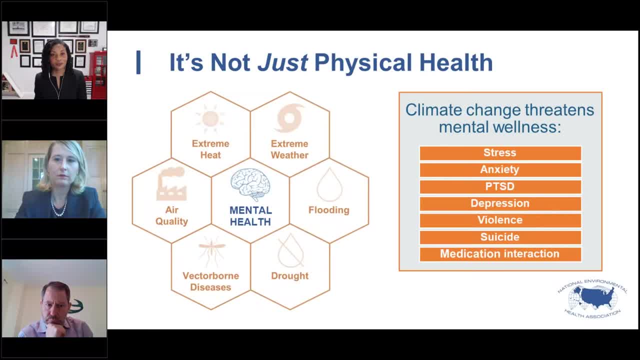 briefly that it's not just physical health that's at risk. I gave a lot of examples of the way physical health is threatened, but our mental health is threatened also by climate change. Climate change, exposure to extreme weather, in particular, and floods, can increase. 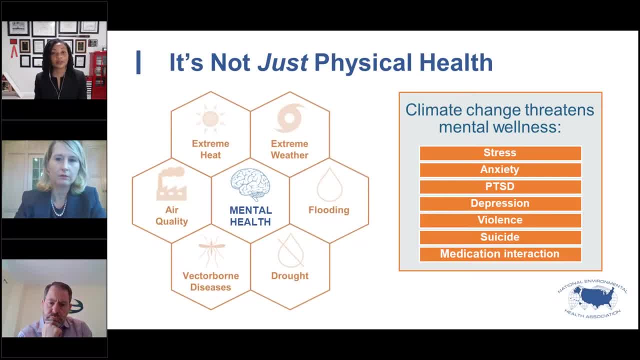 risk of stress, of anxiety, of PTSD and depression. Nearly half of Hurricane Katrina survivors developed a mood or anxiety disorder And one in six developed a post-traumatic stress disorder. In addition, extreme heat and extreme weather can increase risk of depression of violence. 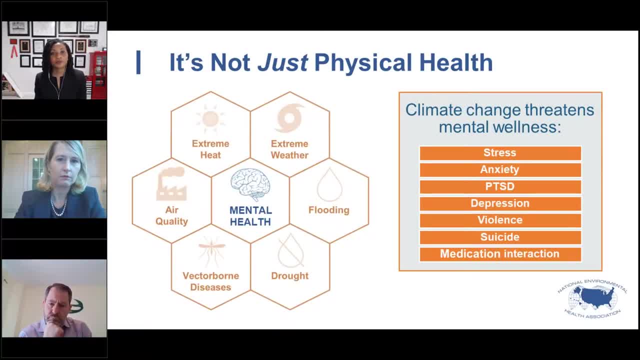 of suicidal ideation or even suicide. Extreme heat can also render active, render inactive, some psychotropic medications. Also, drought and extreme heat can cause conflict, especially internationally, where land is no longer sustainable, through drought, for example, and tribes, nations will need to move into other areas And this can certainly contribute to conflict. 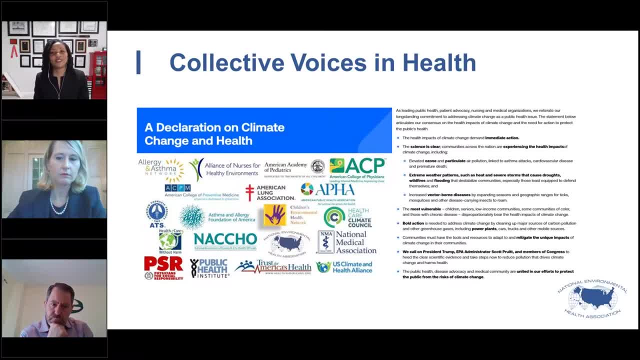 So I don't want to once again leave you in the dark place. There are many health organizations that are calling for action. NEHA is part of this amazing group that's led by the American Lung Association that comes together to to, as a group, stand and say that we call for nothing to undermine the Clean Air Acts authority. 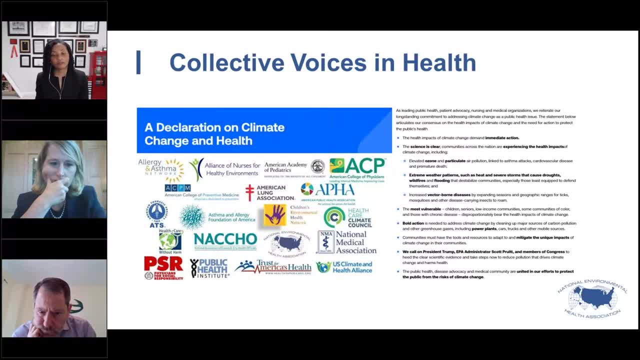 because of the significant health benefits that have been that we have benefited from through the Clean Air Act. In addition, we all also collectively call for climate action, and we do that from a health perspective. So just wanted to share with you and put a human face on the many ways that climate change impacts health. 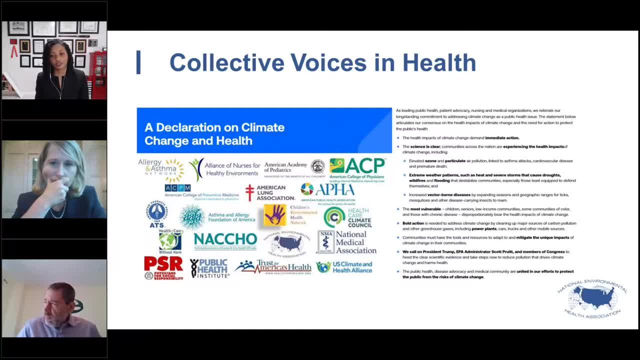 but through the lens of clean air, as clean air is very strongly connected to climate change and climate action in particular. So I thank you for your time. I'm happy to take your time If you have any questions. I'm grateful for this opportunity once again. 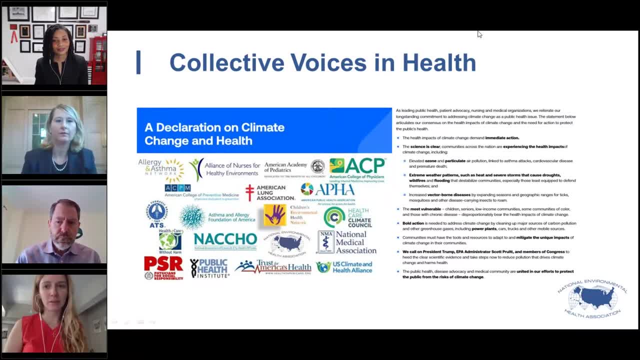 Thank you all so much, So we will now turn to questions. Let me open up the first. All right, Thanks for your patience. So the first question that we have for any of the panelists who want to answer is: our participant asks: how is the Clean Air Act implemented? on the Clean Air Act: 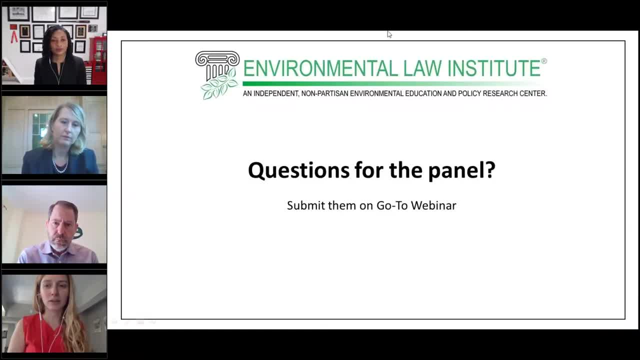 Is it any different than non-tribal lands? Well, I can start that on Stacey if you want to add anything, but it basically depends on the size of the tribe. The larger tribes are basically treated as states. They have their own environment departments and functionally it's the same. 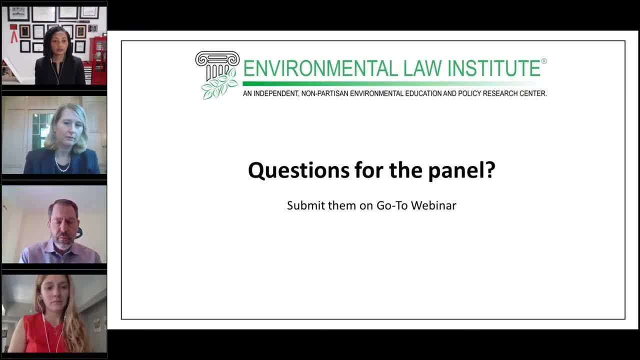 Some of the smaller tribes basically wind up being under state authority because they're too small to have their own programs. I don't have anything else to add to Larry's answer. Perfect, Thank you. So another question is. one of our participants asks: what are the main current EPA efforts to control greenhouse gas emissions? 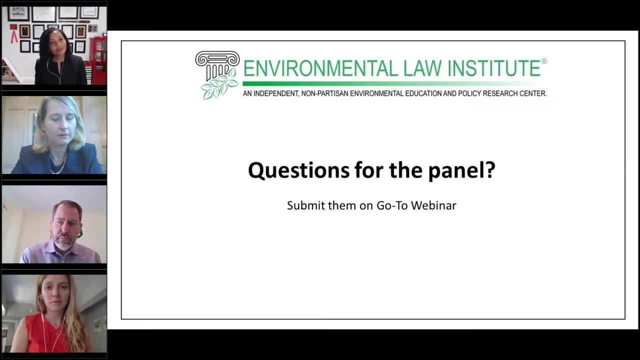 Okay. So We have a regulation on fuel efficiency in cars and other mobile sources. They have a wide variety of voluntary programs. We have very active programs working with state and local governments to help them both plan for and adapt and also to get reductions as well. 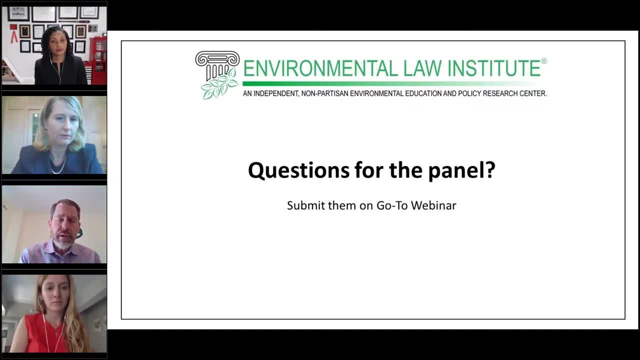 And we have. I mean, we got rid of the Clean Power Plan but replaced it with AIDS, which should hopefully get some reductions as well. Thank you. Another participant asks what the deadlines are like for bringing non-attainment areas into compliance. 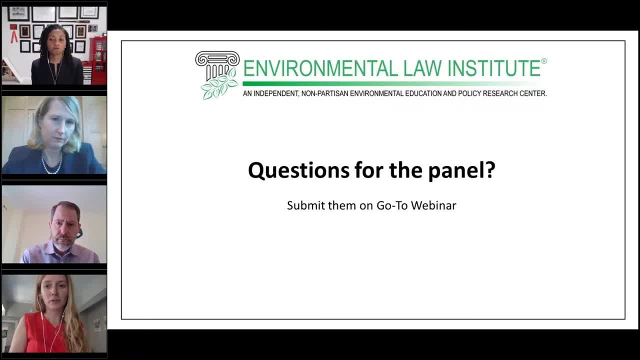 Do states set those individually, or is that a federal action? Okay, so the Clean Air Act has provided deadlines for attainment for states bringing areas into attainment based on the level of pollution in the area. So the worse the air pollution, the more time states have. 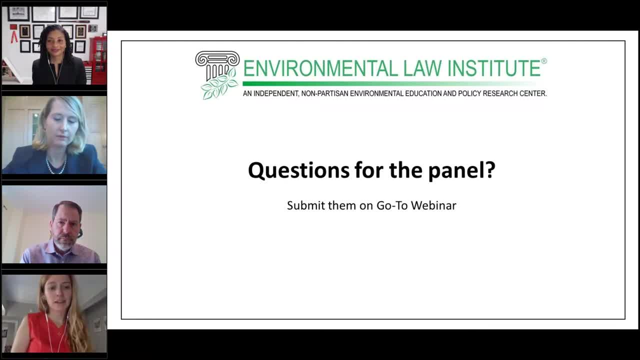 Perfect. So another Participant asks if each of us want to speak on. you know where you see opportunities for folks who are participants in today's audience or more. you know everyday people who can provide action in this area to ensure cleaner air. 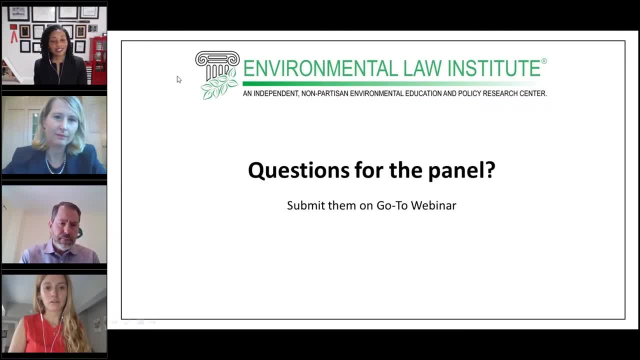 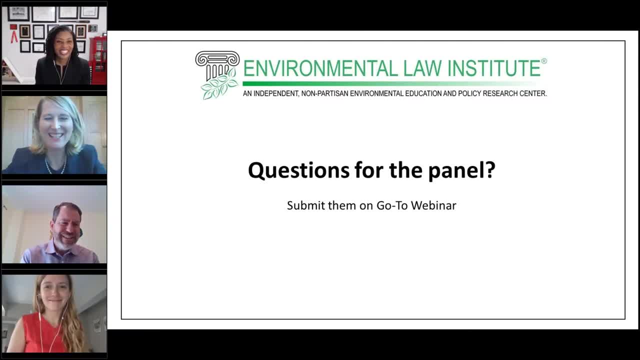 So I would like to call to ensure that health is at the forefront of this. I'll give Larry a break, since he's had to go for the first three questions. I would just add that, as we highlight it throughout today's presentation, the Clean Air Act contemplates a role for the public in both setting standards. 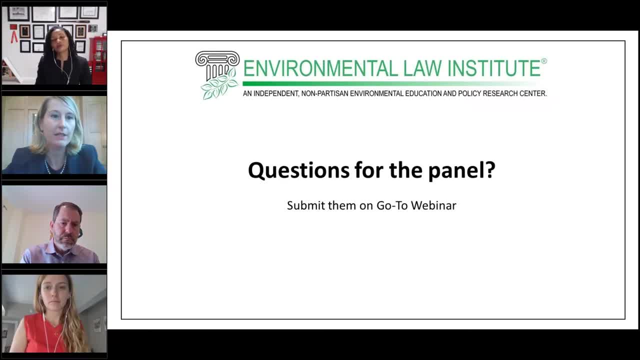 but also commenting on individual facilities who are going up for permits. Those are often available on state websites. You can see what permits are up for review and participate in that regard as well through the existing processes set forth in the Clean Air Act. I would also add that you know. 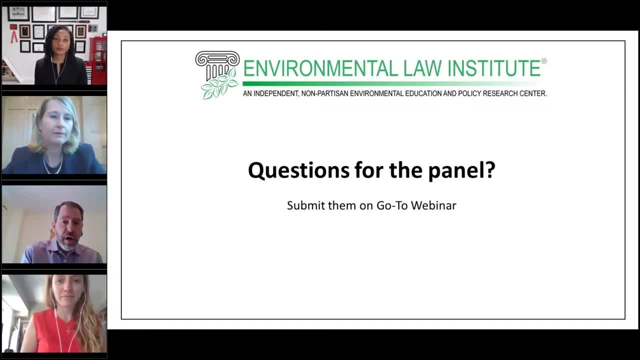 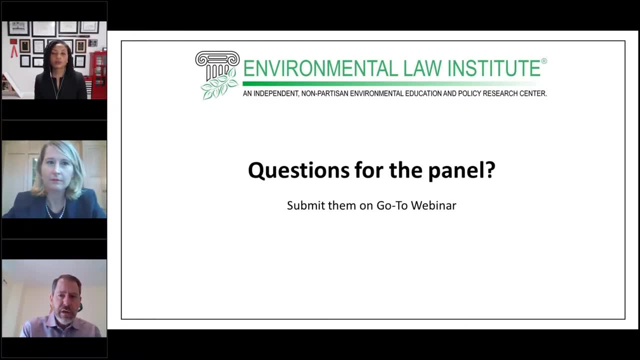 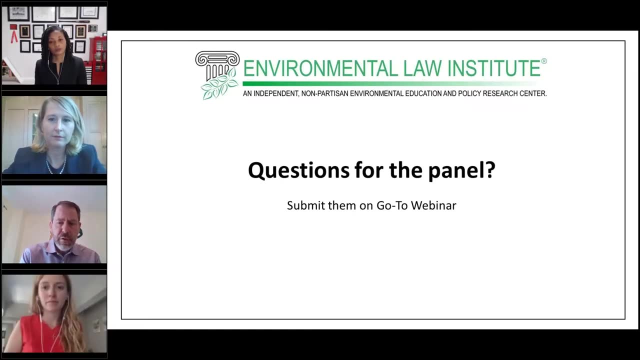 especially when it comes to climate. all of us are taking action that you know results in emissions of greenhouse gases and we can increase our own energy efficiency to help reduce total emissions you know be part of the solution. Thank you all. 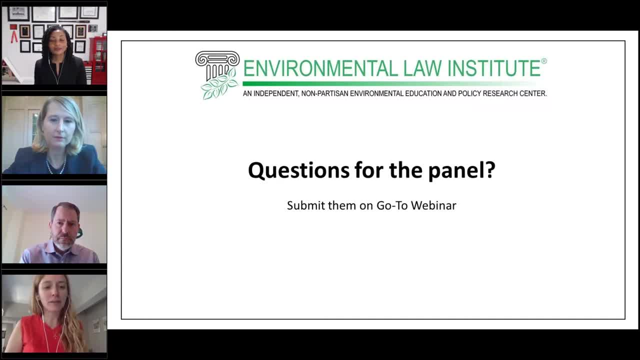 We have another question from a participant. Are enforceable limit standards and permits determined by federal or state authorities, and who would write these permits? So in the NSR? I'm sorry, go ahead, Larry. No, I was going to say: do you want to take it, Steve? 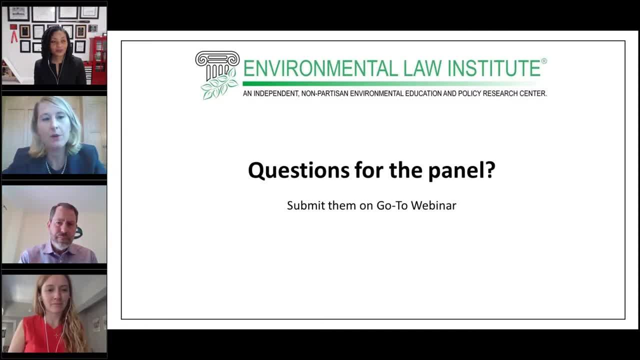 So in the NSR program, which is probably the best example, typically most states have the delegated authority. There are some states where it's not been delegated, but that's probably the majority rule. So your state permitting agency would set the limits. 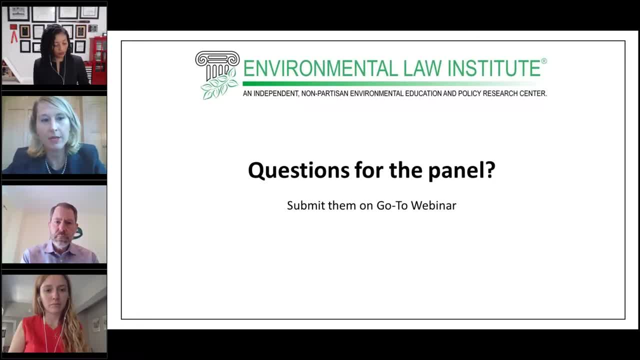 based on their review under PSD or NSR in your construction permit is the general rule. And just more broadly, EPA standards sets the general federal standards which states are enforcing. but states can always go and be more stringent. So in any given state for any green facility. 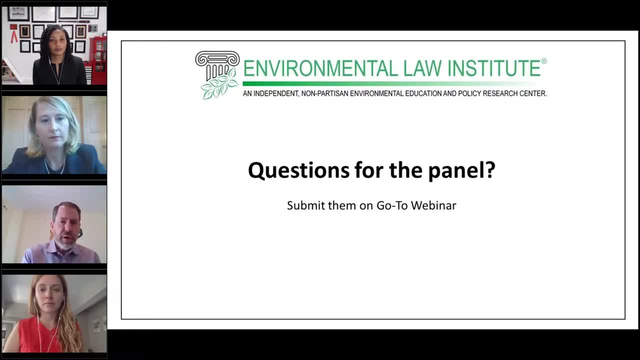 the state has more stringent rules than the facility would have to comply with those, But at a minimum they have to meet federal standards. Thank you both. Another participant asks criteria pollutants like carbon monoxide are naturally occurring. Should carbon dioxide, which is naturally occurring? 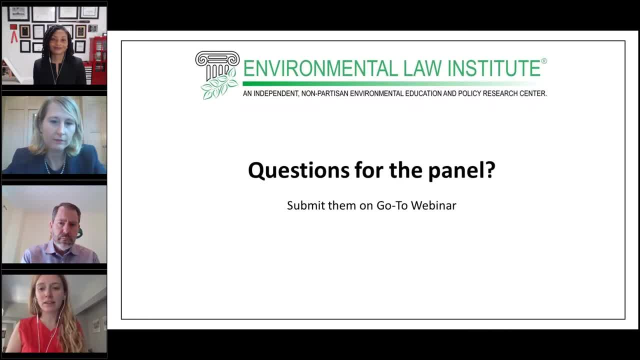 and causes climate change and associated effects be regulated as a criteria. pollutant I mean, I'm sure there is carbon monoxide naturally occurring but there are not health effect levels of carbon monoxide anywhere. Part of the issue with having attainment for carbon dioxide. 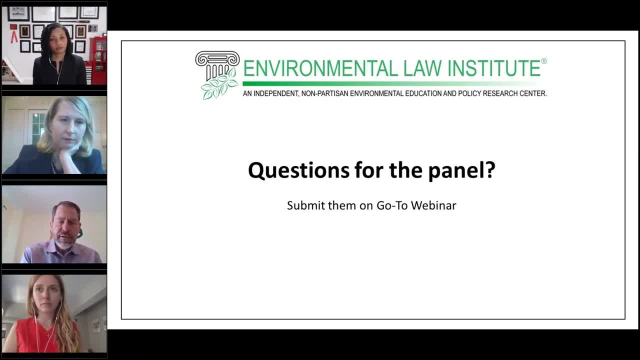 is simply that there's a state couldn't write a set that would guarantee attainment with whatever. I mean, assuming EPA would set a specific level of standard for carbon dioxide, which would be pretty hard to do. that there's nothing that any individual state 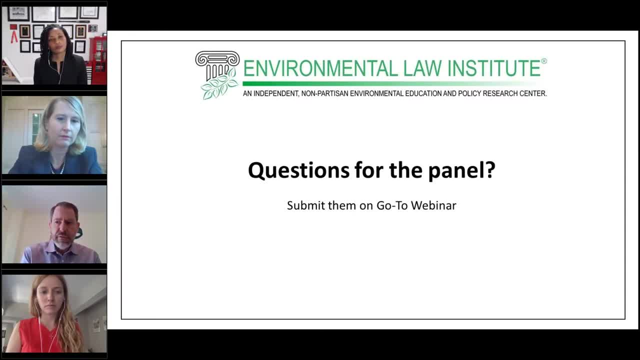 I mean a total individual state for a specific area, could have zero emissions and that would not, you know, wouldn't necessarily cause attainment for any standard that would actually be meaningful. So it's not a very practical solution because it doesn't lead to any actual- you know, real- attainment. 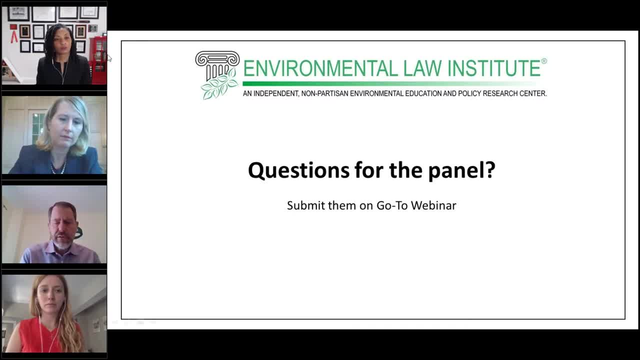 I mean you can't do an attainment situation, so the whole kind of concept isn't really workable. Okay, and we have a related question. A participant asks how and why were the original criteria pollutants selected? My understanding- and this is not an area I have huge expertise in- 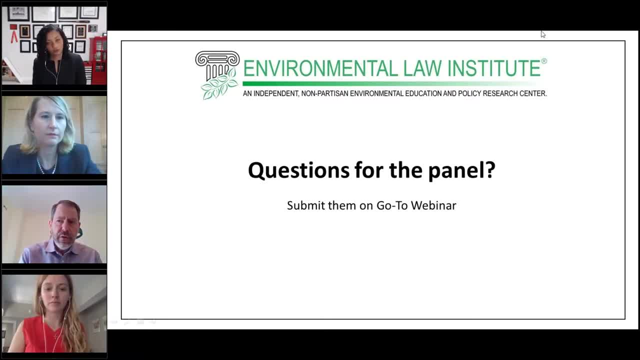 but they were selected because they were basically ubiquitous in an area. So, as opposed to the air toxics which, for the most part, are going to be released from very singular points and their effects are going to go down as distance from that point occurs, 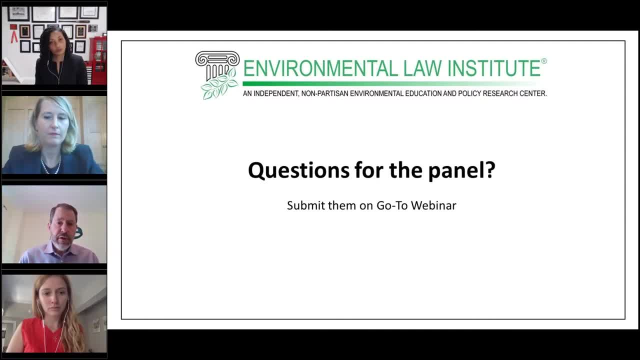 And you know, in an area like New York if they're in non-attainment for ozone, there aren't like different. I mean there may be some variation but as a general rule all of New York City is in non-attainment. 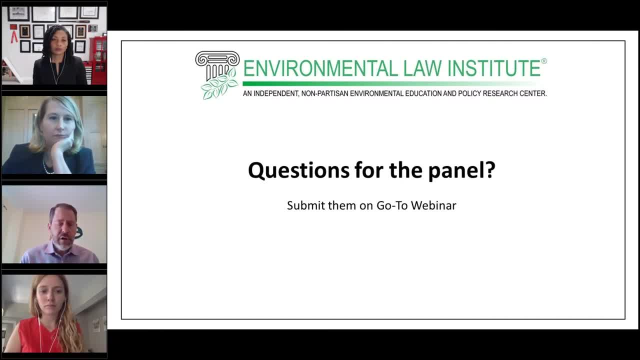 All of the air. air is bad And so that's why the site concept of ambient air, So carbon monoxide, would be in, you know, most of an urban center. If the urban center had problems, it would be, you know, very broadly based. 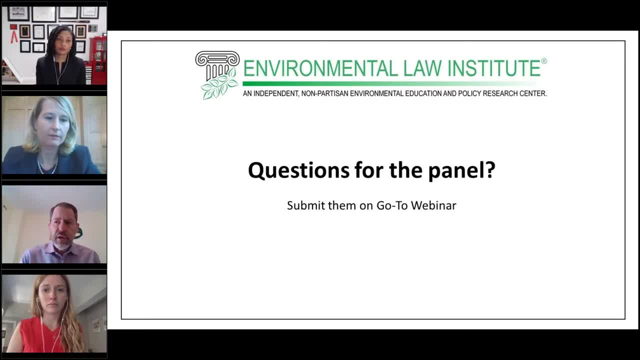 and it was coming from tailpots emissions. So they were looking at pollutants from that point of view. what were things that were hazardous, but the concentrations were not changing so dramatically over relatively small areas. Thank you, So I think we have one more question. 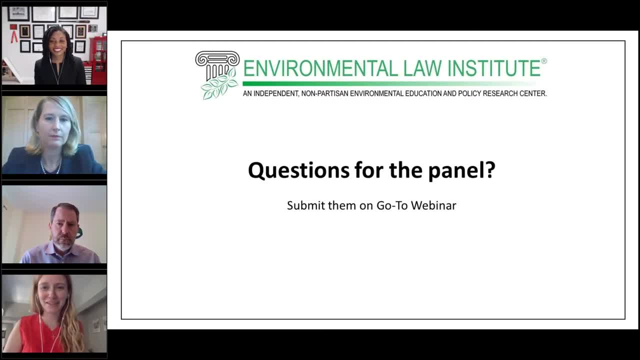 And if there's any others, please all feel free to send them in using the question box. But one of our participants asks especially in reference to the proportion of the air to the perpetual nationwide non-attainment query that you talked about just a second ago. 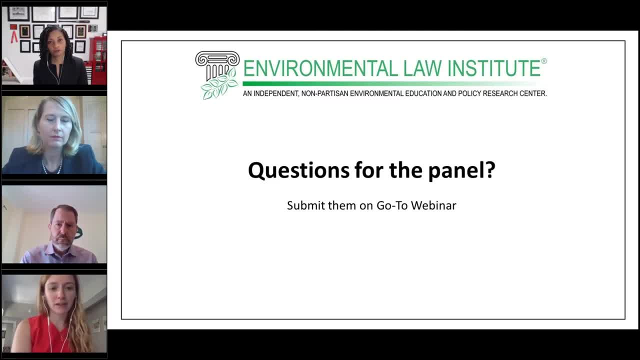 The participant asks: what do you all think about the possibility of a secondary NAX for greenhouse gases with a long range attainment date, For example with the use of section 179B, but for international emissions and unclassifiable statutes? could that help fix this perpetual nationwide? 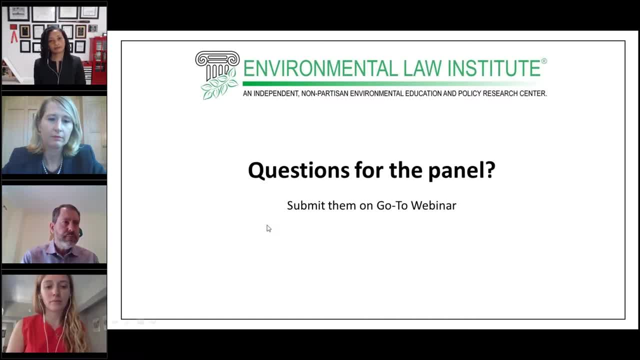 non-attainment. Well, let me say I mean it's possible, I mean anything, any framework that would get reductions would be helpful. but I just think it's a very you're if you're really going to solve the problem. 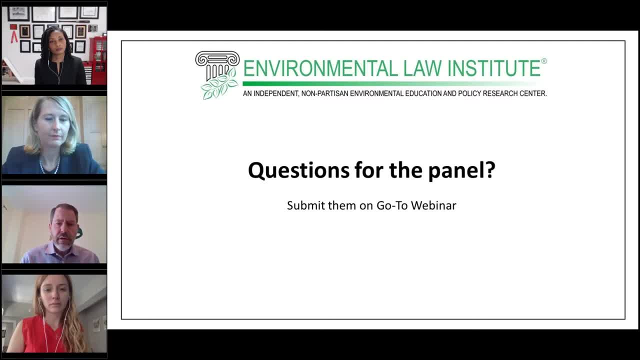 you want a solution that has as little cost as possible to actually running the system. that's fixing the problem. And I mean like for me, just personally- and this is not me as someone who works at EPA, but just me as a private citizen- 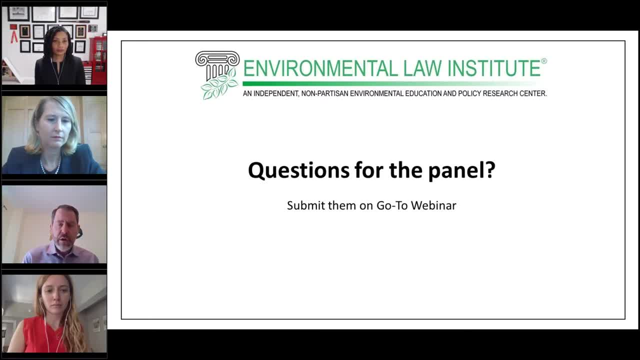 I am a strong supporter of carbon taxes because you the infrastructure is very simple to do. We already have a tax system, We have a sales tax system, So it's relatively straightforward, And then you're not having a lot of individual people making decisions. 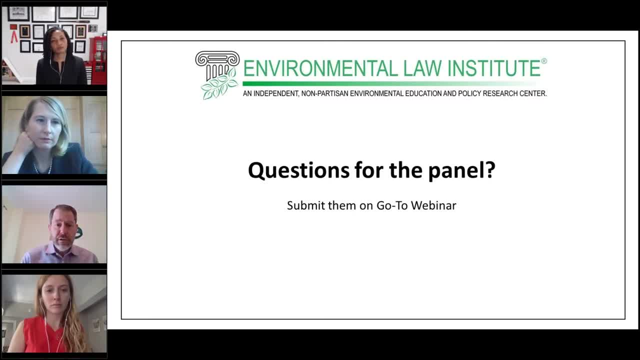 about what kind of government action is going to be taken. Individual businesses and individuals can make decisions for themselves, and you're encouraging all kinds of technology development. Whatever estimates you have for the benefits of a climate change program, if it's significant and broad-based, your costs just in the same way. 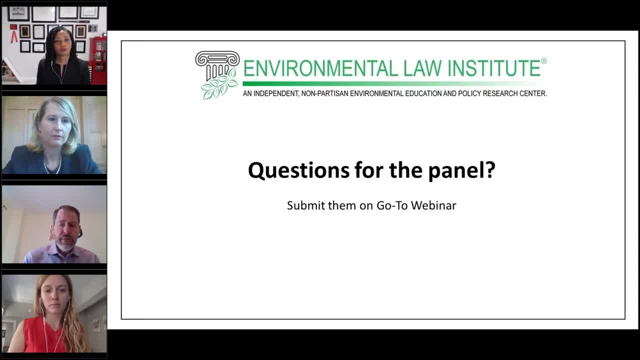 with the EFSA grant are going to be much cheaper, because one of the things that you can predict is technology development And typically when we set a standard, we may assume some slight increases of efficiency over time when we're figuring out costs. 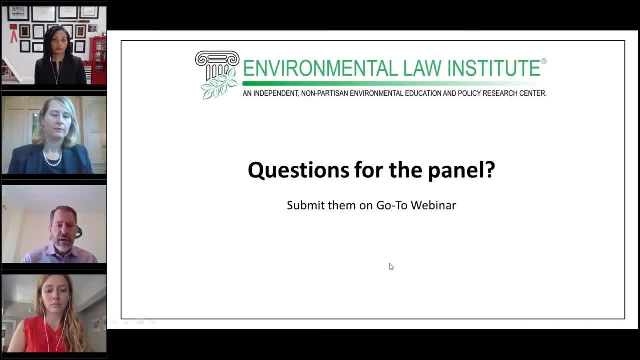 In something as big as the climate. if you have a tax on things, then you're going to get a huge economic incentive for lots of breakthroughs in technology. You'll never be able to figure out where they are If you do a system where you have like a cap and trade. 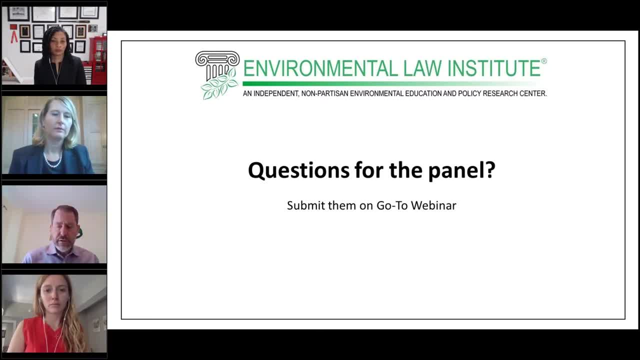 or specific regulations. they if you have a cap and trade system. so then, just for one example, if you come up with some brand-new technology in 10 years, that means that cars have zero pollution Like you, just like a catalytic converter-y thing. 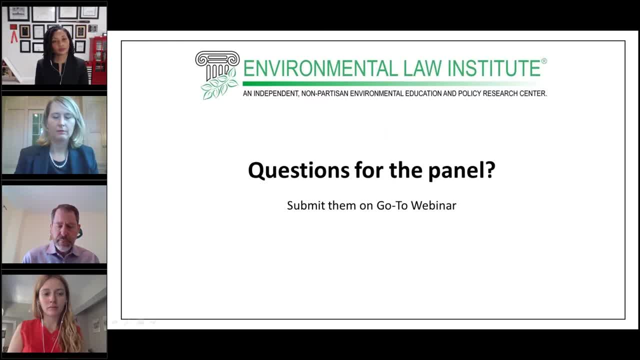 you just put on a car and there's no carbon dioxide coming out of it, Then what happens is you have a series of standards based on a cap and trade system. then all of the allowances that would have come from the automobiles are going to go. 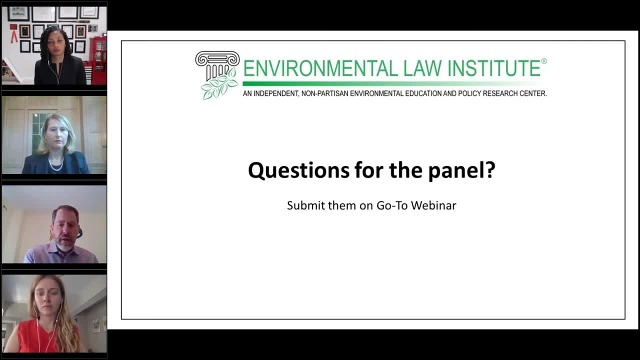 into, say, pharmaceutical manufacturing, and they won't do the reductions. but or if you have a whole set of standards around it, it's not going to make change. It'll make, it's just you're going to have, you won't. 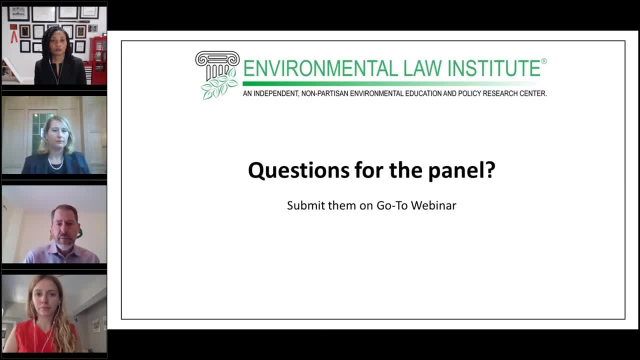 you won't be pushing that kind of technology because your standards are going to be based on current technology. But if you have a tax, then every facility or industry broadly is on their own and reductions in one place, don't you know? it's not going to change. 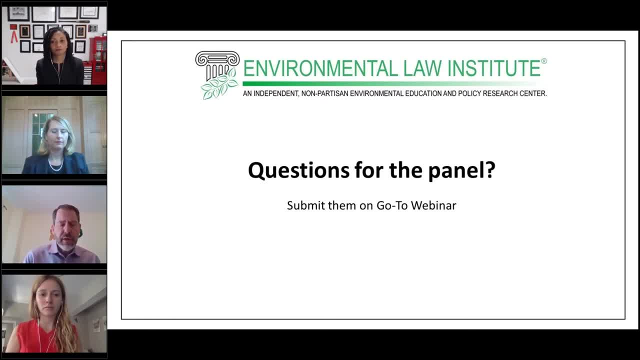 It's going to be based on the same thing. So you know, if you have a tax, then you're going to have a tax on one place. Don't cause reductions elsewhere, Because one of the things you have with a cap is you have a ceiling. 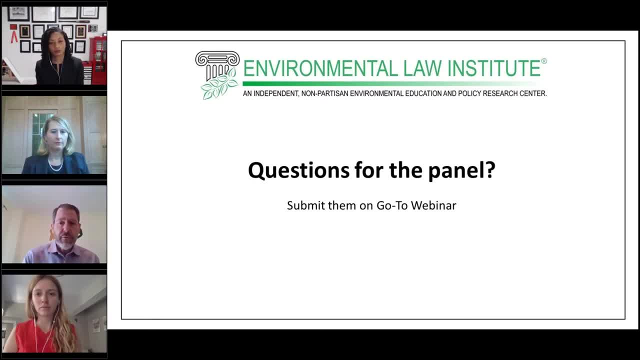 on emissions. but every man's ceiling is another man's floor. You also have a floor on emissions. You have a tax. you can get much lower emissions over time because there isn't trading between the areas where you have huge technological breakthroughs with other areas. 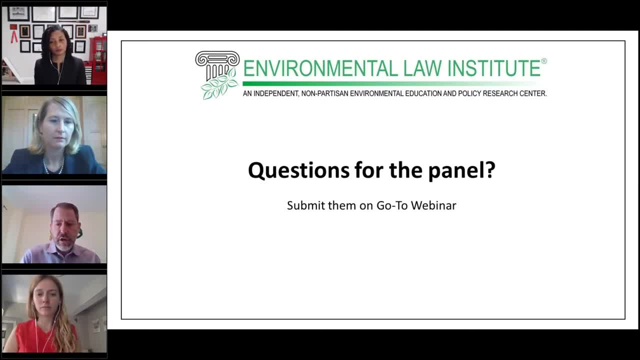 Everybody's kind of on their own. so you'll get the most reduction. You'll have the least transaction costs. You'll have the least. you know the least you know government regulatory transaction costs of setting up systems and all kinds of things. 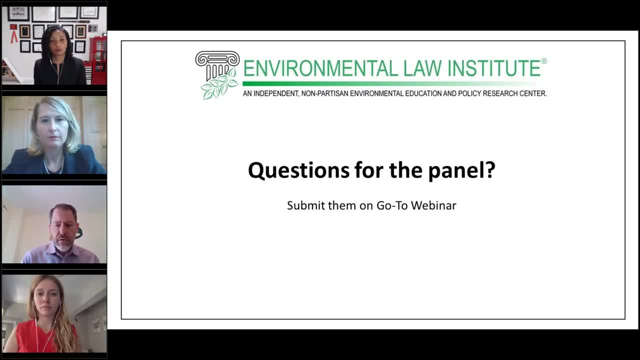 because you have a relatively simple system And you get you force and get the maximum benefit for technology. So sure, maybe you could do some kind of SIP thing, but it would just be so much more sand in the gears and inefficiencies in the system. 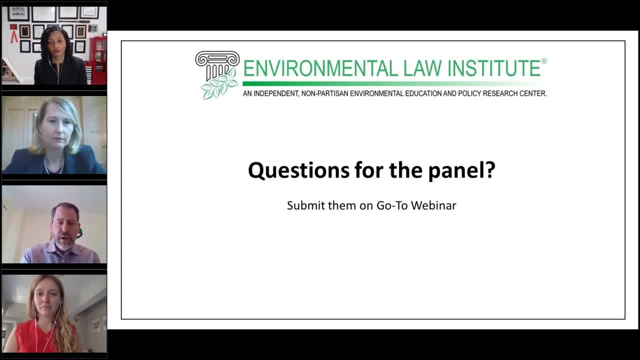 It wouldn't really. if you want to fix it, that's not going to happen. That's not the way to do it. Thank you so much. We have another question that perhaps you or Stacy could take, which is if one of you could give a description. 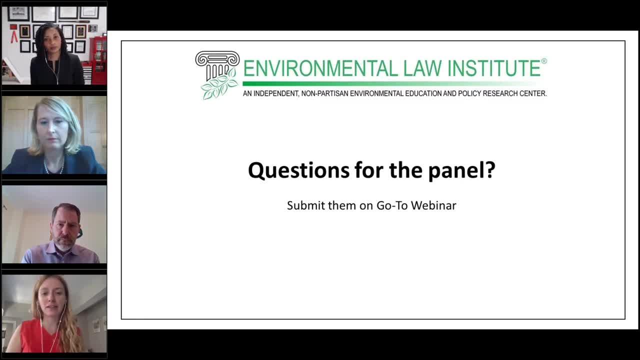 of the relative differences between the MACT and the BACT. Do you want to go Stacy? Well, I'll start, but I'm sure, since you're an expert, you should also weigh in. So the MACT standard which applies to the NESHAPs. 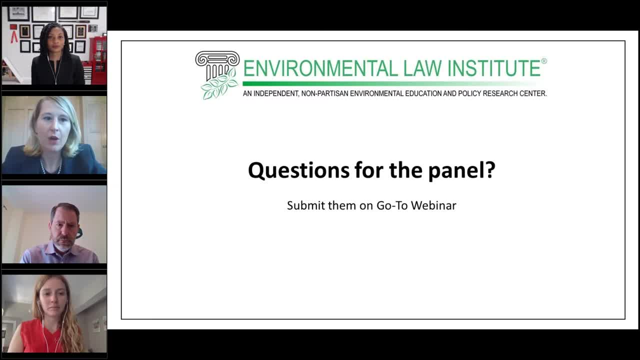 again is sort of a standard that's universal to all the sources that are going to be regulated under that program And it's the maximum achievable control technology. I think Larry had a slide that it's top 12% in terms of control technologies available as used to set the MACT standard. 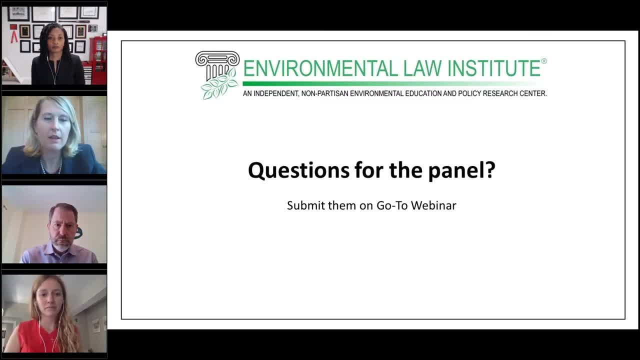 And you can, I believe, consider cost in that. In contrast, the best available control technology is something that's used under the PSD program for pre-construction permits for facilities that are deemed to be a major source there, And that is usually there's clearinghouses and stuff. 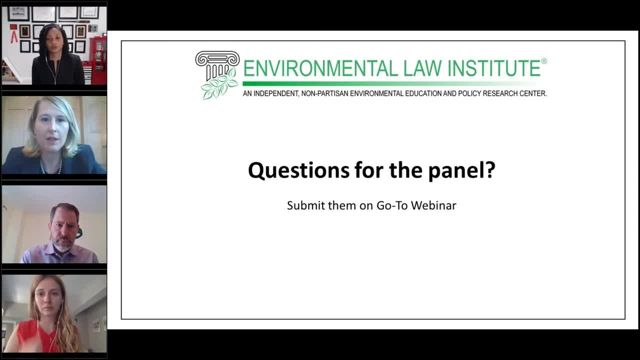 where states can look to determine what constitutes the best available technology at that time and for the particular type of operation you're looking at. So there The concepts are different. programs, in that you know, MACTs go with the NESHAPs and 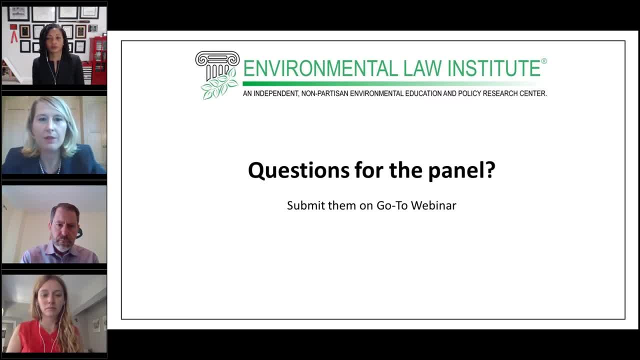 MACT goes with pre-construction permitting, but they also are set differently, with MACT being a little bit more customized based on you know the time and what you're doing, the permitting. So, Larry, I don't know if you have any further context. 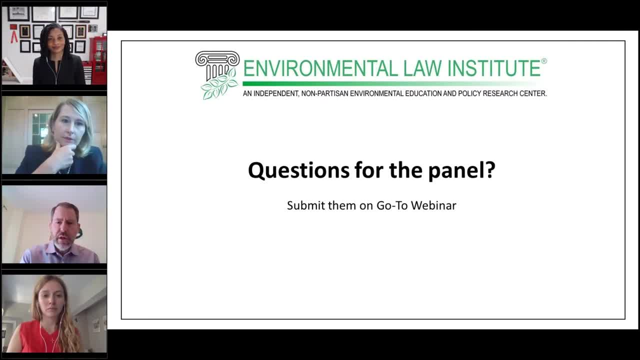 to add there: Yeah, no, I think it's fine. I think people shouldn't get caught up in the acronyms and try to balance. well, is maximum better than best or is best better than You know? they're not set that way. 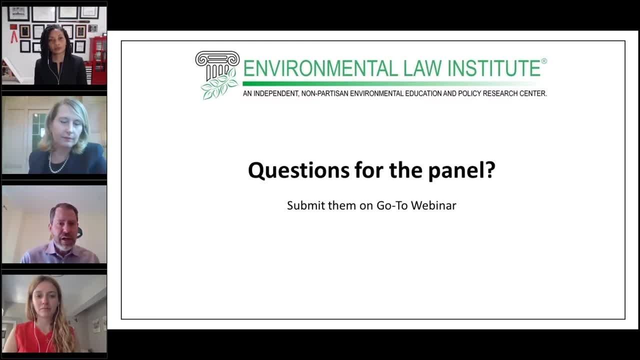 It was just: people are looking for terms and they're taking them and they shouldn't really be compared that directly between each other. So you shouldn't. If that's confusing, you just ignore that totally. It's just not really. Don't worry what the acronym stands for. 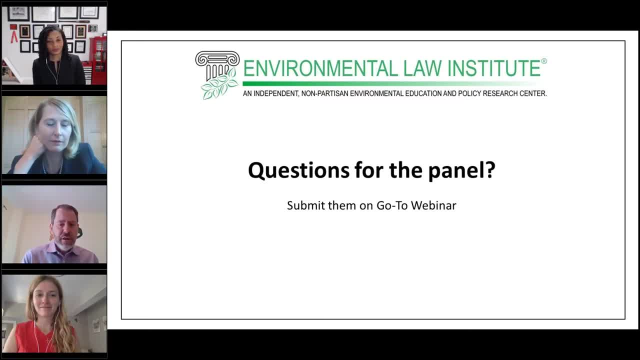 States they got. you know, the MAC standards are general, They're broad-based, They're They're not cost-based. MAC standards are individual to facilities and are very dependent on cost and very dependent on very specific situations. And, don't worry, the difference between maximum and best. 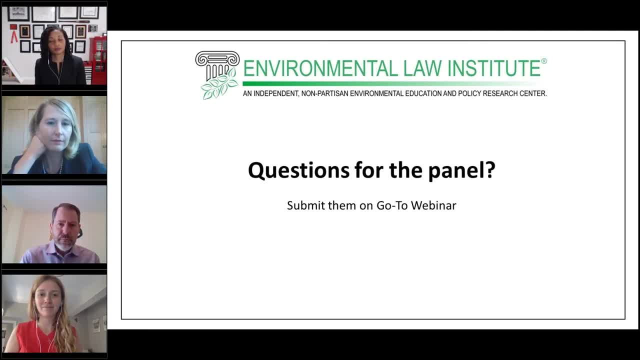 is not relevant. Thank you both, so much. So, Natasha, we have a comment and question for you. One of the participants writes: thank you for reminding us about the health implications of climate change. I know that this is relative, but what do you see as kind of the most pressing health issue? 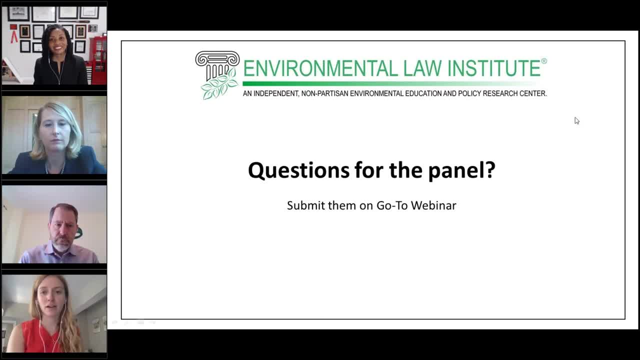 coming out of the implications with climate change right now? Oh, that's such a tough question And I'm going to give a non-conventional answer. I think it is the inequities that climate contributes to. It furthers health disparities. 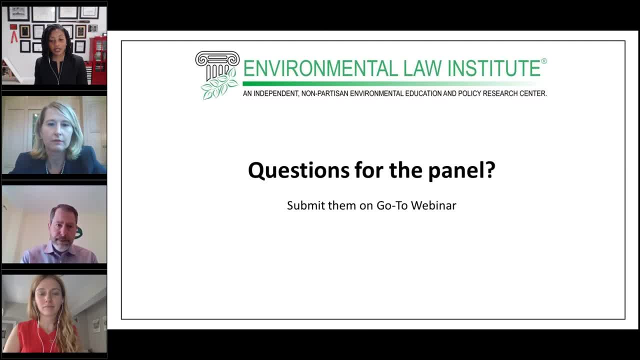 It furthers health disparities, in particular, among our most vulnerable populations, And so I think that it, being a great threat multiplier, is one of the greatest threats that we're experiencing in climate change. So, as I said, we're all at risk. Thank you so much. 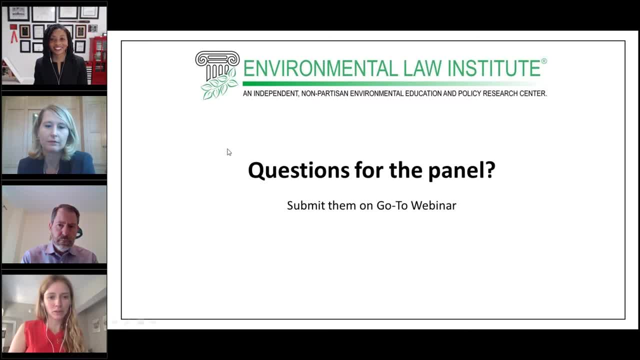 And then I think we have one more technical question before we wrap up. Can someone please explain what is being done for the retirement of existing sources of pollutants? They gave an example of older cars. So is EPA regulating older sources that continue to pollute under the Clean Air Act? 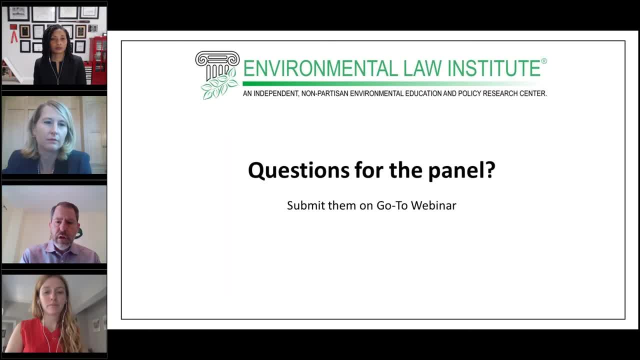 So for older cars it depends on your local area. Certainly we test cars. We test cars while they're in operation as well over time. So that's where you get recalls for pollution control systems that aren't working. I'm sure many people have gotten recalls. 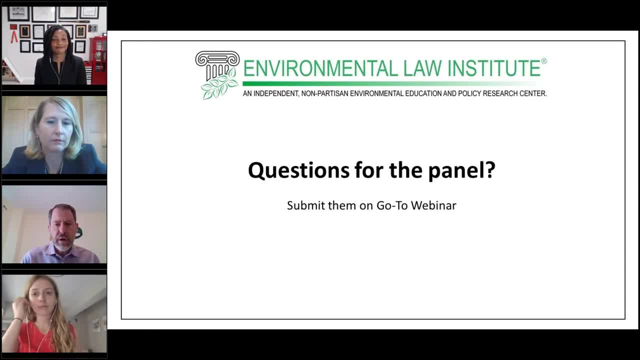 of their cars over their, you know, at least once or twice in their lives. So we do keep testing. There is some ongoing testing of vehicles over time. In addition, in certain areas, depending on your air quality, there are inspection and maintenance programs. 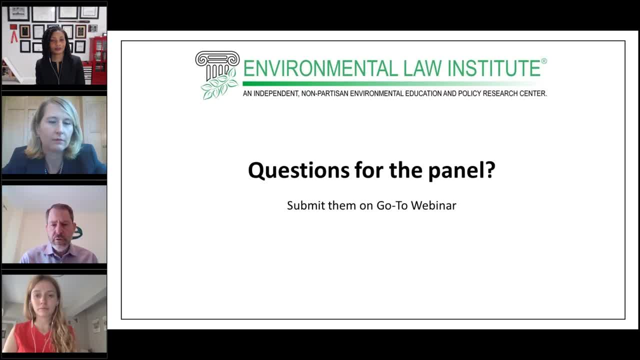 Which, like where I live in Virginia, Northern Virginia, in the DC area, every two years I have to bring my car in and have a submission system tested as part of the registration process. So if I don't get it tested, 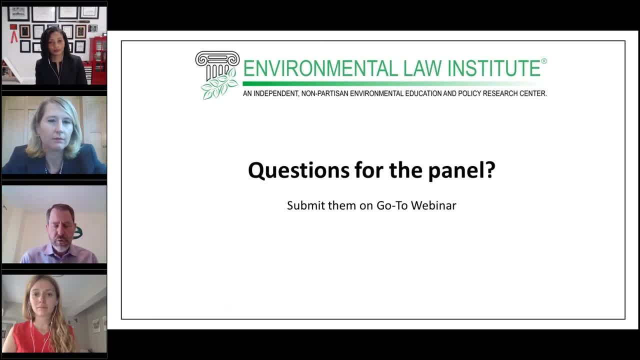 I can't re-up my registration, which then would lead to tickets, So I have a decent incentive to do that, And so people will actually you go to the garage and while they're testing the general safety, like are the brake lights working? 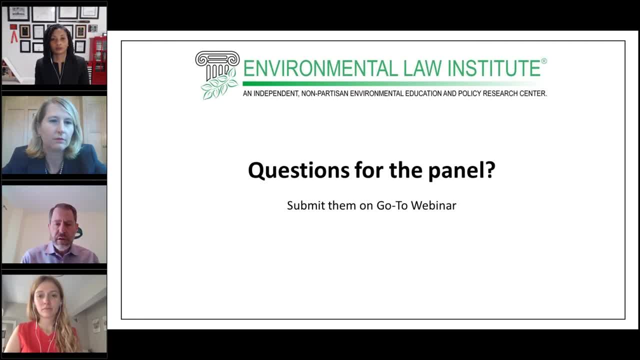 are the brakes functional? they also will test the car emissions to make sure that the equipment's still working. But that equipment's only warrant, you know, only lasts for so long At some point. cars are older than that and there really isn't any specific control.